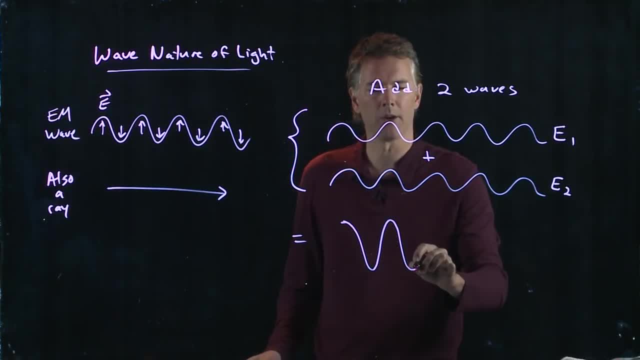 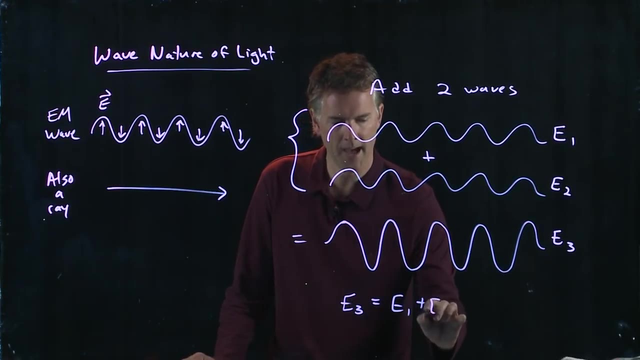 to be a low value, And then it goes back to a peak and a trough and so forth And we can see that our resultant wave is bigger than either of those two. And all you have to do is add a wave. And so what we're going to do is add up the electric fields: Electric field one plus electric field two. 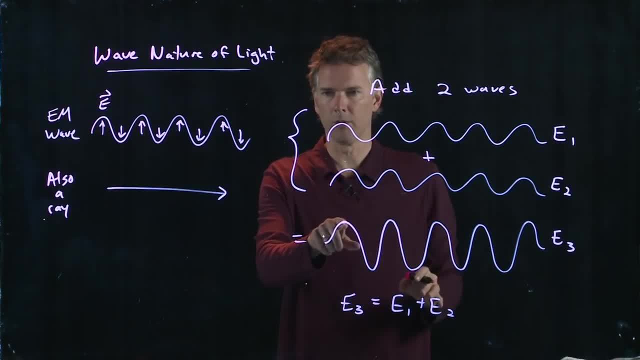 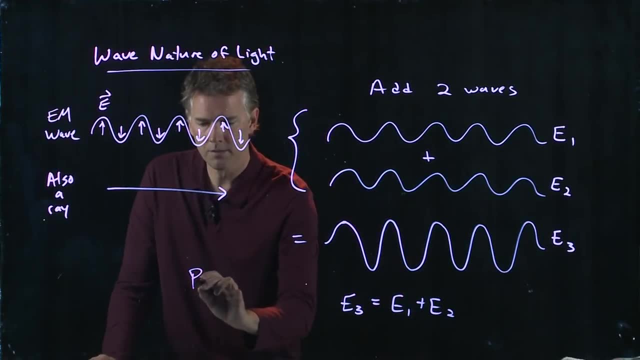 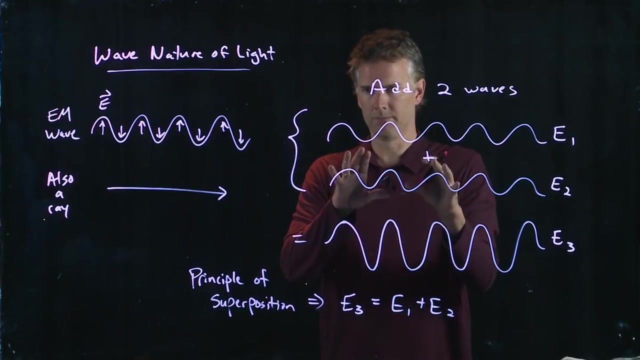 equals electric field three. So if these were the same size, then this electric field would be twice that. Okay. Now, this is because electric fields, as we know, obey the principle of superposition. So if you look at that earlier, in the case of static electric fields, right, if you have two. 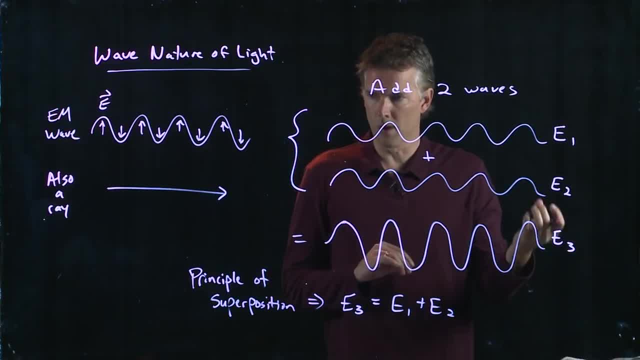 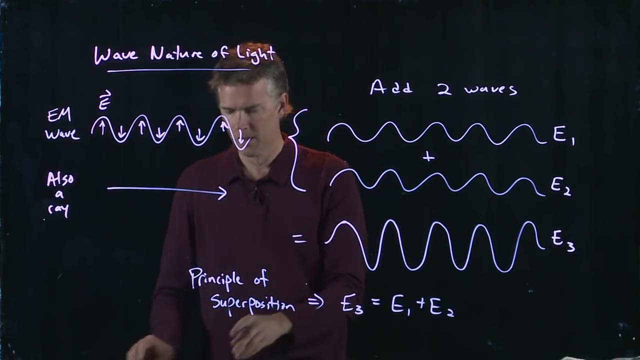 different charges and you want to calculate the electric field. you calculate the electric field due to one, the electric field due to number two, and then you just add them up. Same idea here, except these fields are now changing in time and changing in space. Okay, We're into dynamic. 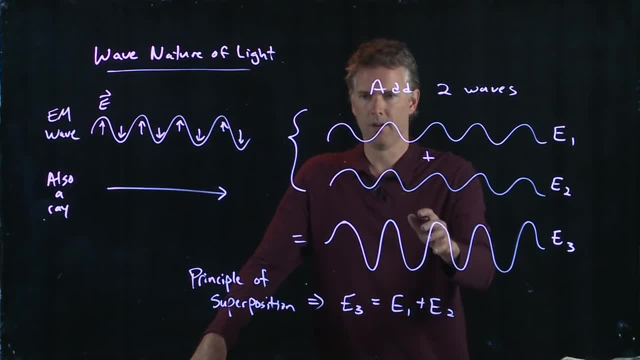 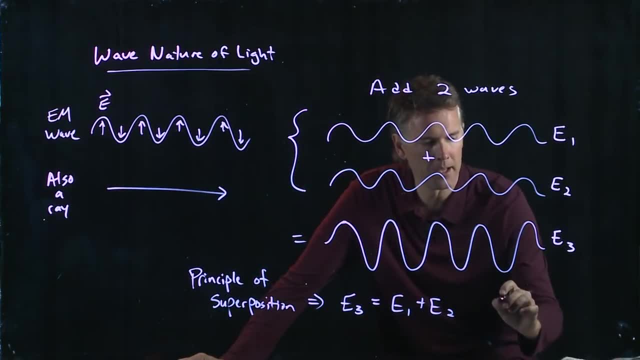 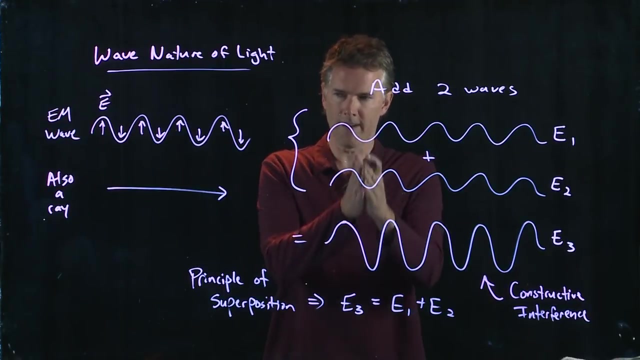 fields. So the way we added these up here, I lined up the peaks and the valleys of these waves And that led to a big wave here, And that is known as constructive interference. Okay, All the peaks lined up, all the valleys lined up, And so the 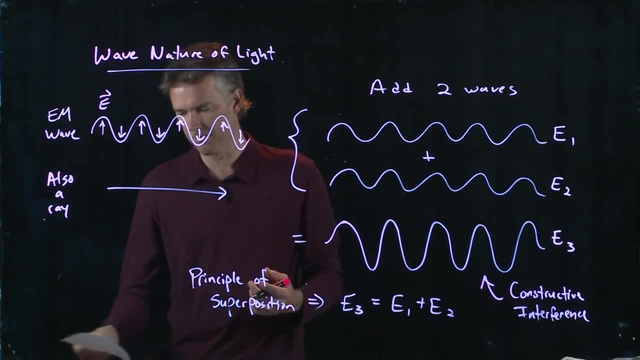 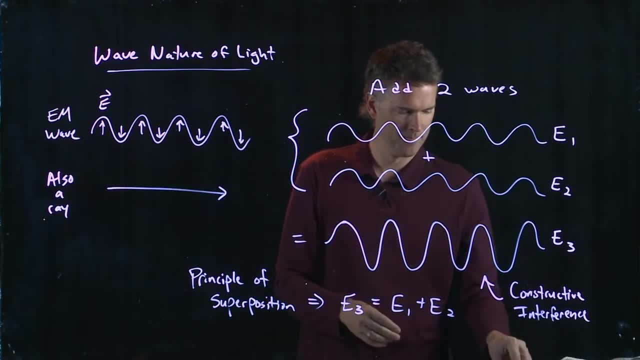 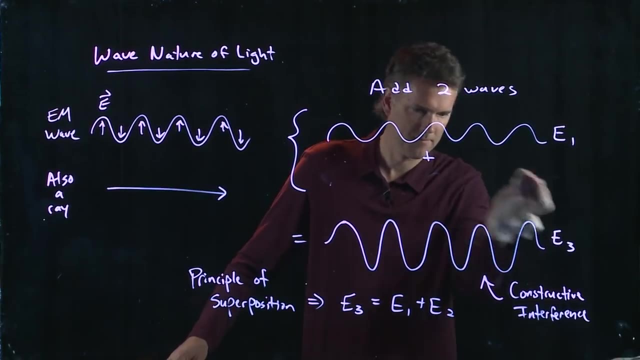 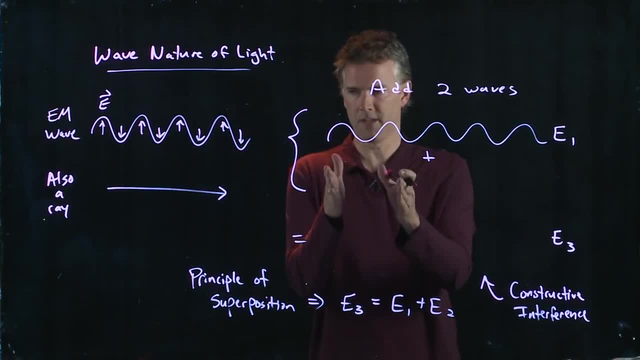 So let's make our second wave slightly shifted in time And therefore it's going to shift. so far We can make two waves and we get a very smooth kingdom cycle. Everything else is negotiable. you know that. it's the inverse of wave number 1.. 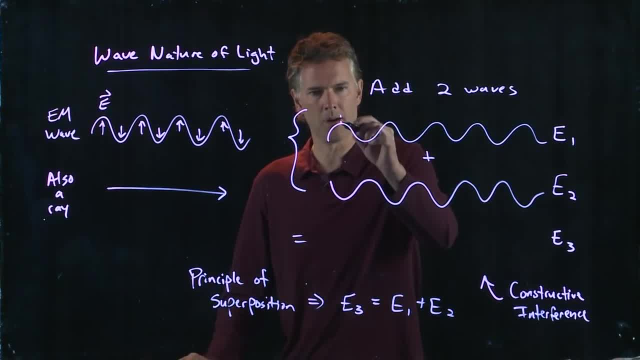 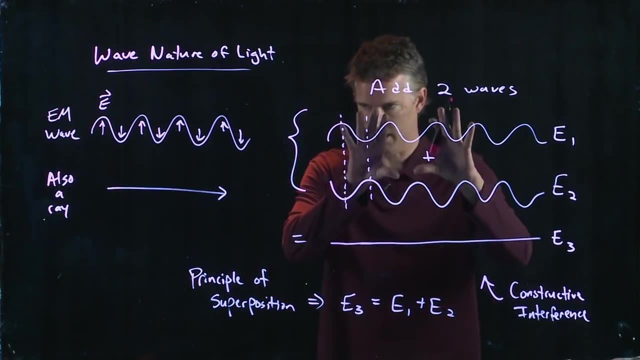 Okay, And now, when you add these things up, what do we get? Well, we add up those fields and we get something pretty flat. And we add up those and we still get something pretty flat. And in fact, if those two were exactly equal in amplitude? 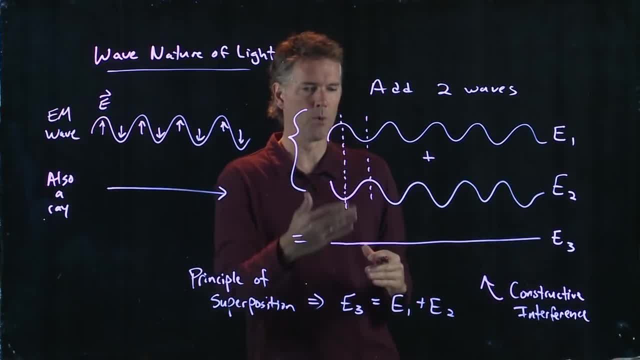 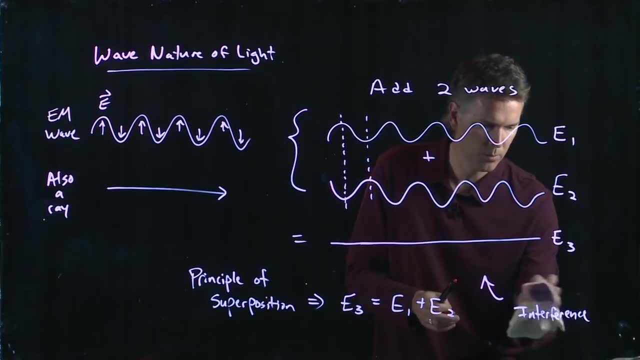 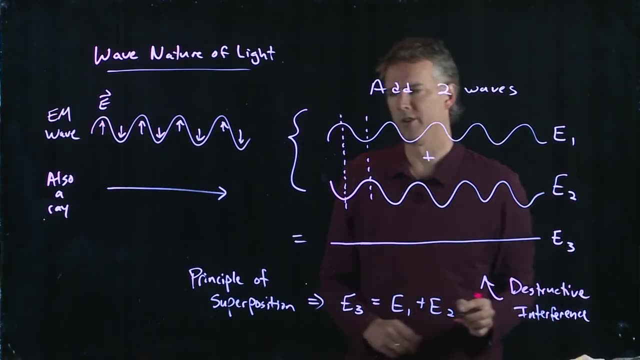 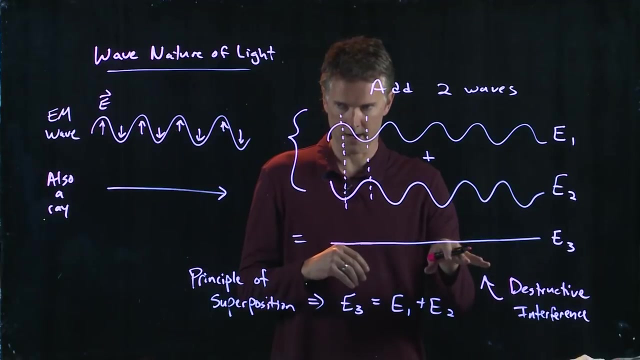 but flipped. in other words, one was the negative of the other. the resultant field would go away. E3 would be 0 and that is called destructive interference. Okay, Add one wave to its inverse, it goes away entirely. You can take that wave out of there. 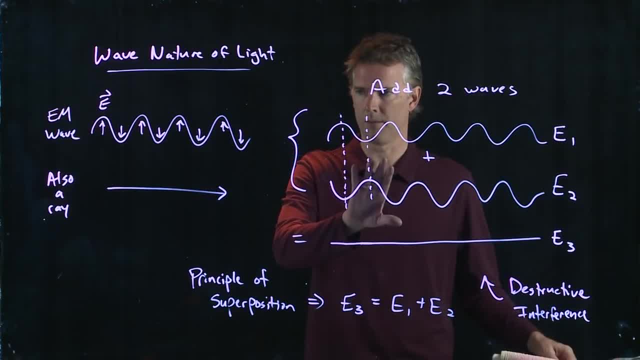 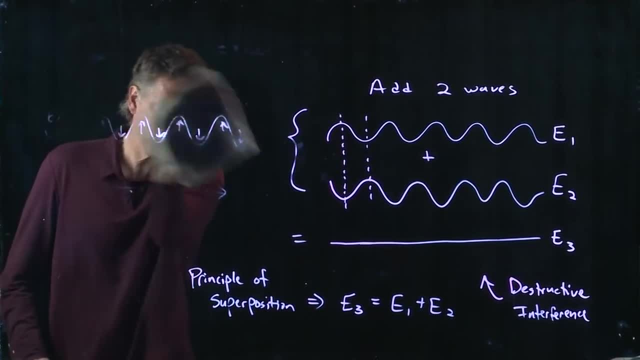 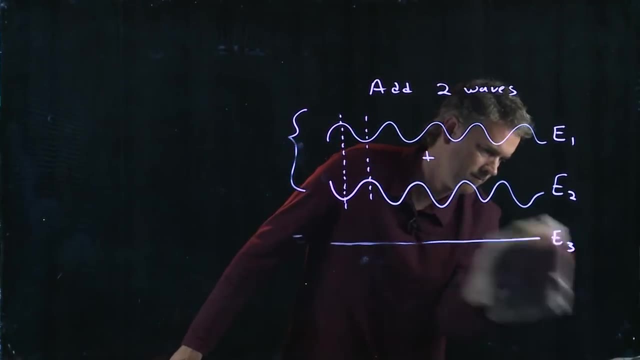 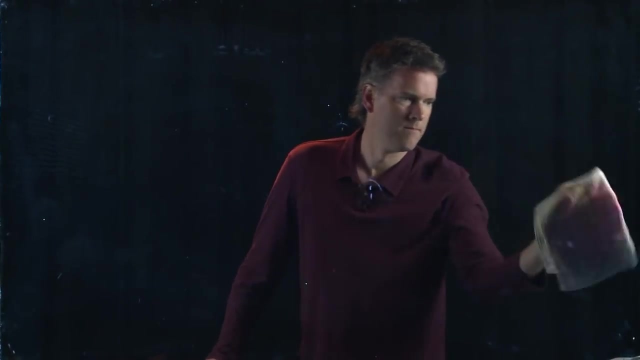 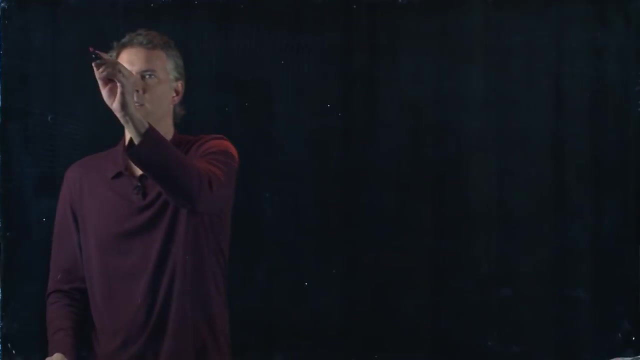 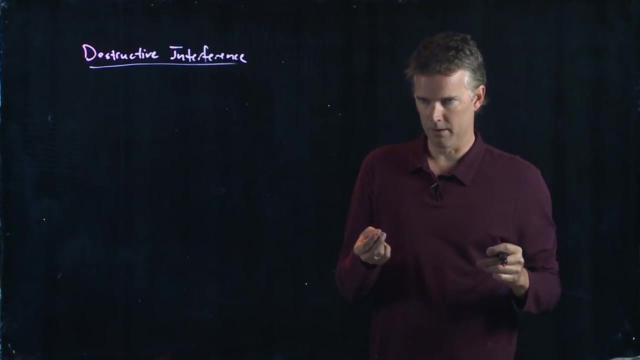 So you're actually kind of in the middle of the equation. You're kind of familiar with this concept already. Where might you be familiar with the derivative? It's called destructive interference. This is used in a very popular device that I'm 99% sure you have heard of. 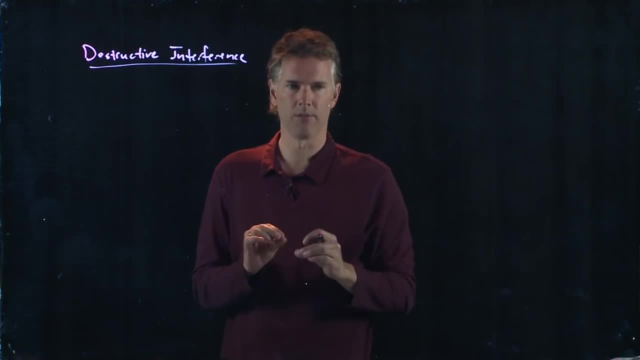 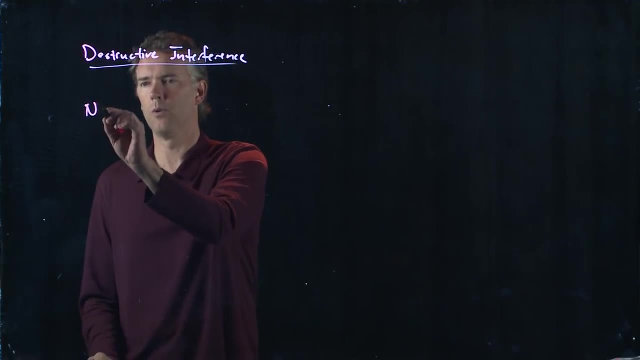 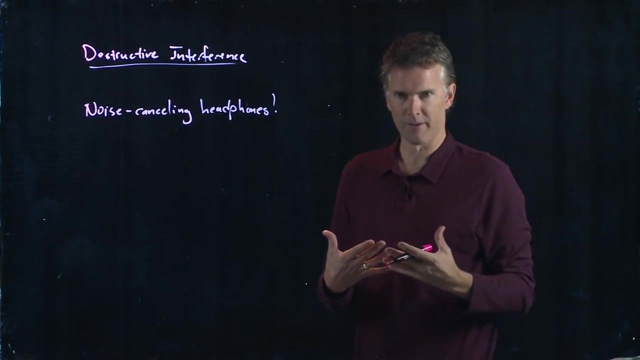 Okay, And it's not with light, but it is with sound. Anybody know what I'm talking about? talking about noise-canceling headphones. You see these on the SkyMall catalog, right When you're flying around. they're like: hey, it's really loud on the plane. 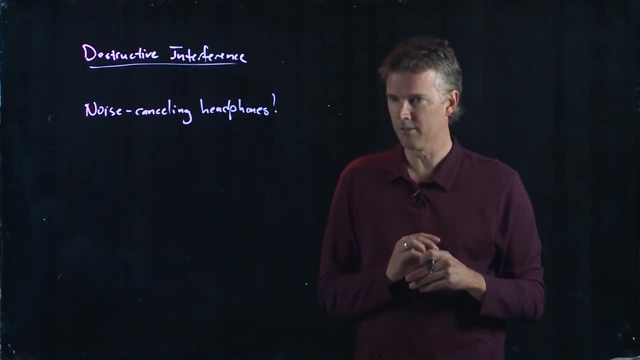 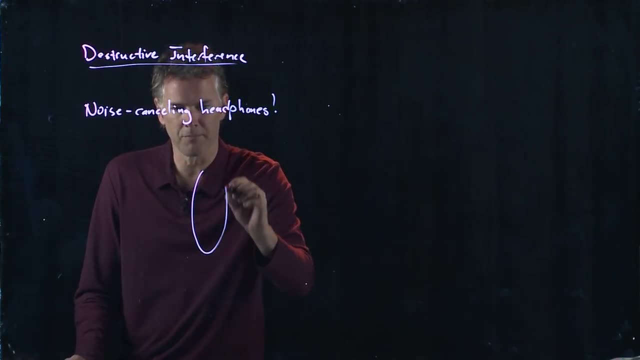 Perhaps you'd like to buy these noise-canceling headphones for $250 and cancel out all that external noise. How does it work? Well, headphone is just a speaker that's right up next to your ear. We know what a speaker consists of. 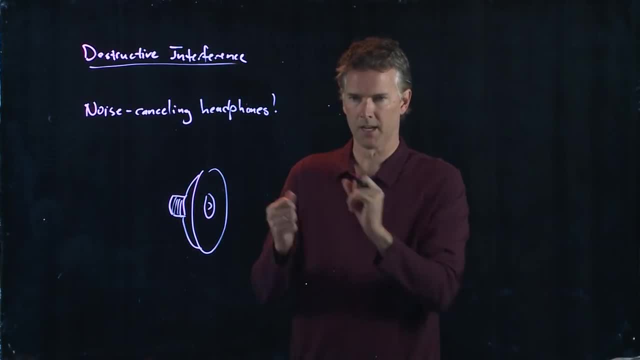 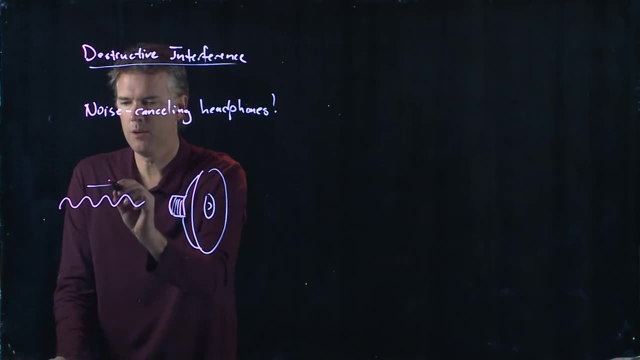 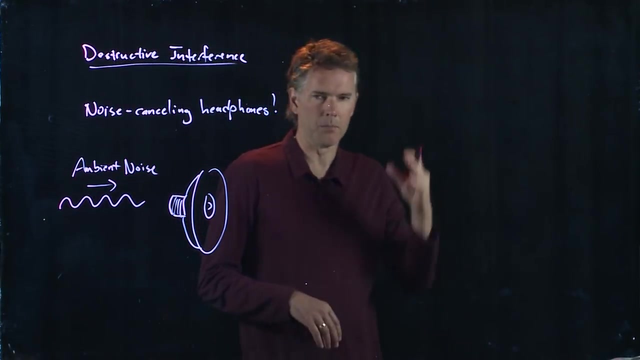 There's a coil, there's a magnet speaker goes in and out, makes a sound wave. How does a noise-canceling headphone work? Here comes some noise from the outside. That's our ambient noise. That could be the rumble of the engines of the plane. 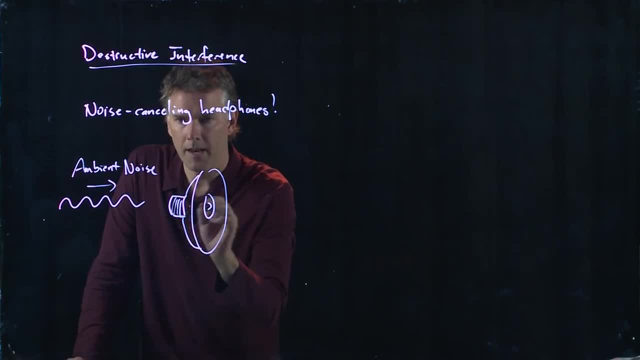 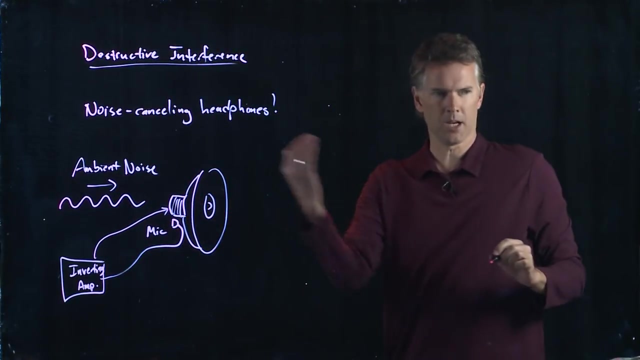 In the noise-canceling headphones. they not only have a speaker, but they have a little microphone And that mic records the ambient noise, sends it down to an amplifier which inverts it and sends it back to the speaker. So now, coming on the other side of the speaker, what do we have? 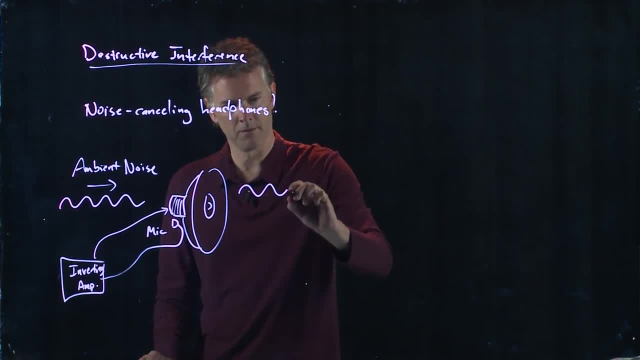 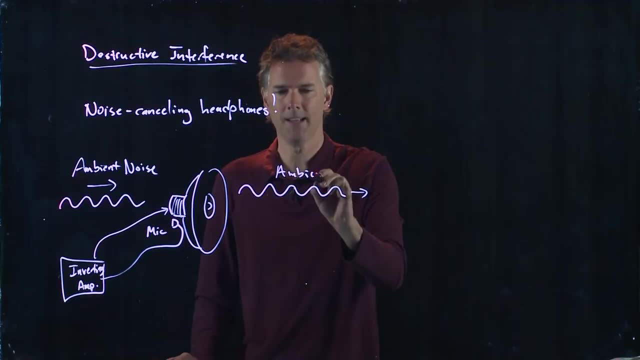 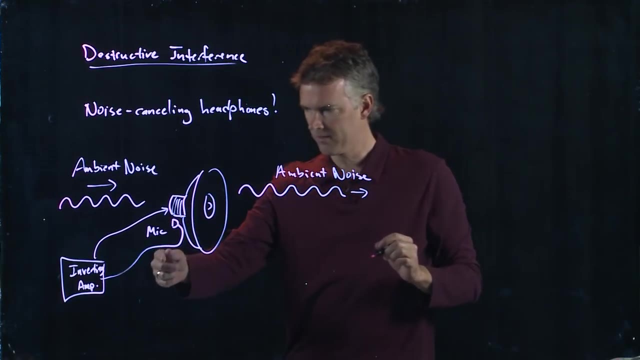 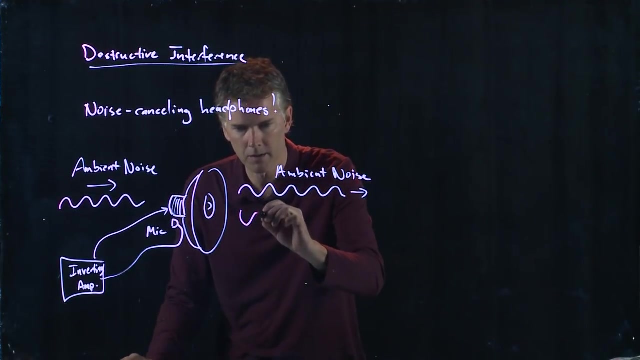 Well, you still have your ambient noise right. Ambient noise keeps coming right on through, But you're going to add something from the speaker. It recorded that sound, it inverted the signal and it sent it back to the speaker, And so the inverted signal looks like this: 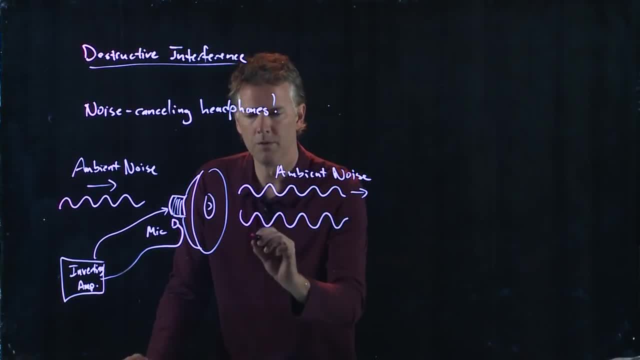 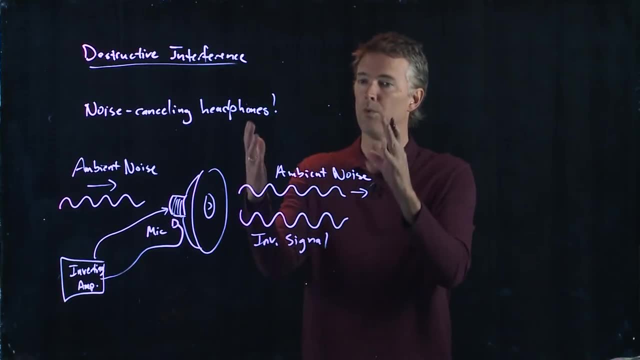 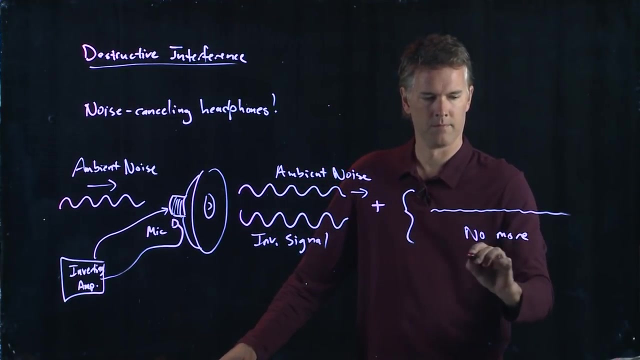 And so it's going to send it back to the speaker, which is just what we drew a second ago, And so the resultant sound wave that you hear on the other side is nearly zero. Okay, so this is a very clever little idea. 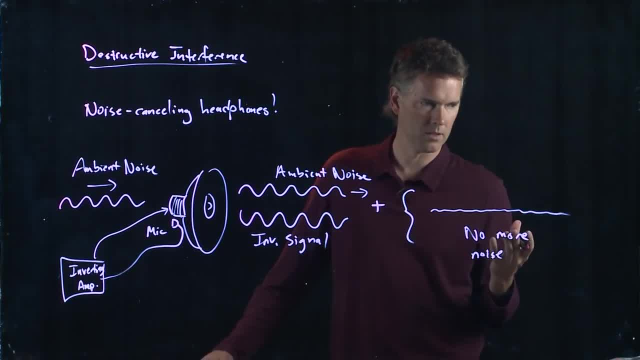 It's been around for maybe 15 or 20 years. It's been around for many years. It's been around for many years. It's been around for many years, And so if you've ever tried some of these headphones, they work really well, right. 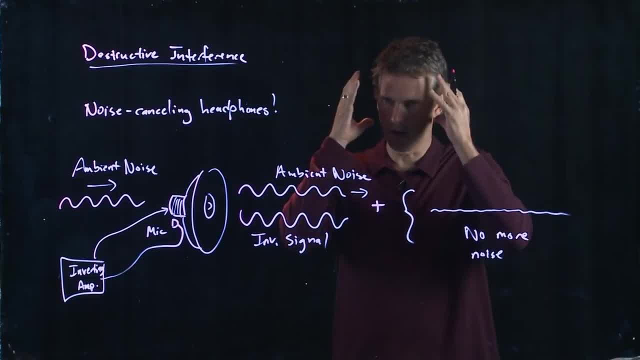 You put them on and you turn on the amplifier and all of a sudden all the room noise goes, It disappears. It's a little disconcerting actually, initially when you do it, because as humans we like a little bit of noise in our ears. 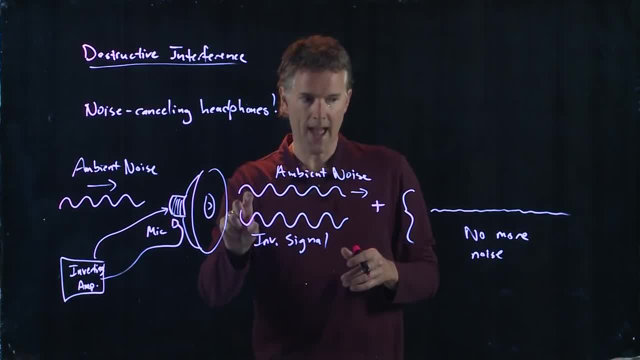 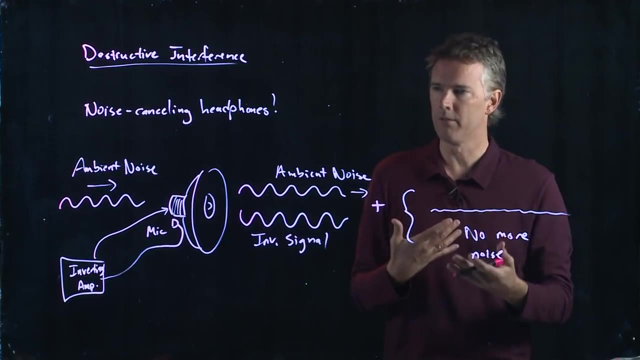 Okay, It's very good at doing this at low frequencies. Okay, Okay, Okay, easier to record the low frequency, invert it, send it back. The low frequencies are long waves, very clean signals and so, like the rumble of the jet, those noises will go. 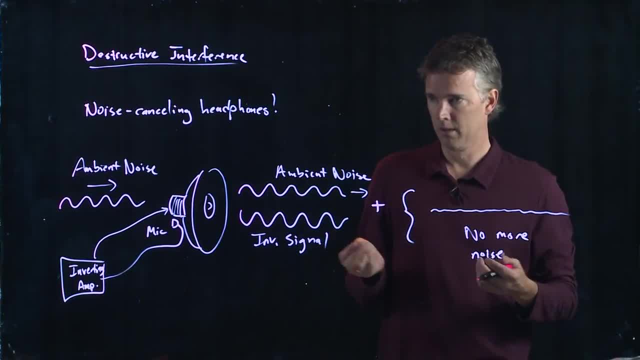 away. It's not very good at the really high frequencies, So if you have somebody next to you on the plane hitting their triangle, that's not going to get cancelled out, unfortunately. Okay, so this is the acoustic analog of this idea of destructive interference. Let's 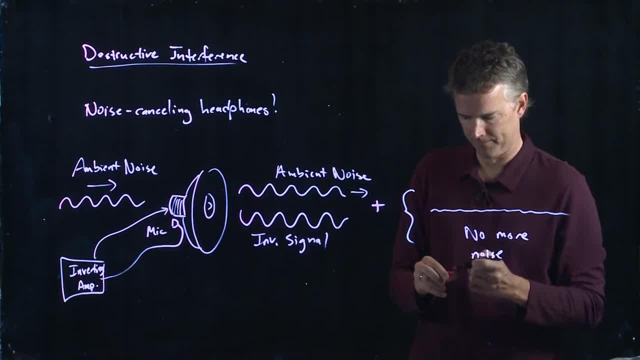 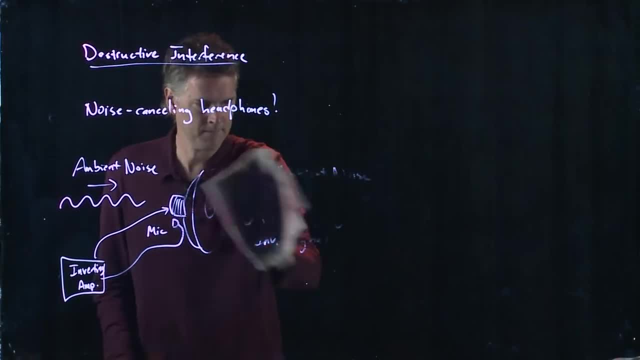 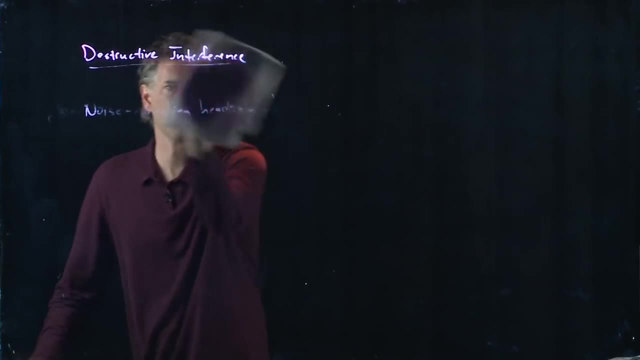 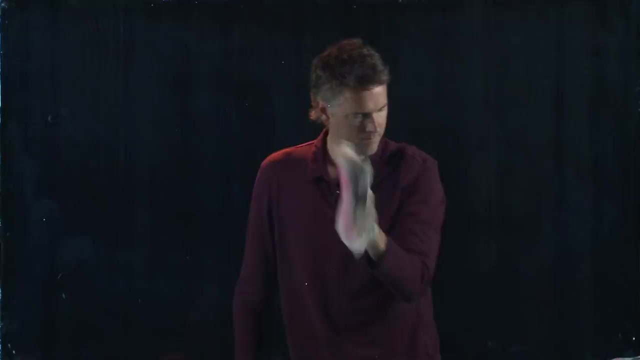 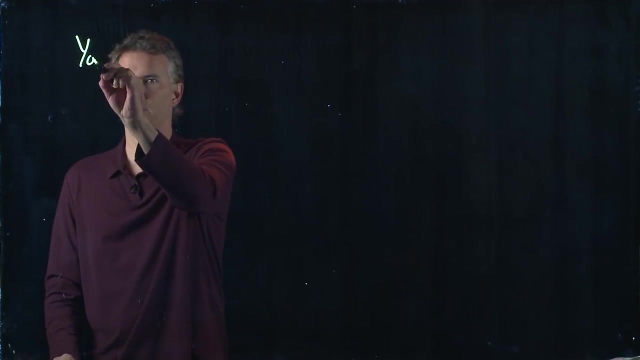 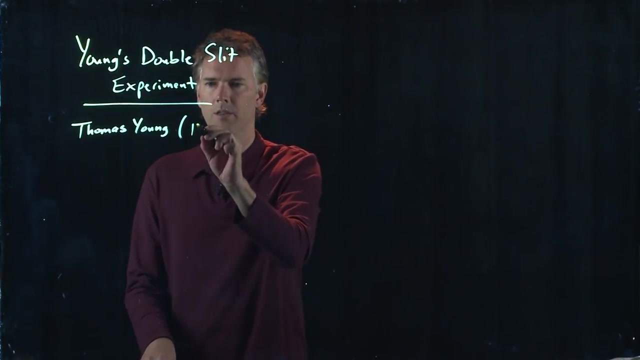 talk about the optical version of this. So the optical version was demonstrated in something called Young's Double Slit Experiment, And this was done by Thomas Young and he lived in the United States, and he lived in the United States from 1773 to 1829.. And Young's Double Slit Experiment is the following: 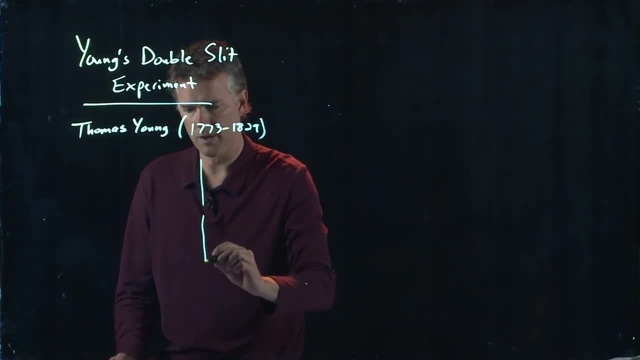 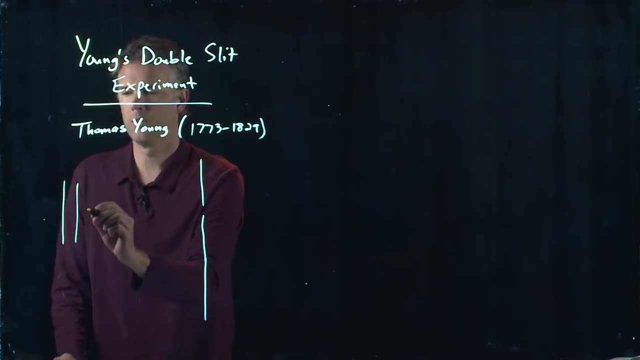 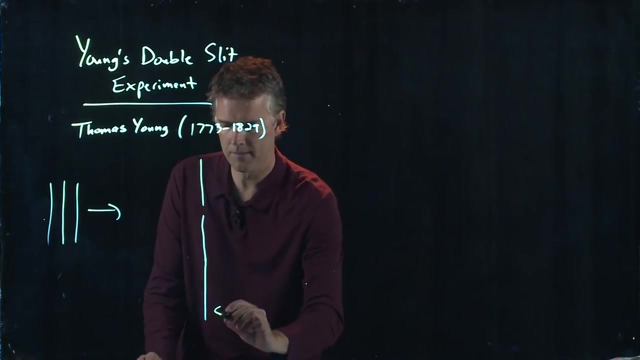 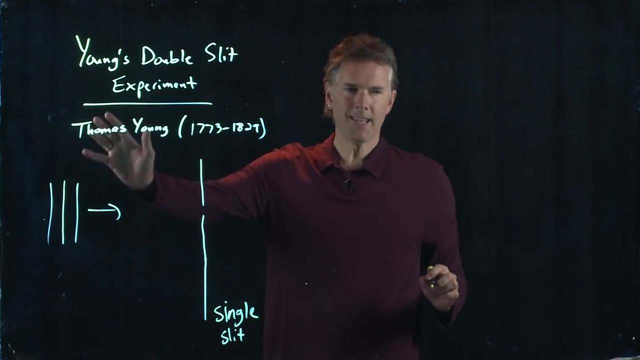 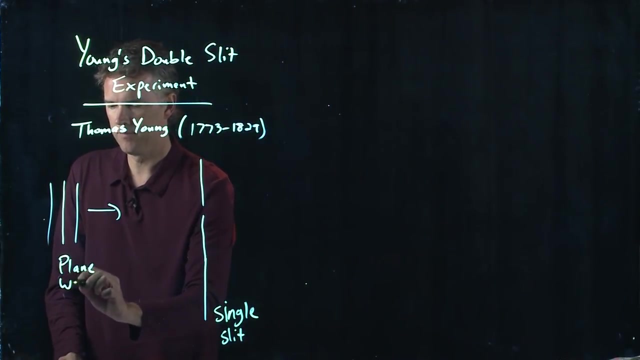 Take a card and put a hole in it. And now let's send some light towards that little hole in the card. This is a single slit. He did this using sunlight that he filtered appropriately, so it behaved like a plane wave, And when you send it through this single slit, what happens is the light spreads out. 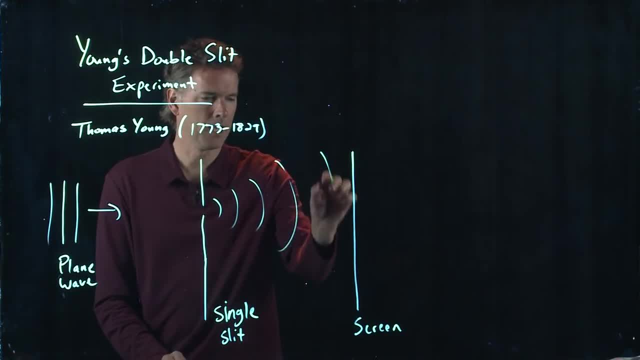 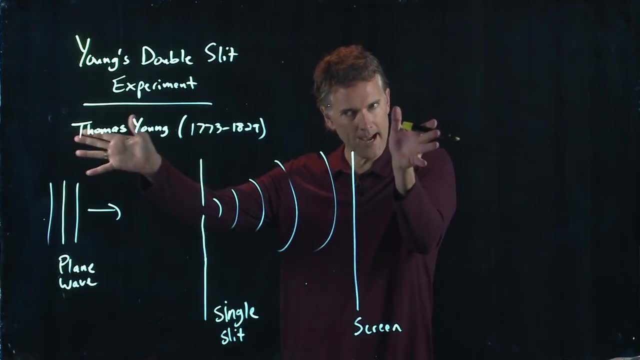 And it starts to spread out and it covers the entire screen with sunlight. So a light comes through this little pinhole, spreads the light out, it covers the entire screen, Okay, and so the whole screen gets illuminated. Now that in itself is kind of cool, right? It tells us a little bit about diffraction. 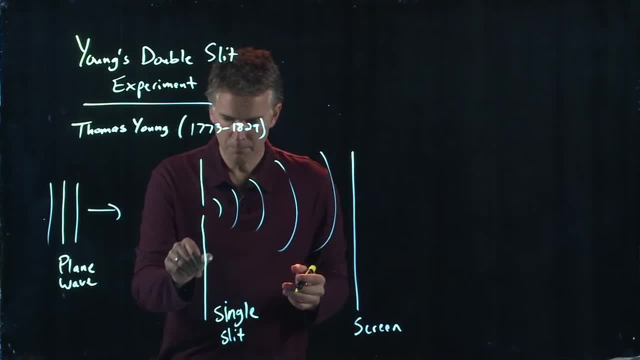 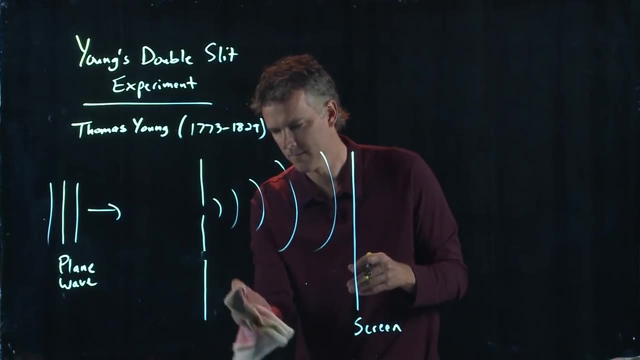 from this thing. But the important point is, he put a second hole in this screen, in this screen right here, And so now it's not a single slit anymore, it's a double slit. Now, that's not a single slit, It's a single slit. 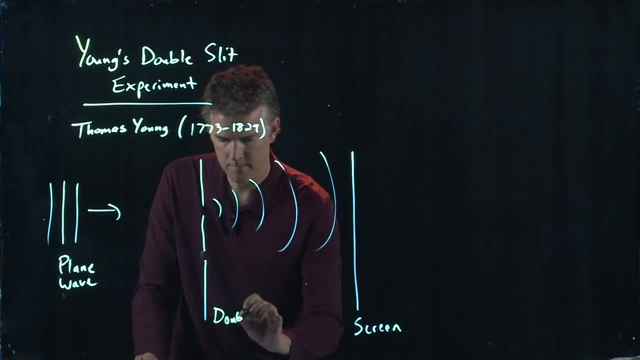 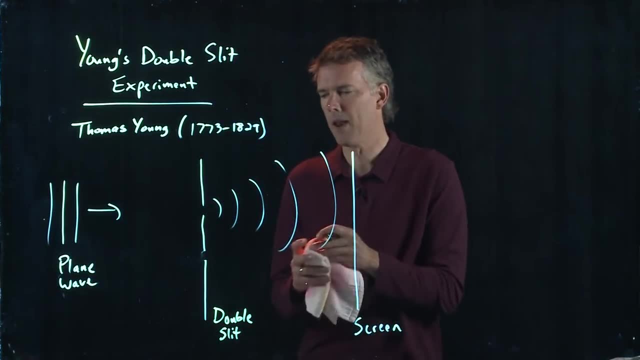 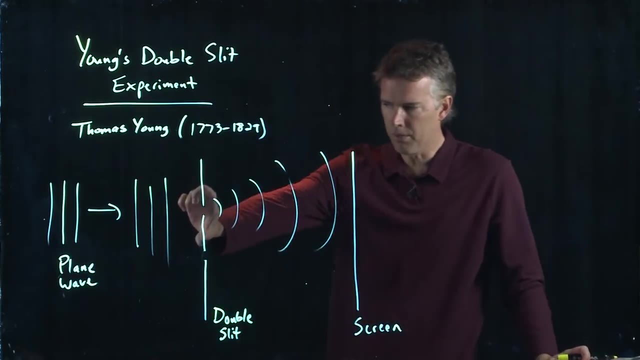 And here's what's going to happen. Now you might think: wait a minute, we've just let more light in, right, This plane wave that's coming in, which occupies both of those holes that light's going to go through. 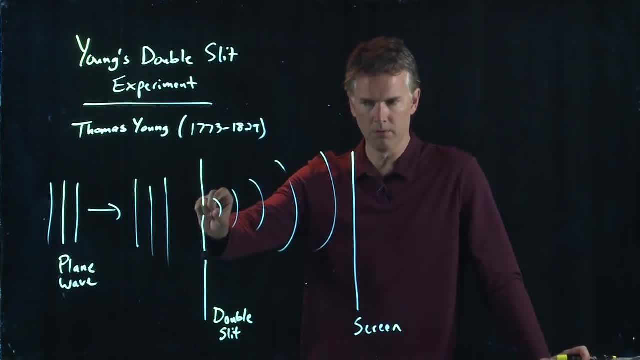 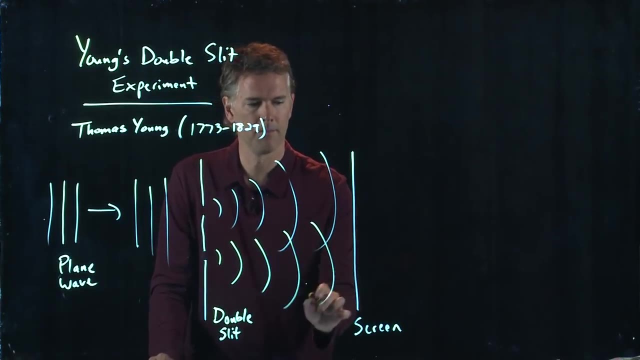 This one's going to spread out. This one's going to spread out. My entire screen is going to be a single slit to spread out. my entire screen should just get brighter, okay. And yet something very different happened When this one spread out and hit the screen. there were regions on the screen that certainly 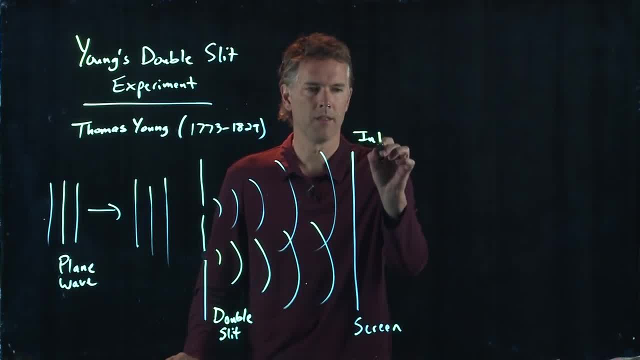 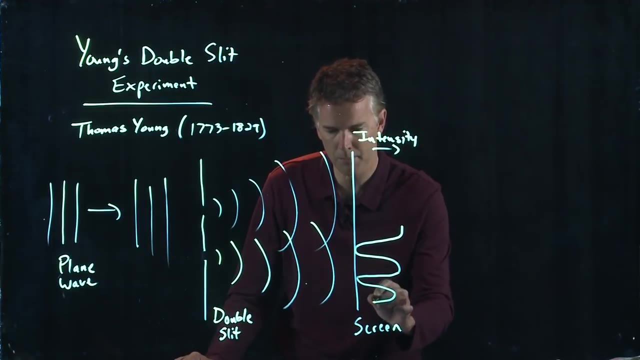 got a lot brighter And if we think about the intensity, the intensity in the center was very bright, but then something really weird happened: It went to zero and then it got bright, and then it went to zero and then it got bright. 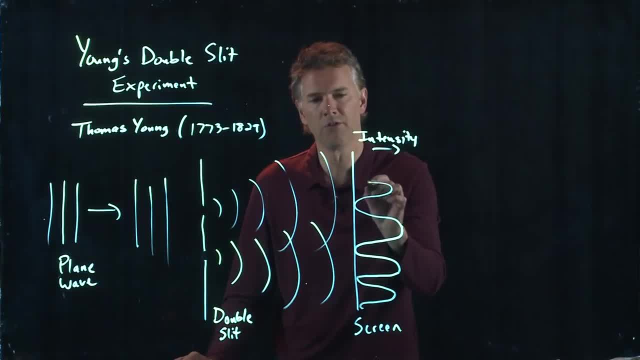 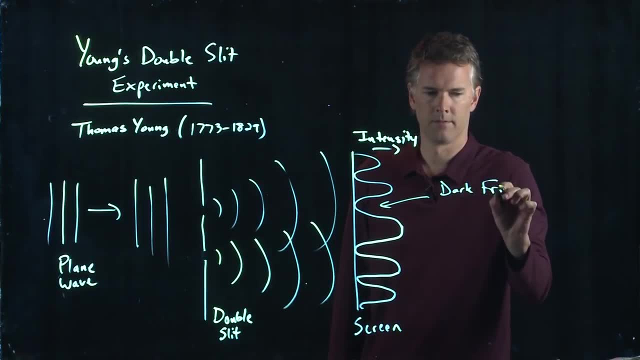 and then it went to zero And there were these dark fringes that developed. There were these bright regions which people expected. right, We've added more light. There must be more light over here. So if I take a picture of this thing, I must have some bright regions. 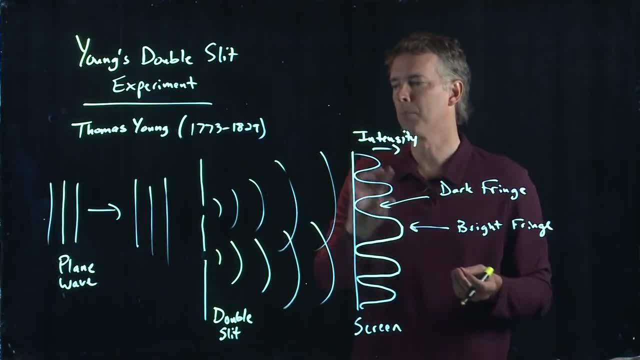 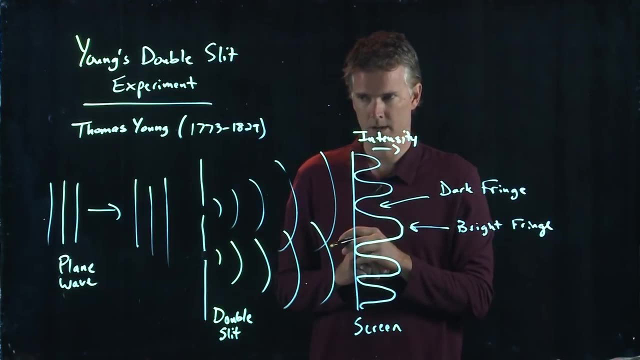 You absolutely do. You have some bright regions, and those regions are certainly brighter than with just one hole. But there are these regions where it is completely dark. It's not like just kind of dim. there The light intensity goes to zero at that point. 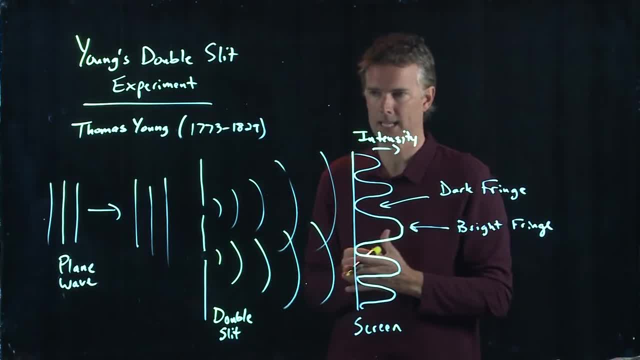 And this really confused people. okay, back in the late 1800s, right. So thinking about this experiment, they were saying you just added more light and somehow you got the light to go away entirely. And it's kind of like those noise-canceling headphones that we just talked about. 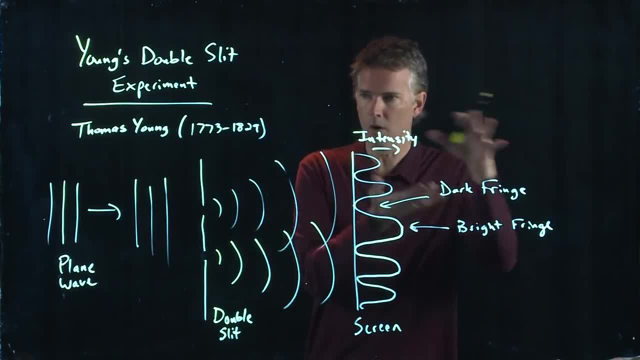 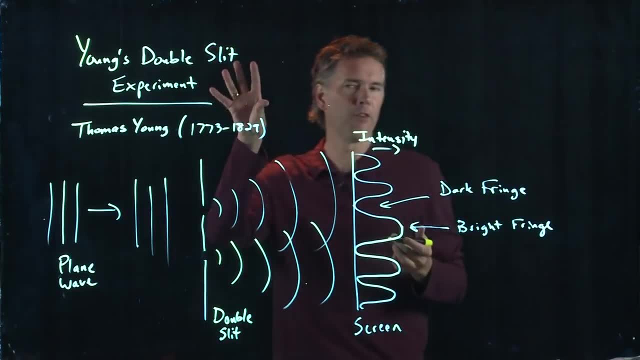 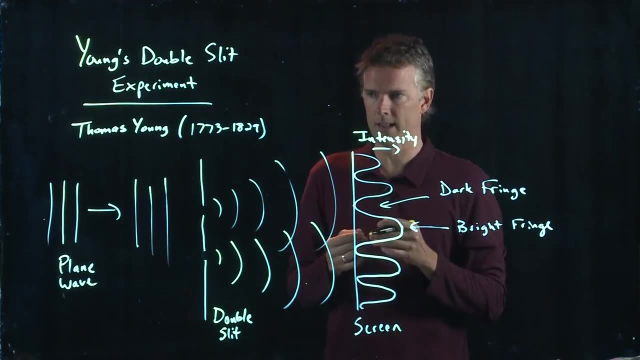 You're actually adding more noise and yet all the noise goes away. okay, And it's because of this wave nature of light, And this was one of the very first experiments to really demonstrate that light is a wave. Okay, It's not just rays flying around in straight lines. 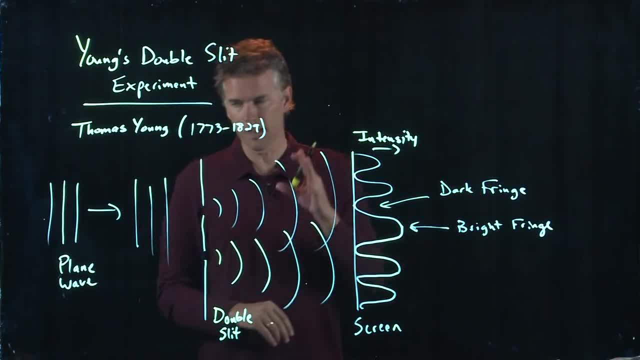 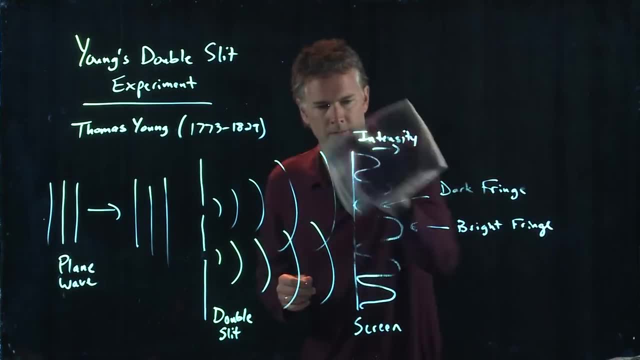 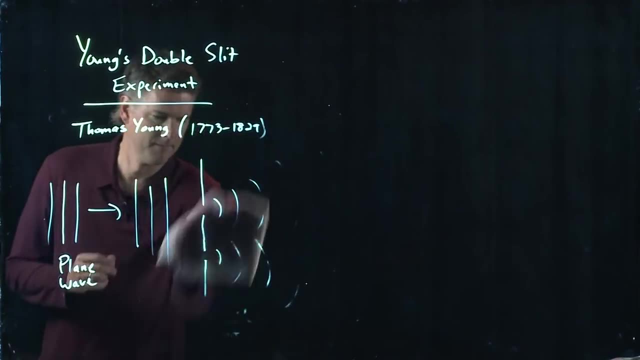 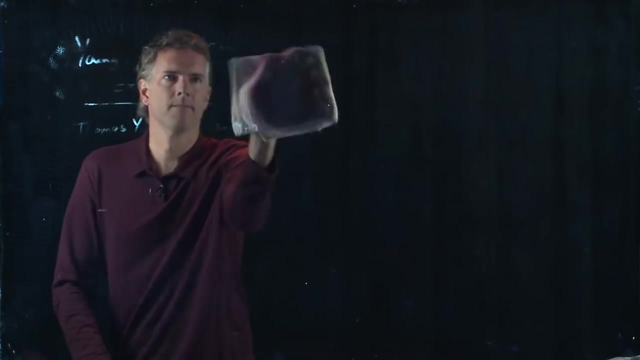 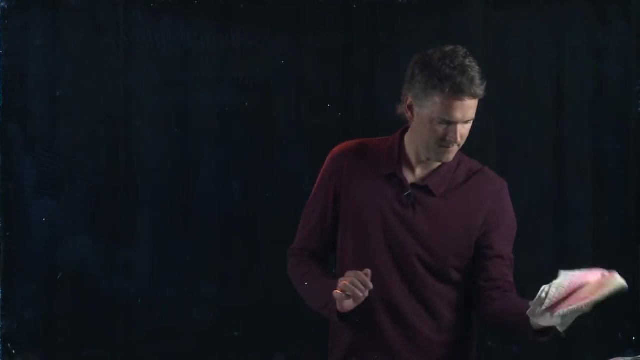 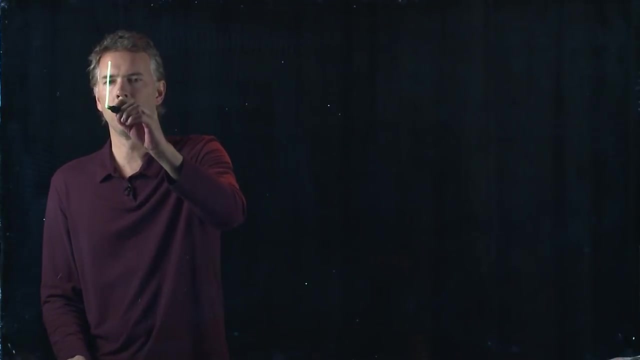 There's more to it. Okay, It's much more complicated than that, So let's see if we can understand this experiment in a little more detail. So let's just draw this portion of our picture. Here's our double slit. 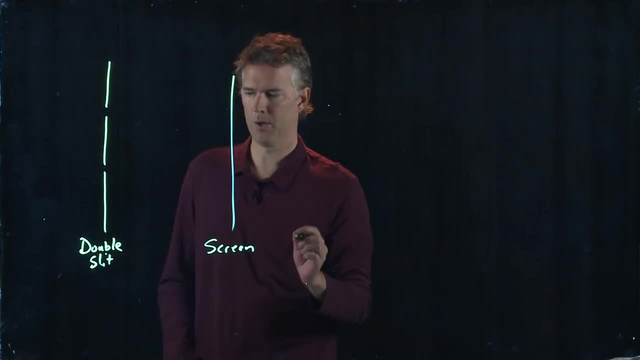 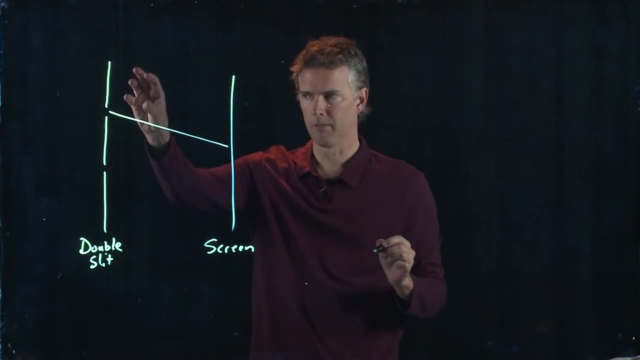 Here is our screen where we're going to capture our picture. And now let's think about this: There's some propagation of light from the top. Okay, From the top slit to the center of the screen, And let's call that L1.. 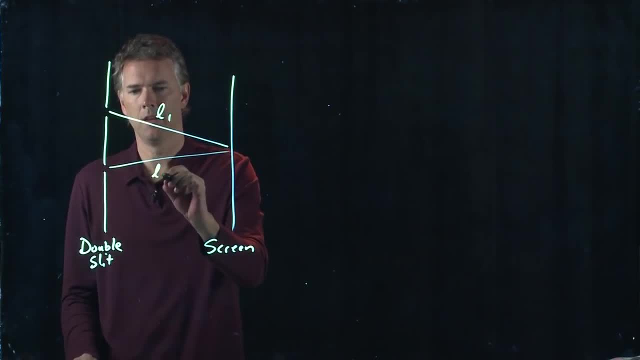 There's some propagation from the bottom slit to the screen, And let's call that L2,. okay, And if these are exactly equal, then we're in the center of the screen. okay, And if L1 equals L2, then the wave coming from L1, which is going to look like this: 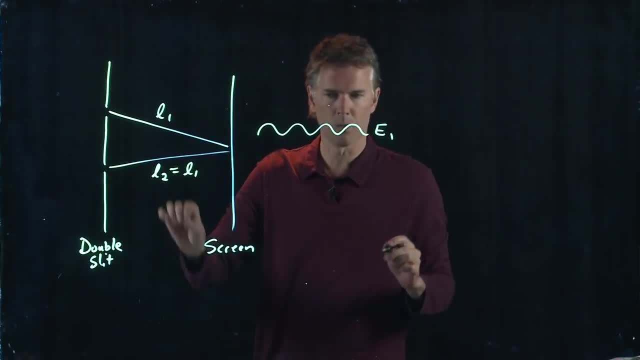 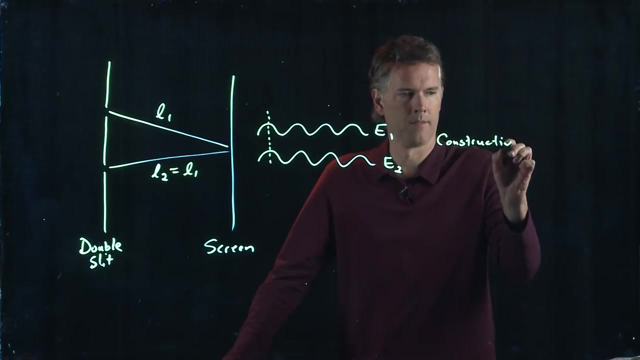 is exactly in phase with the wave coming from the second slit. Okay, Got a little mushed over here on the right side, But they're supposed to be lined up in phase And that means that we have constructive interference. and when we have constructive interference, 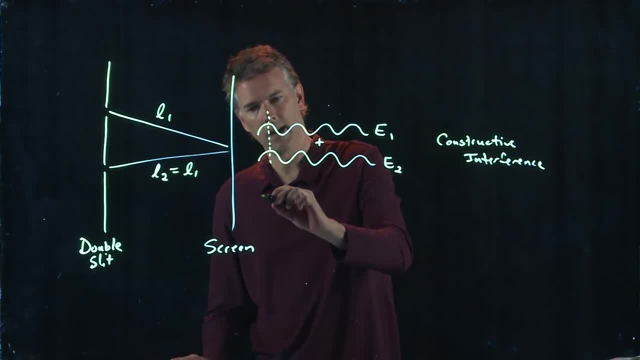 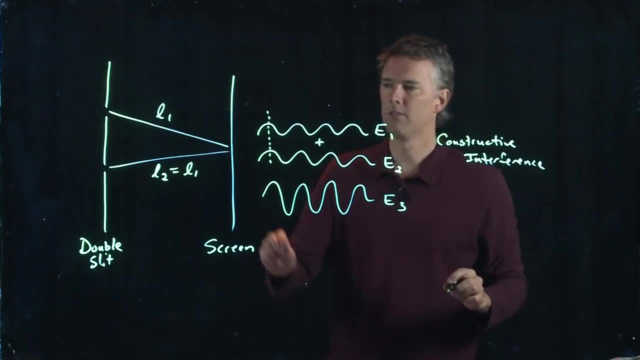 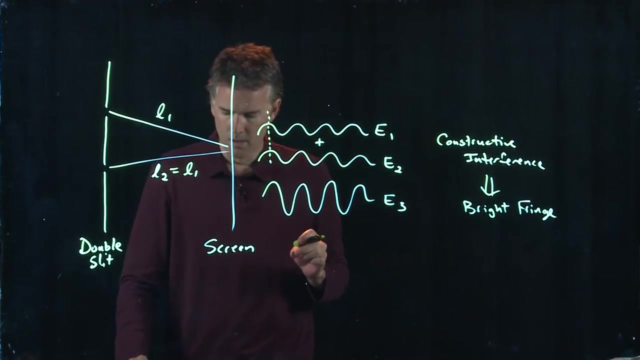 We get a maximum. So when I add those two things together I get something much bigger than each one individually. So in the center of that screen you've got a bright fringe, a region of maximum intensity. But let's shift this a little bit. 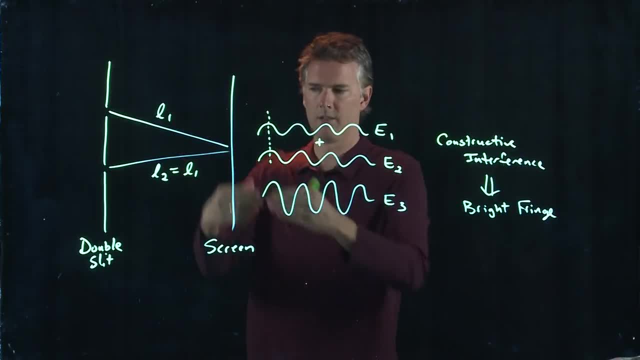 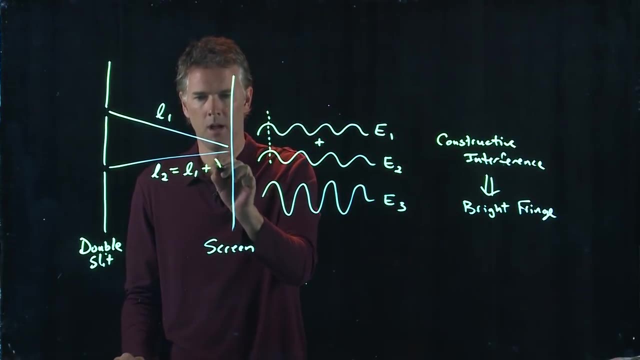 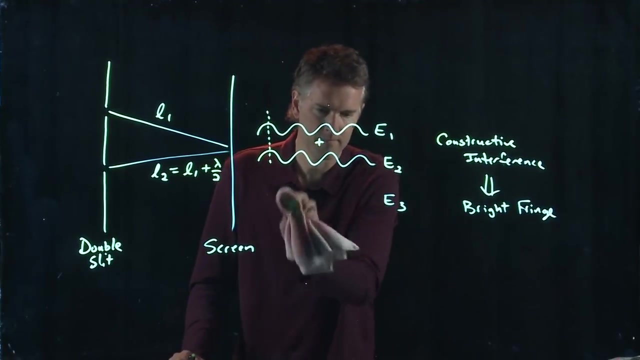 Let's move this position up slightly, such that L1 and L2 are no longer equal. We're going to let L2 go a little bit further than L1.. So let's say that this is now lambda over 2 further. Okay. 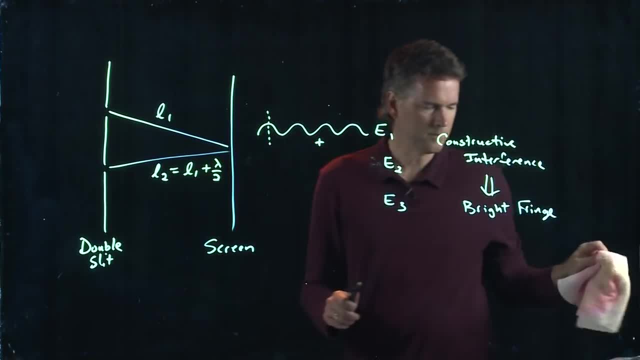 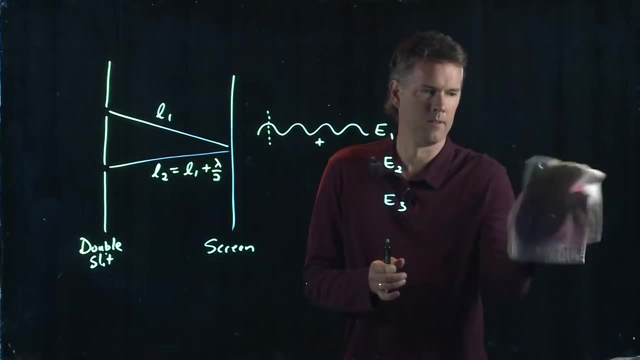 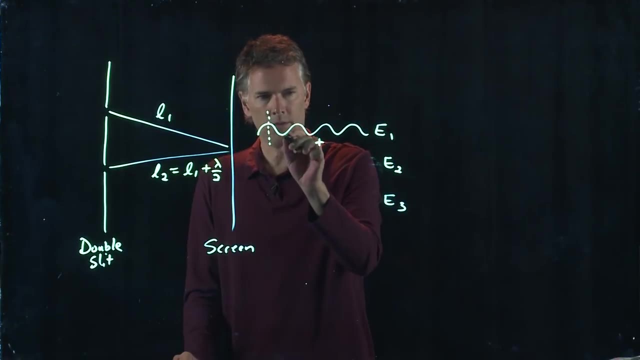 Okay, Okay, Okay, If I shift it by lambda over 2, let's see what happens. So if I shift it by lambda over 2, that wave that was looking like this now in fact gets flipped over, And we know what happens when you add a wave to its inverse. 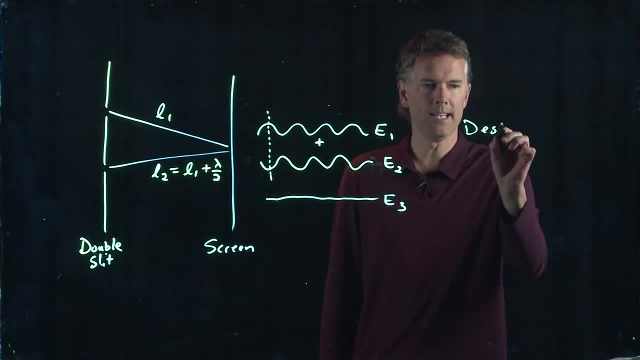 So we now get a flat line that is destructive interference. Okay, And that is our dark fringe. If I keep moving this position, I'm going to get bright fringes and dark fringes and bright fringes and dark fringes. 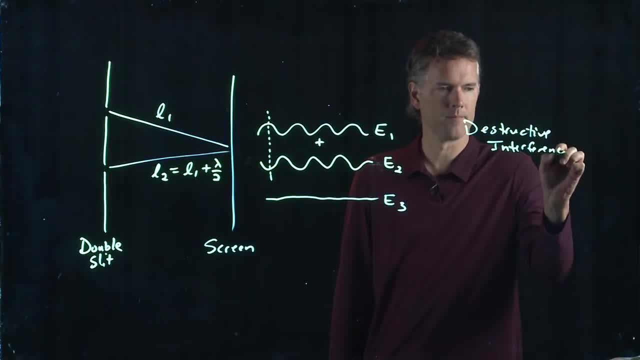 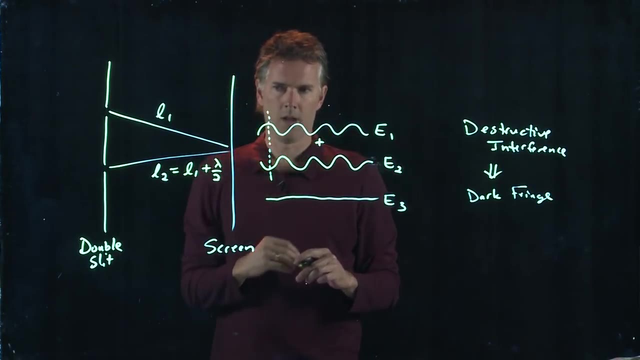 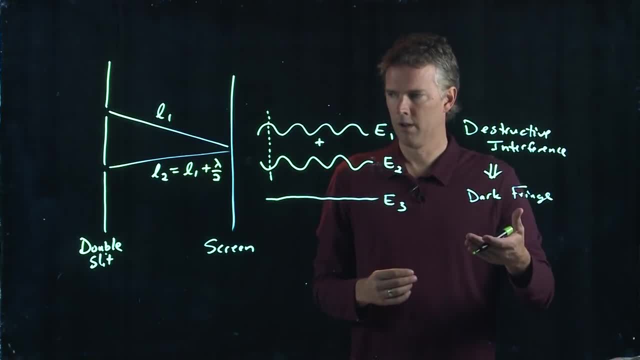 Okay, Okay, Okay, Okay, Okay. For instance, if I change this from lambda over 2 to lambda, then I'm back to the constructive case, because I've shifted E2 by one whole wavelength. It looks exactly like E1.. 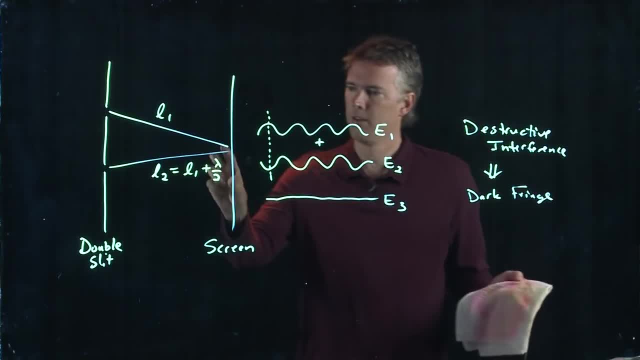 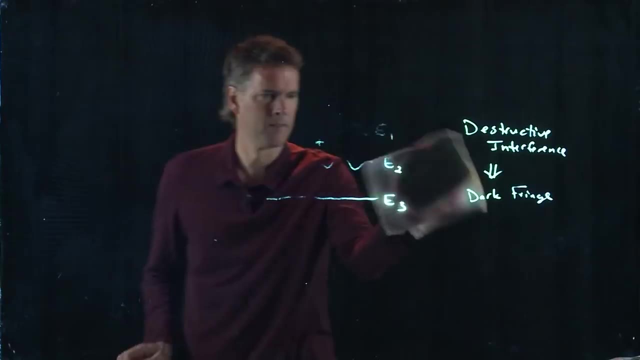 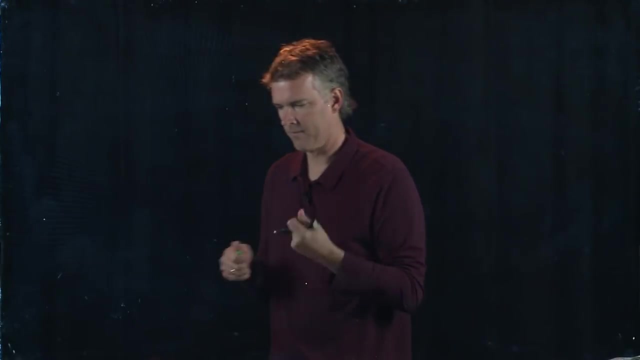 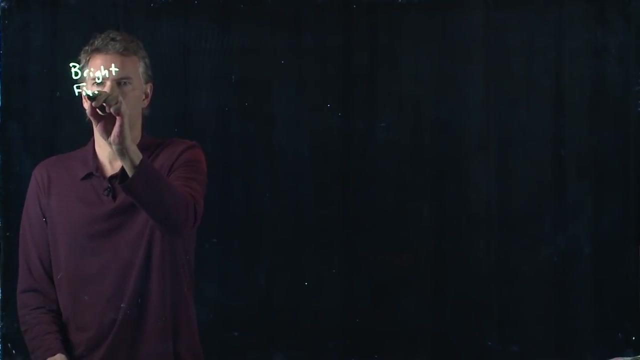 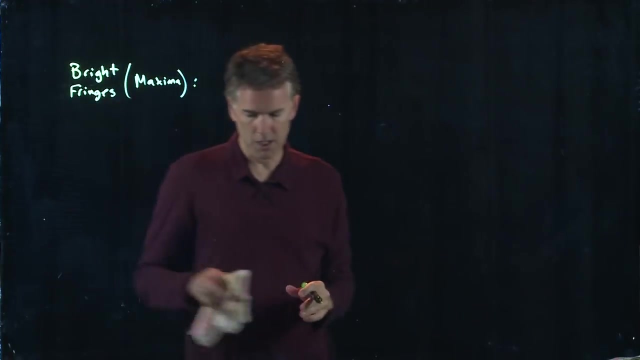 So there are conditions for this geometry and it's dependent on the wavelength. How many waves are you adding to one path versus the other? Okay, The bright fringes are called maxima. The condition for the bright fringes is the following: 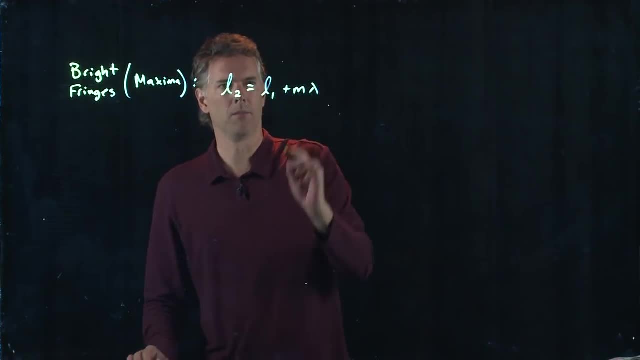 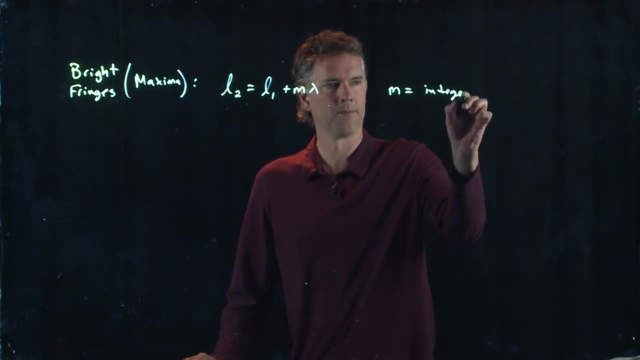 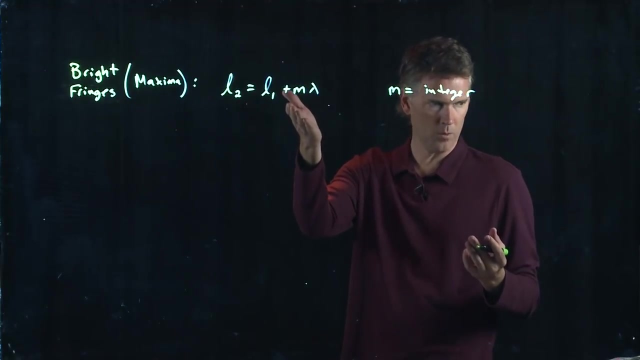 L2 has to be L1 plus some multiple of the wavelength. M is an integer, So if it's zero, then the lengths are exactly equal. we get a bright fringe. If you're adding one wave to L2, then you still get a bright fringe. 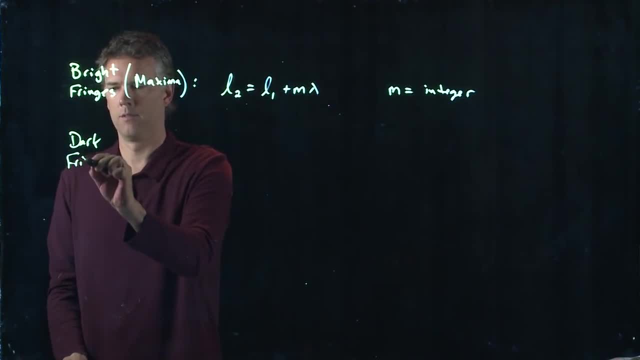 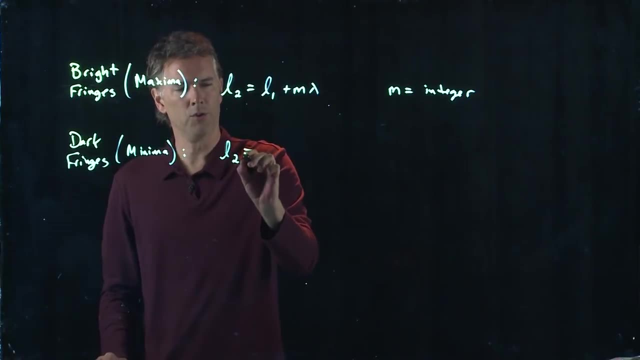 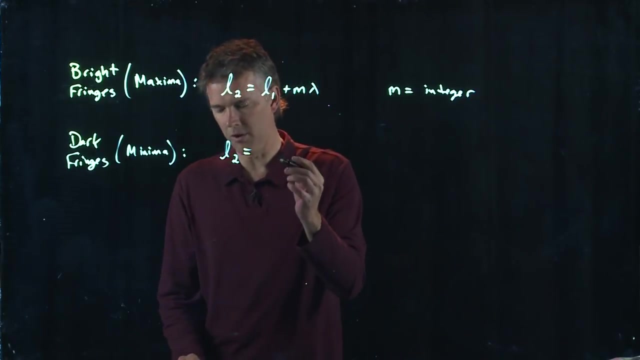 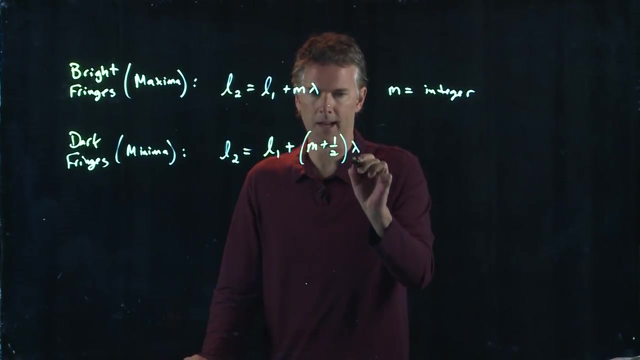 The dark fringes. Okay, Okay, Okay, Okay, Okay, Okay. Which are the minima are when L2, you're going to add a half a wavelength, or one and a half wavelengths or so on, So this becomes L1 plus m plus one half lambda. 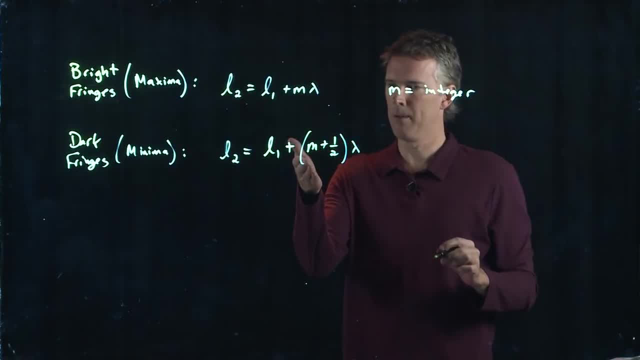 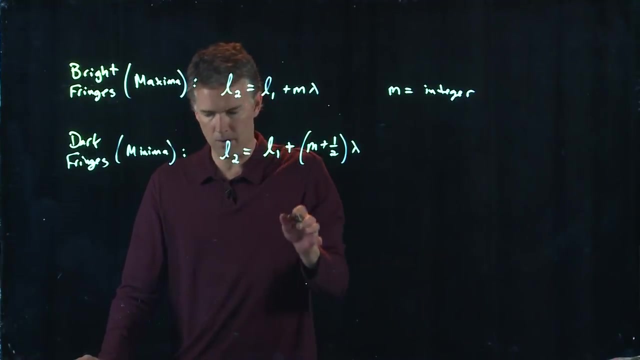 Okay. So again, m is an integer- 0,, 1,, 2,, 3, and so on, But it can also be negative. Negative just means the bottom half of the screen. Okay, so let's see how this now applies to the geometry of that picture. 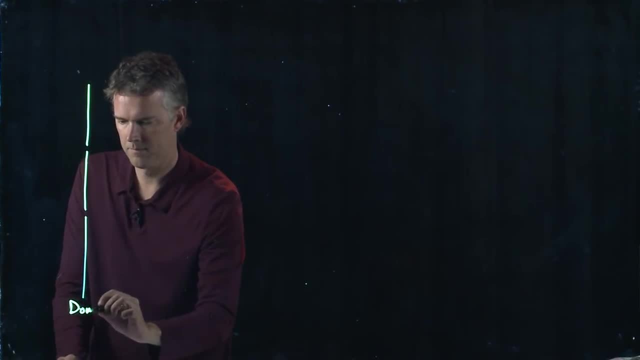 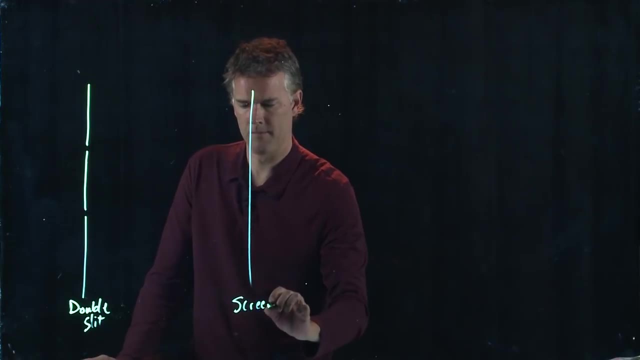 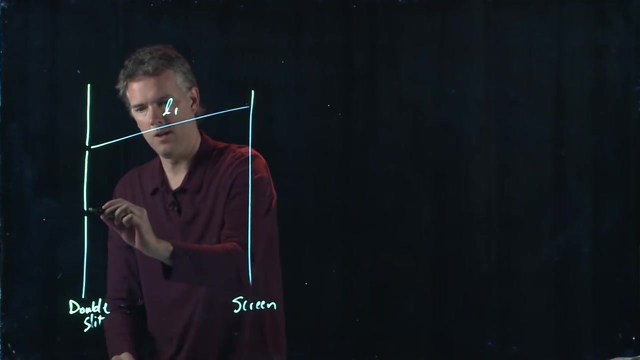 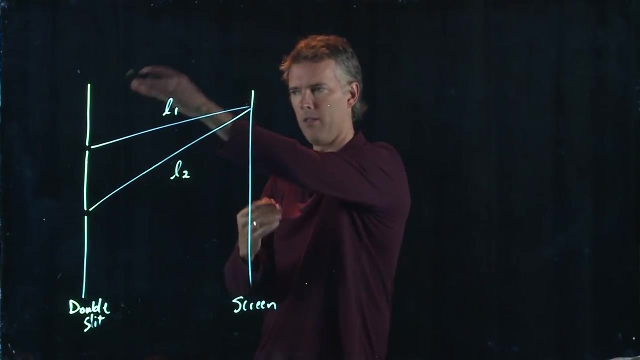 Okay, there's our slits, here's our screen, and now we're going to draw L1 coming way up here, L2 coming up to the same point. Anytime you're looking at a point on the screen, you have to worry about the fields from the first slit and the fields from the second slit. 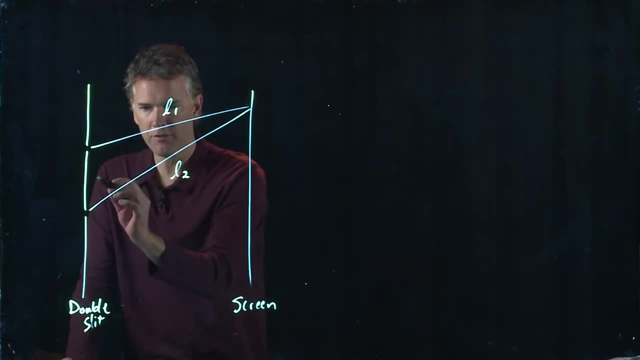 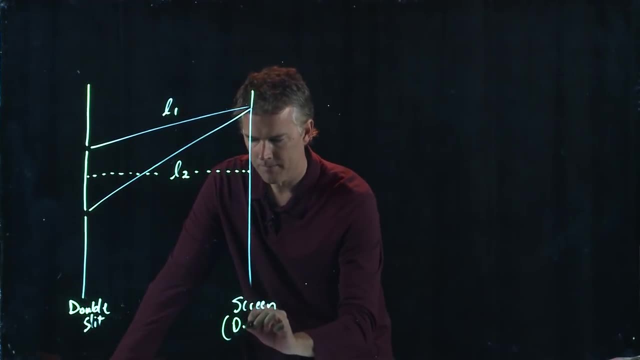 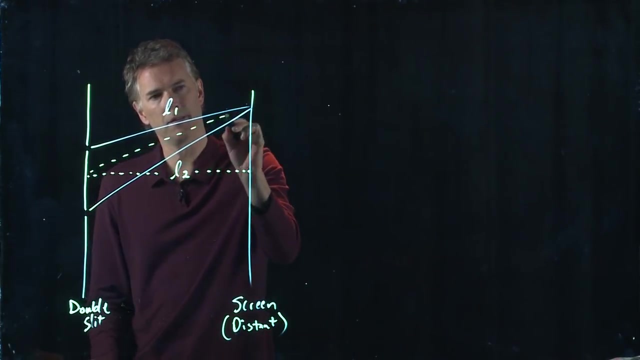 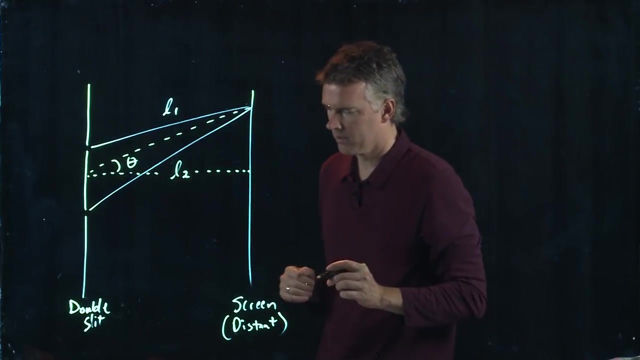 because you of course have to draw them. You have to add those up Now. if this screen is very far away, then we can say the following: There is some central angle here, theta, which is approximately the same for each of those slits. 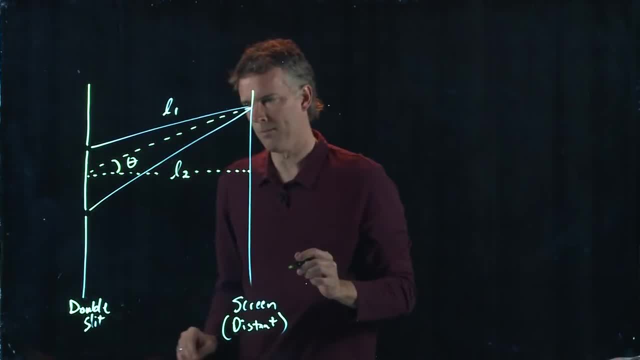 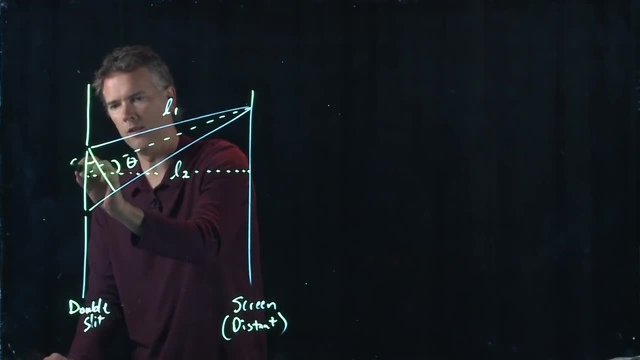 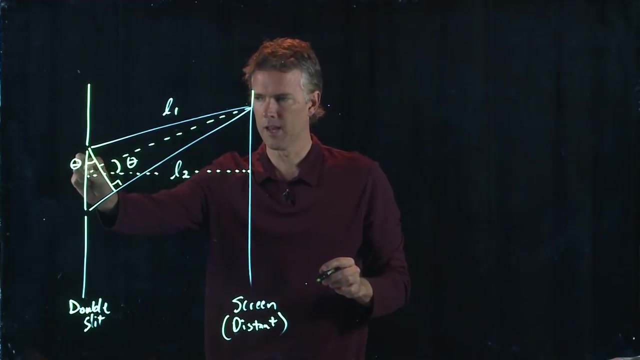 And now here's where a little bit of geometry comes into it. If this is angle theta, you might be able to convince yourself that this is also angle theta, right there, If I make a right angle, and this angle is theta as well as that angle. 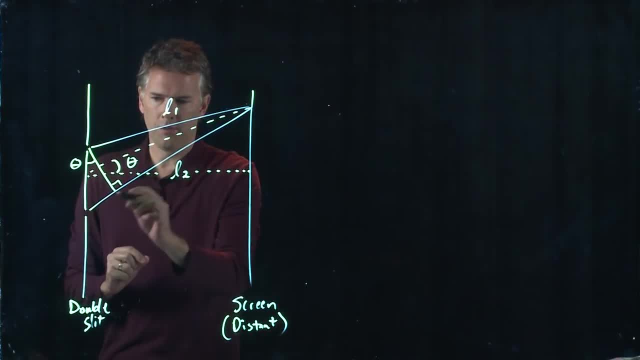 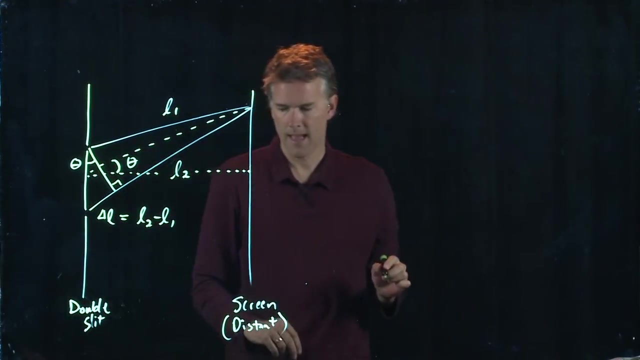 Okay, L2 is this whole length, and it consists of this portion plus this little delta L. Okay, And the delta L here is just going to be the difference between the two, l2 minus l1, and so that little difference is what's important in the interference pattern that we're. 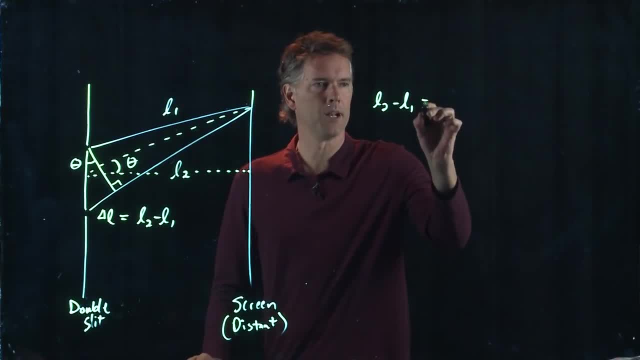 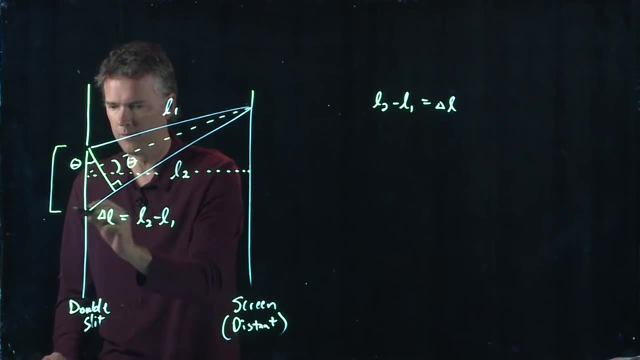 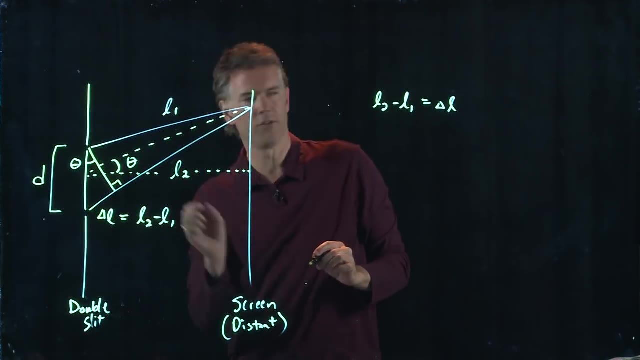 going to see on the screen. l2 minus l1 is equal to Delta L, but if the distance between the slits is d, then this little side of that triangle is just d sine theta right. theta is up there, this is the right angle, and so this side of the 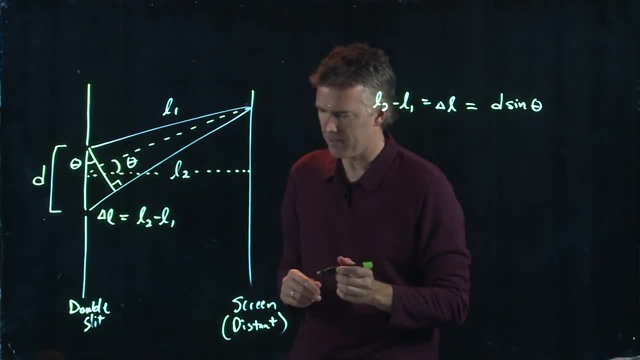 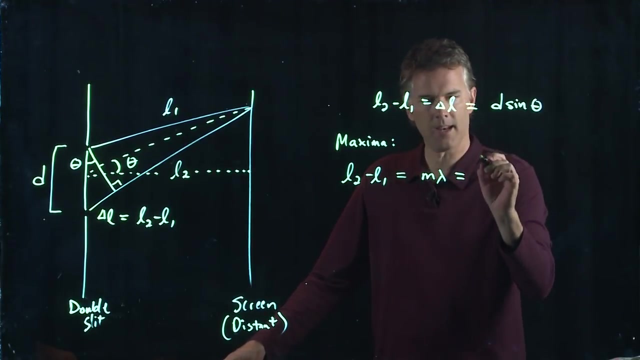 triangle. it's opposite the angle, so that is d sine theta. all right, what are the conditions for maxima? the conditions were L2 minus L1 had to be equal to m lambda. but we also know that L2 minus L1 is equal to delta L, which is d sine theta. 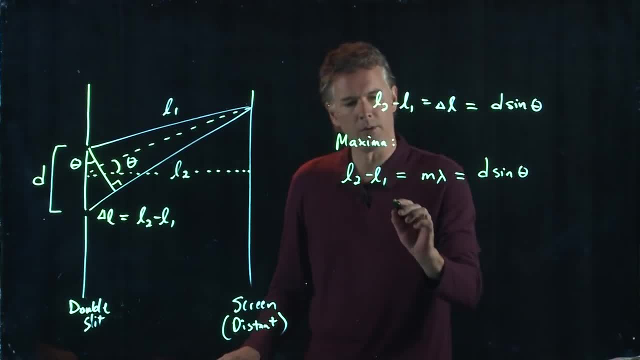 And so we have this nice relationship here. for maxima d sine theta equals m lambda. If you know your slit spacing, if you know your wavelength, you can predict exactly where those maxima are going to be on the screen, what angle they're going to be at. What about the minima? 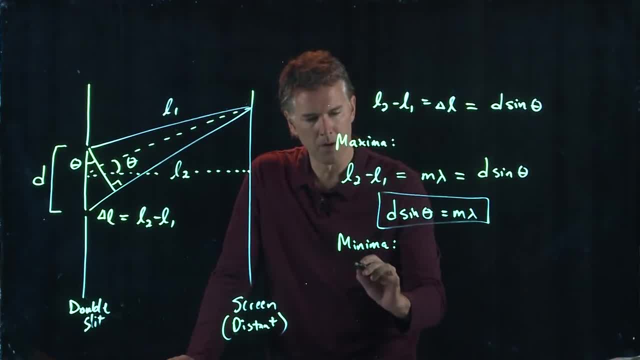 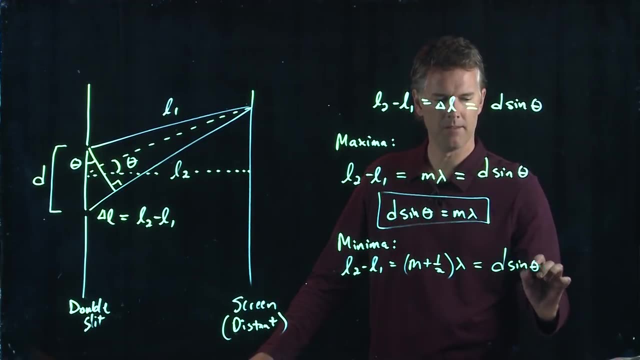 The minima we said, L2 minus L1, has to be m plus a half times lambda. L2 minus L1 is still d sine theta, And so we get the equation for minima, which is the following: d sine theta equals. 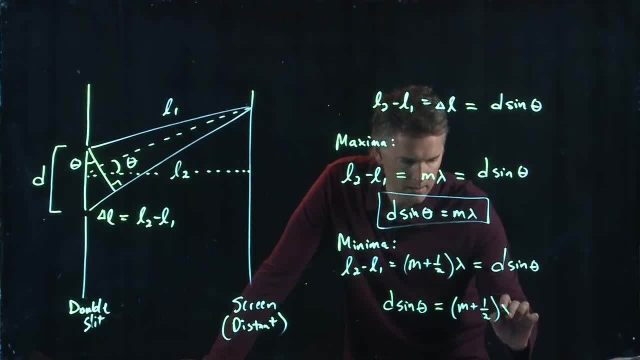 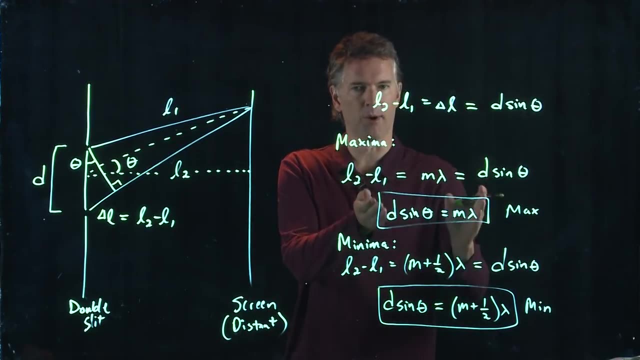 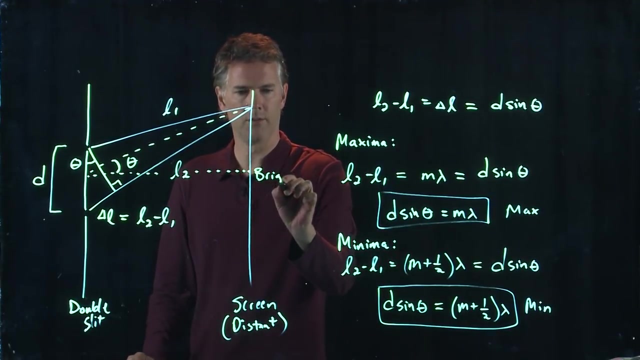 m plus a half times lambda. This is max, this is min. This is where your dark fringes are. this is where your bright fringes are. So, as you go up and down this screen here, you're going to have bright fringe, dark fringe. 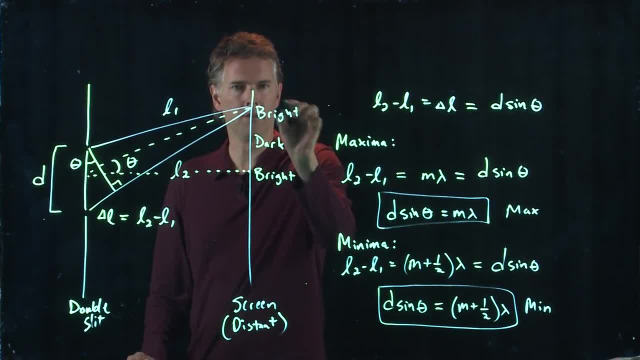 bright fringe, dark fringe, and it's just going to alternate back and forth. But going the other way you get the same thing: Dark fringe, bright fringe, dark fringe, et cetera. It keeps going out for quite a ways. 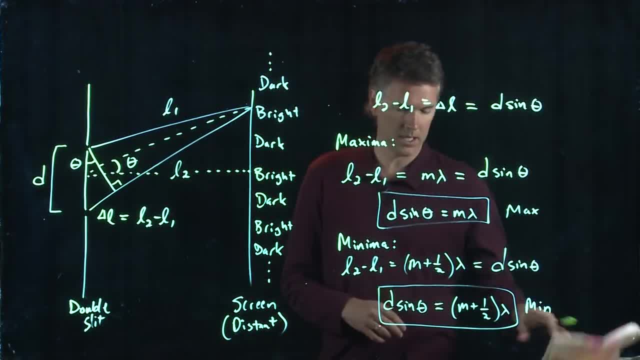 All right. so this was obviously a very strange notion back in the 1800s that you could make light disappear by adding more light. But what is also really cool about this equation right here is it is a way to measure the wavelength of light. 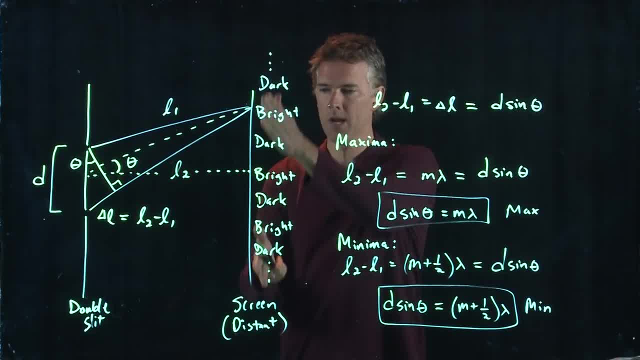 If you send light into these double slits and you can measure the spacing of these fringes on a screen, you can go back to this equation and figure out exactly what the wavelength of light is. And the wavelength of light is pretty small, right. 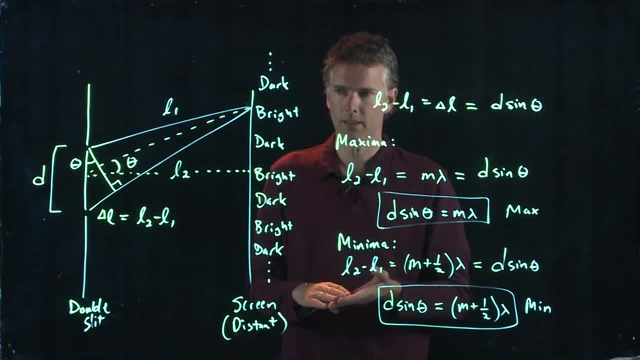 A Heaney laser beam, like we talked about, has a wavelength of 633 nanometers- Really really small, And yet here's a very simple way to measure it. All right, with that in mind, let's take a look at one of your homework problems. 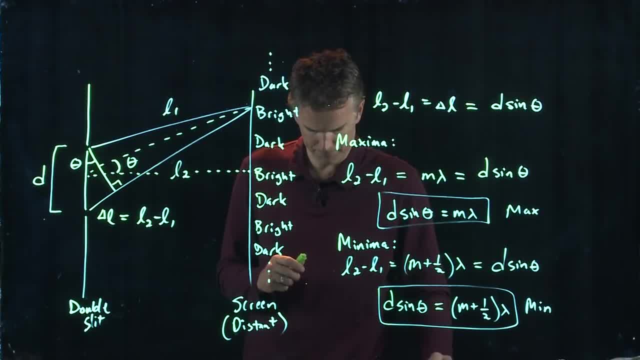 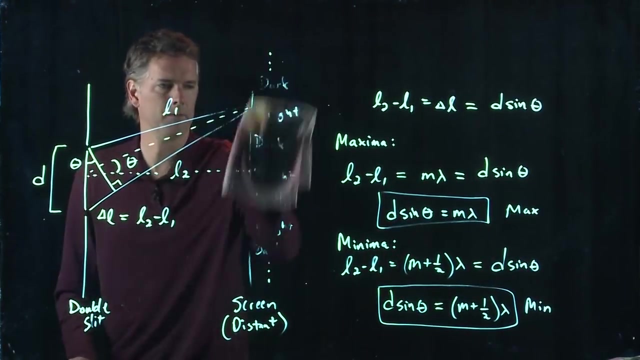 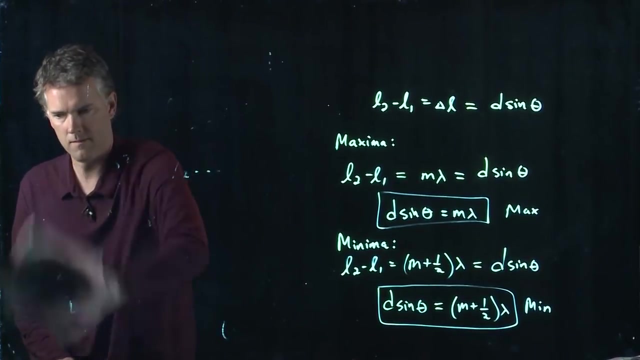 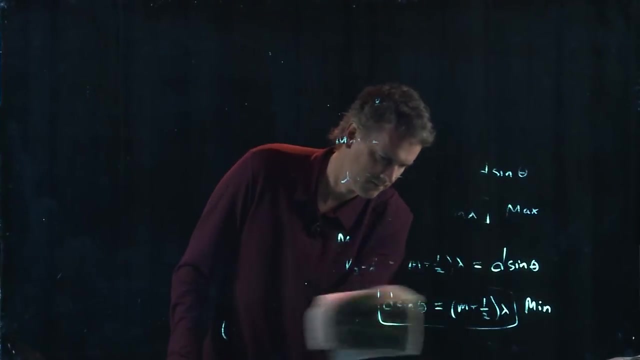 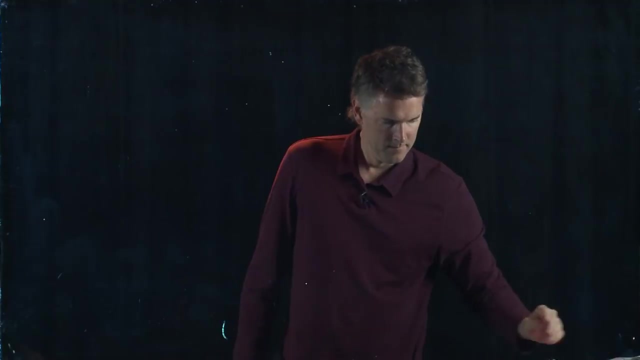 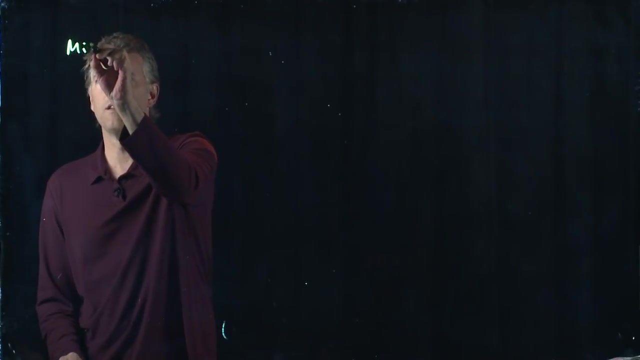 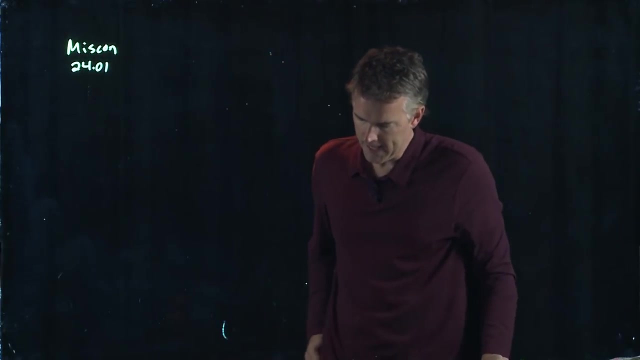 Samuel, if you want to switch the other screen active, Okay, and let's just start right at the beginning. Let's look at the Misconceptual Question 2401.. Okay, so this is Misconceptual Question 2401.. 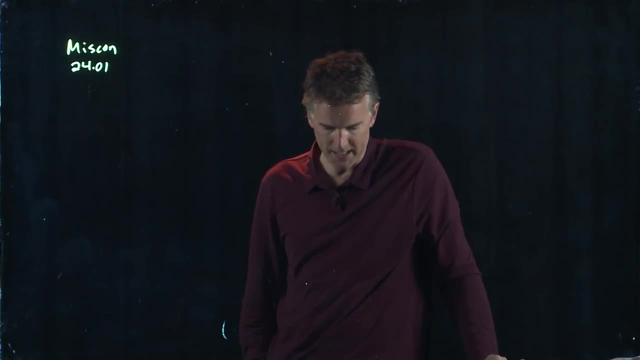 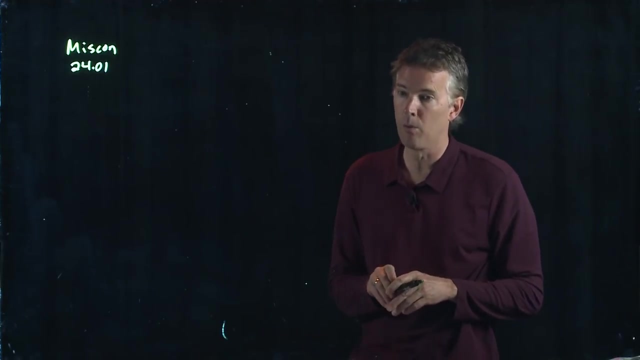 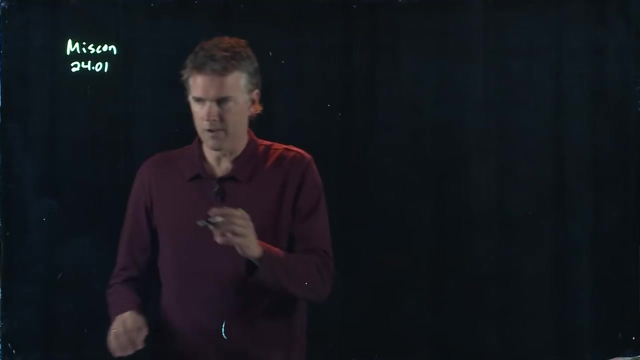 It says Light passing through a double slit arrangement is viewed on a distant screen. The interference pattern observed on the screen would have the widest spaced fringes for the case of what. Okay, so let's see how this works. We've got our double slit. 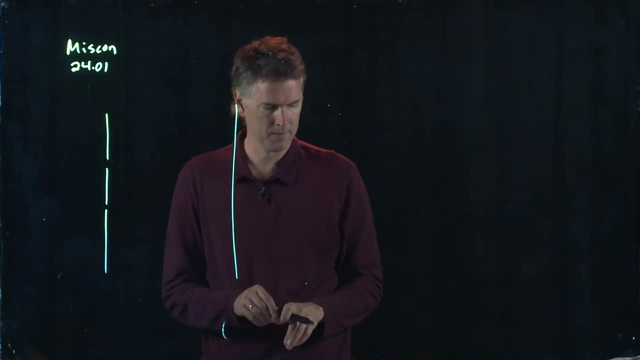 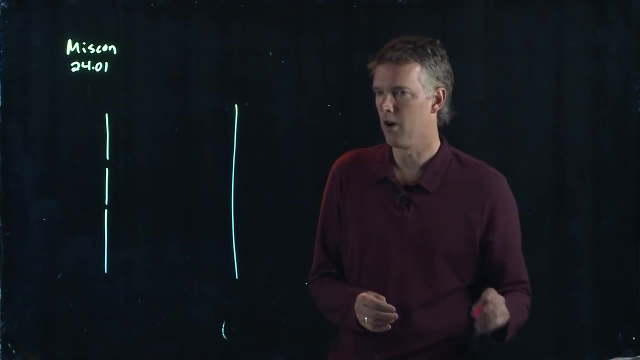 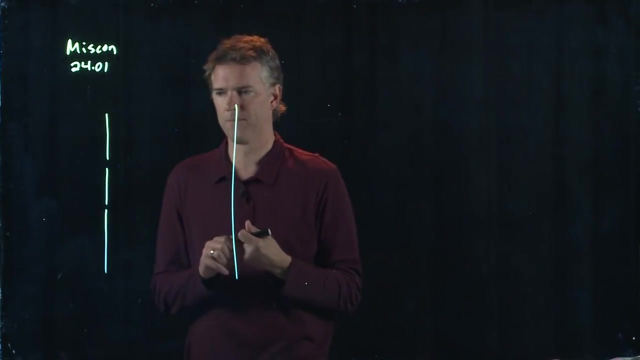 and now we have a distant screen And what we know is there's going to be regions of bright and dark fringes on this distant screen, And let's draw two different colors and see if we can figure out exactly where those are. Okay, there's going to be bright fringes that look like this: 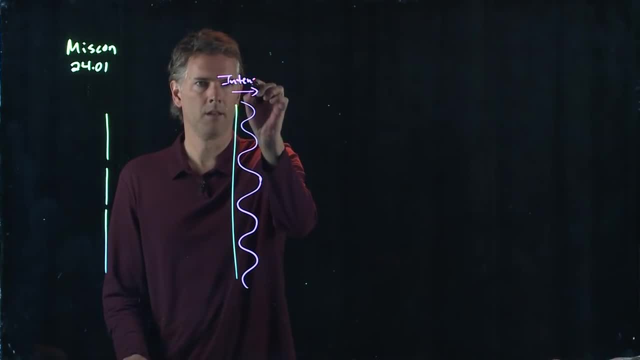 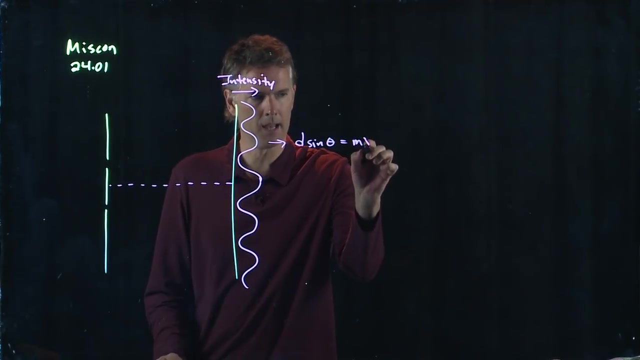 Okay, I've drawn the intensity big to the right. So we know along the center line we have to have a bright spot. But the second one here is going to obey the equation d sine theta equals m lambda. And it's the first bright fringe that we come to. 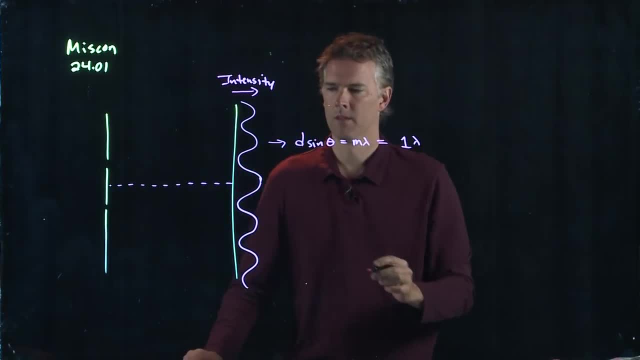 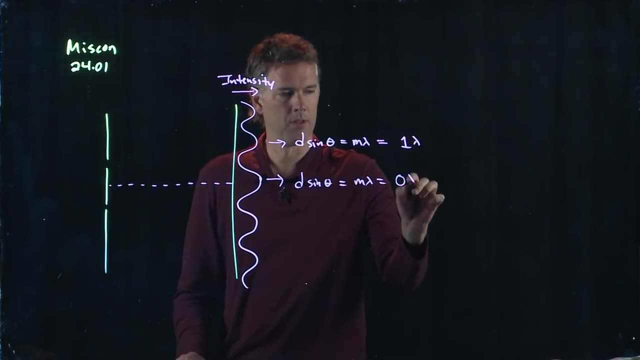 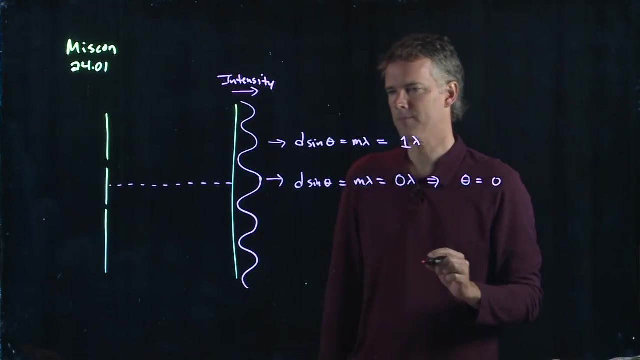 So this is one lambda. This one was the zeroth, This one is the fring. So for this one we have. theta equals zero. For this one we get what? Well, we can just solve this equation. Sine of theta is going to be lambda over d. 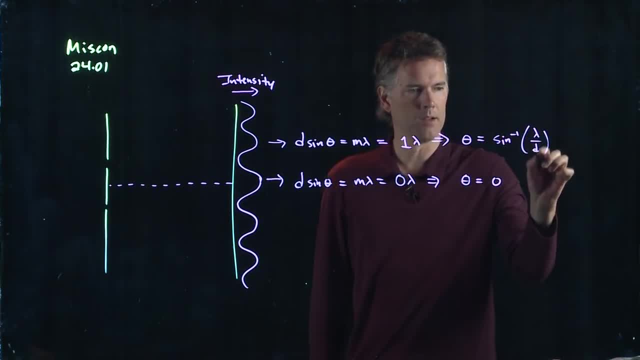 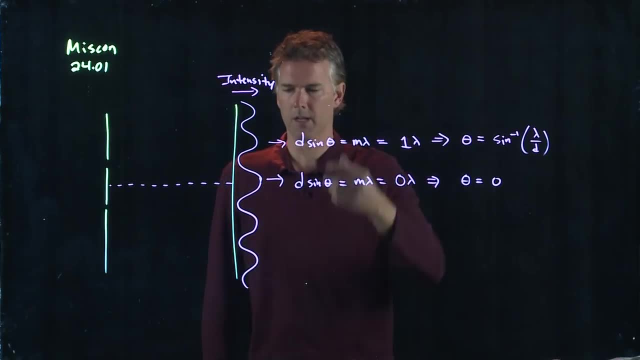 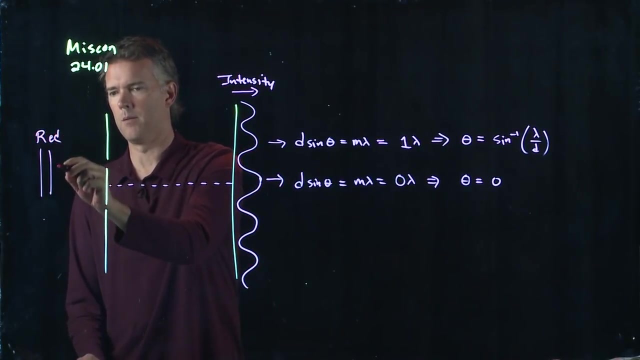 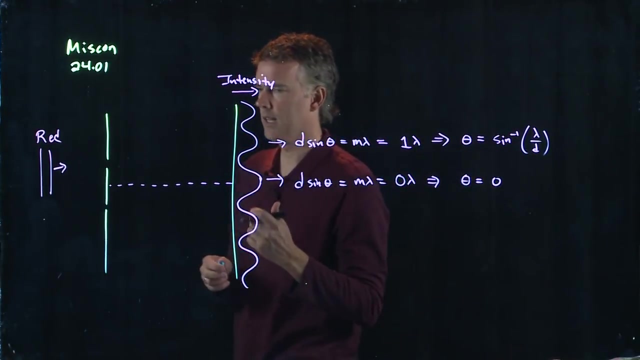 So theta is the arcsine of lambda over d And the next one is going to be 2 lambda over d, and so forth. All right, so this is for red light coming in. But let's say we switch now to blue. Okay, let's take blue light and send it in. 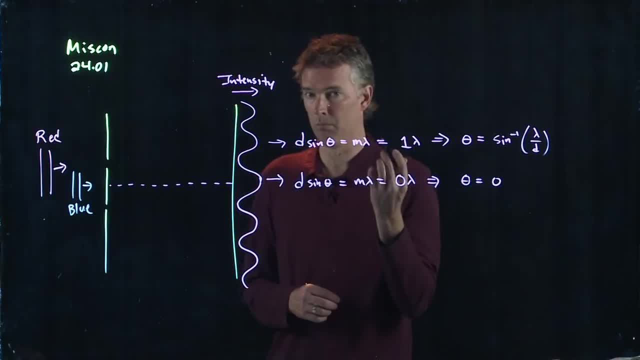 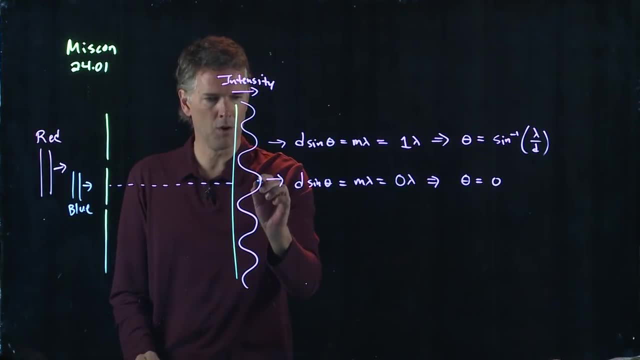 And let's figure out where the intensity pattern is going to be. for blue. Blue is, of course, shorter wavelength. The first intensity peak is always at the same spot. It's going to be right at the center line, But the next one is going to be a little bit closer. 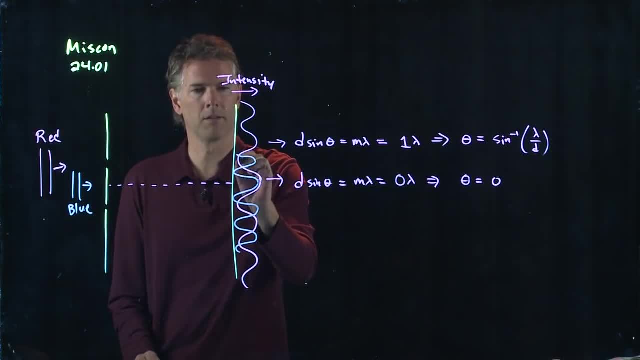 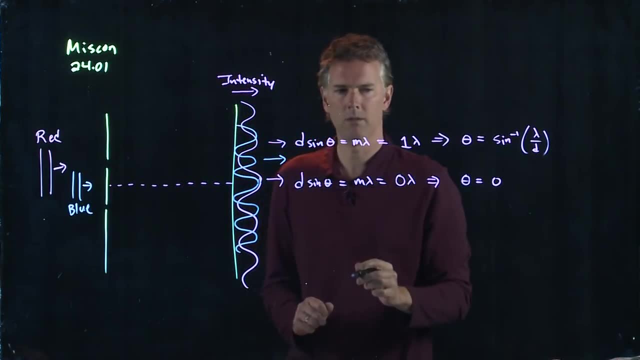 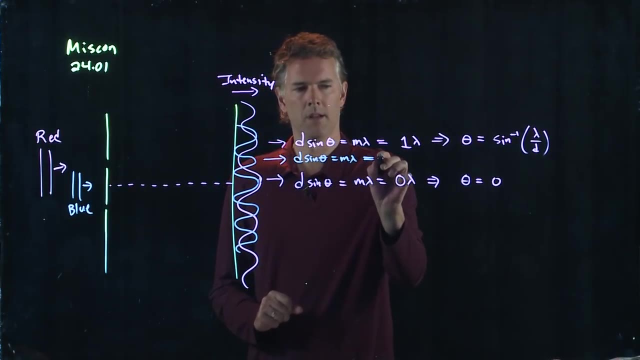 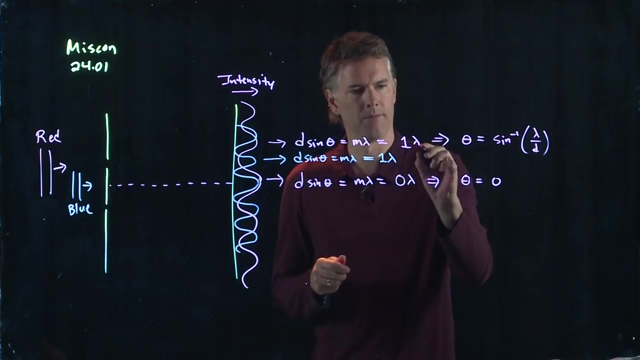 And so it's actually going to look like this. Okay, how do we know that? Well, we have the same equation d sine: theta equals m lambda Equals m lambda equals 1 lambda. But this lambda up here was for red. 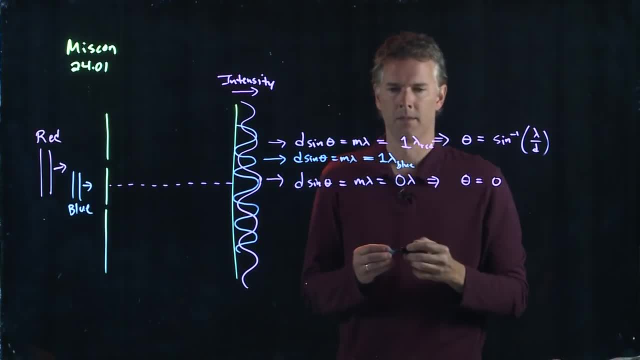 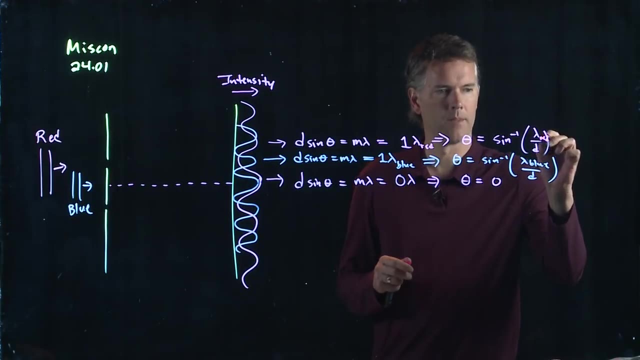 This lambda down here is for blue, And so for this equation we get: theta equals the arcsine of lambda blue over d. Where's the other one? It's lambda red over d. Now, let's make sure that that works right. 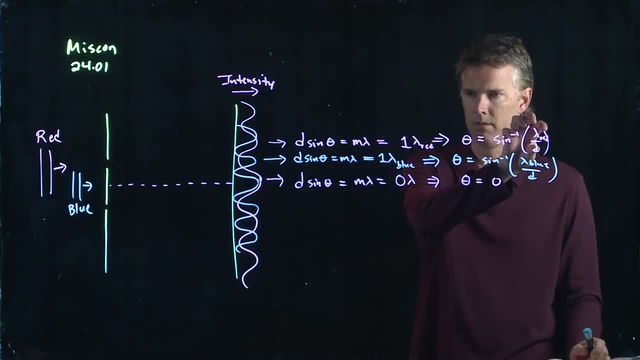 If I take the arcsine of a big number, do I get a bigger angle? Yes, Okay, you can convince yourself on your calculator. But as the argument gets bigger, the angle gets bigger. Okay, since lambda blue is less than lambda red. 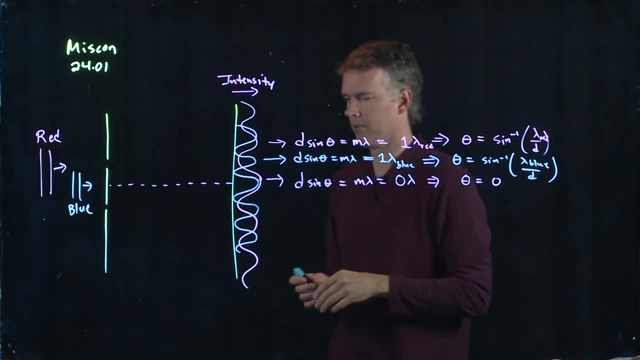 this angle, for blue certainly has to be less than red. All right, So we've distinguished between these possibilities here, because they're talking about red light or blue light, And so we know that the first one red light and a small slit spacing. 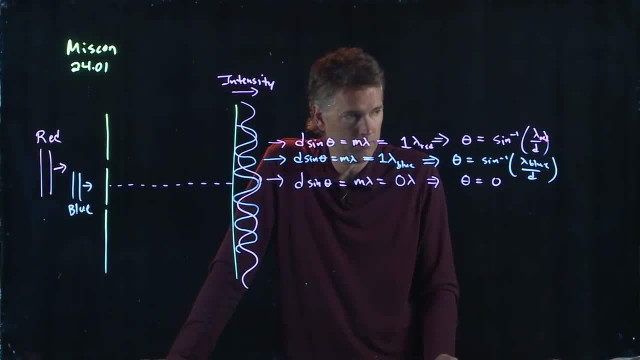 maybe will give us a wide space fringes. That seems pretty good because lambda will be big, d will be small. Let's see if we can eliminate the other ones. Blue light and a small slit spacing. That's not going to do it right. 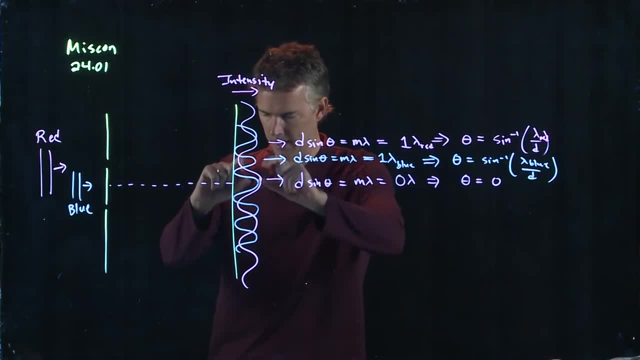 Those things are closer together, Those fringes are closer together for the blue, Blue light and a large slit spacing. That doesn't seem very good either, because d is in the denominator. So as that gets bigger, this angle in fact gets smaller. 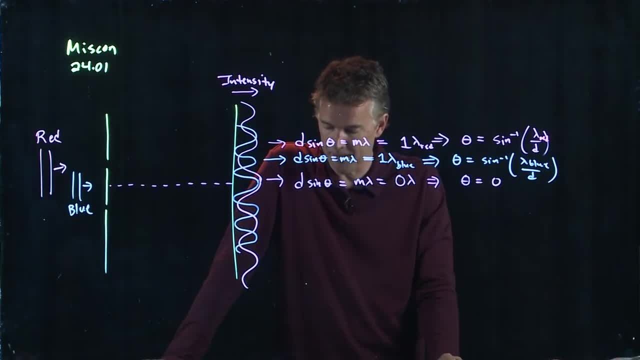 And then the last one, red light, and a large slit spacing. So we're between 1 and 4, and the large slit spacing means that this number gets small. If that number gets small, theta gets small. That's not what we want. 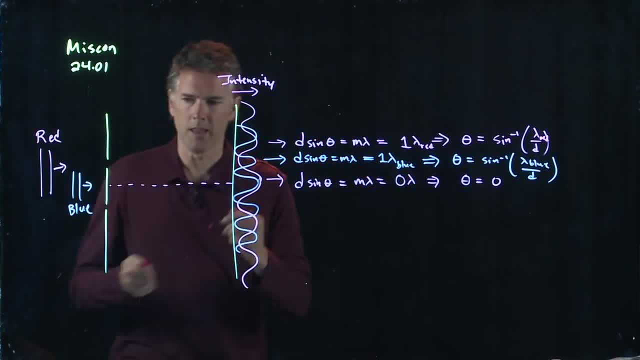 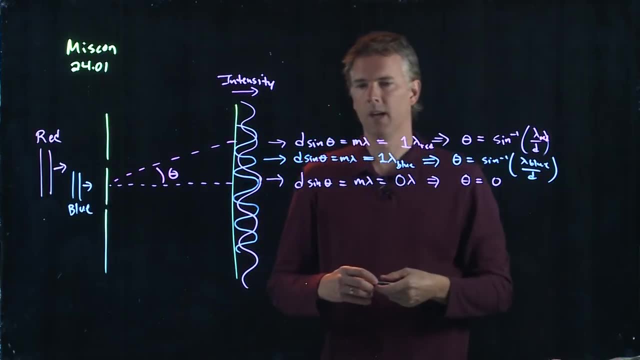 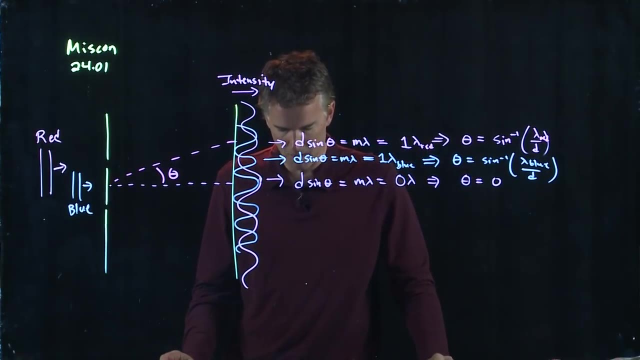 We want theta big. Remember theta is the angle to the fringe that you're interested in, And so as theta gets bigger, the fringe spacing gets bigger. So I would say we want the first one, red light, and a small slit spacing. 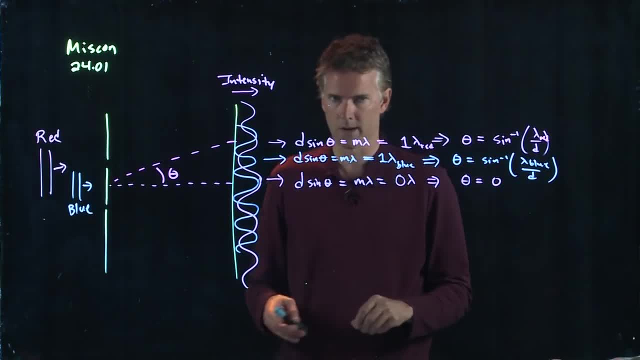 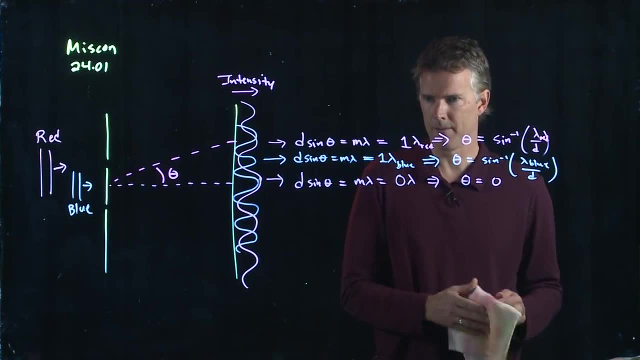 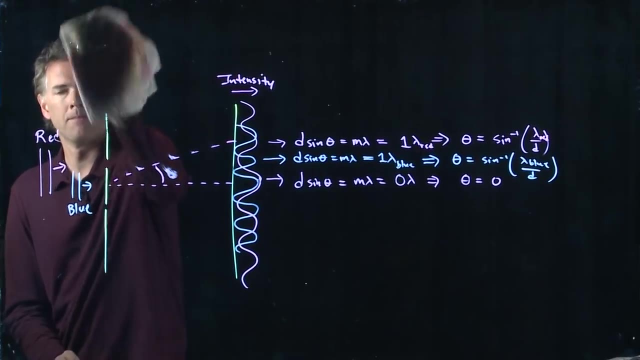 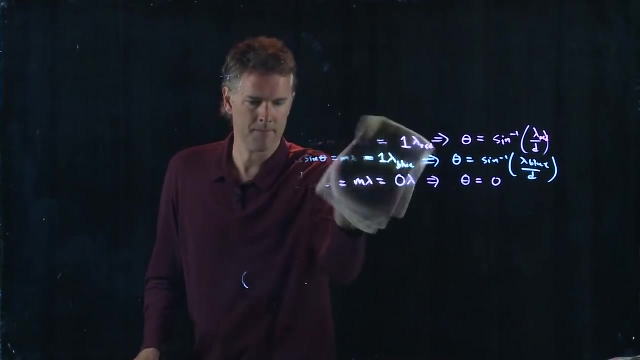 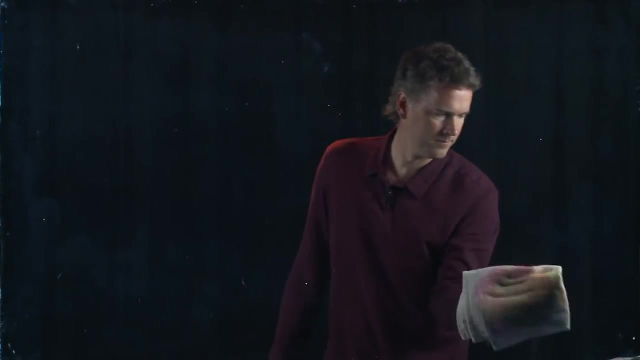 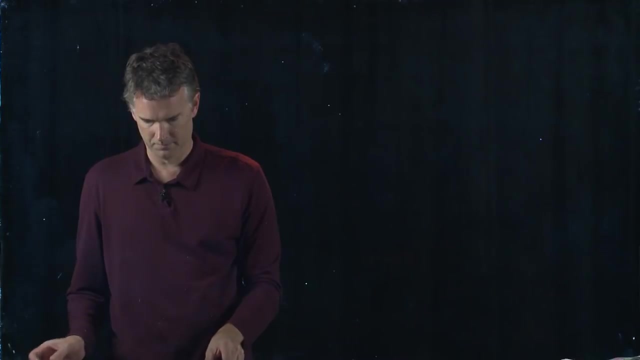 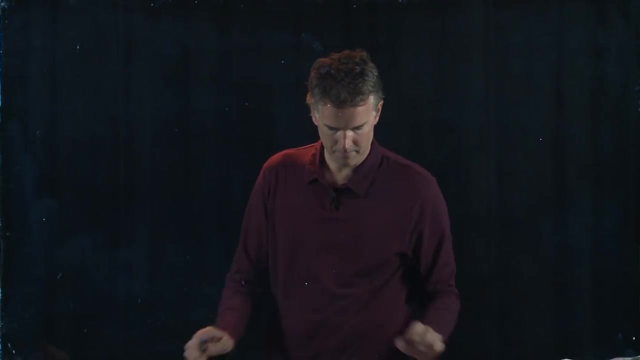 Let's try it and see if we're right, And indeed we are correct. Okay, Questions about that one. Okay, You can turn off that insert if you haven't done it already, Samuel Mm-hmm. Okay, So one thing that we had mentioned last time. 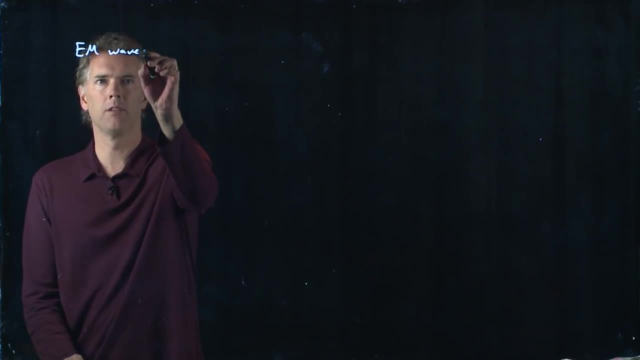 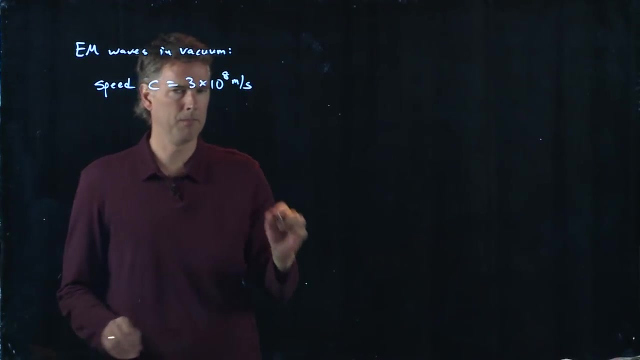 is that electromagnetic waves in vacuum have a certain speed, And that speed is of course 3 times 10 to the 8th meters per second, and we call that c. But in material they slow down a bit And there we get a speed v. 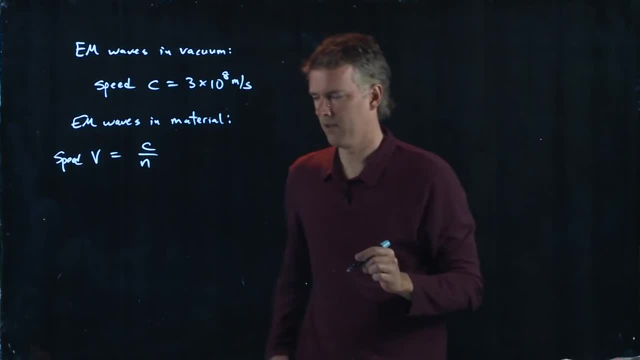 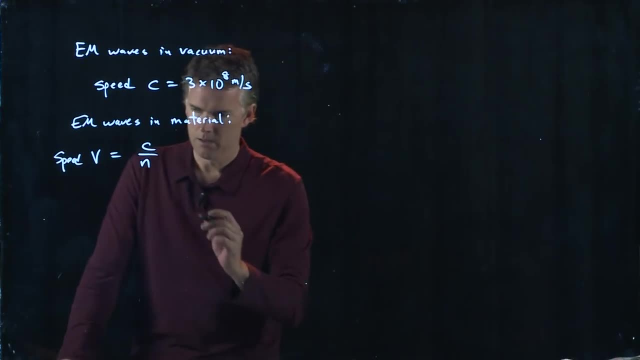 which is c over n. Okay, The index of refraction tells you how much that wave slows down. Okay, But we know that there is a relationship between speed and frequency And wavelength. Speed is equal to frequency times wavelength. So we have the following. 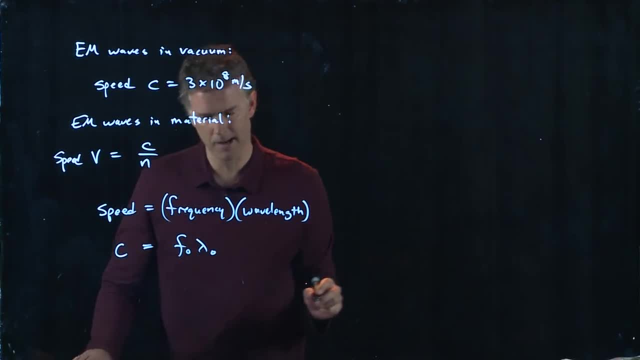 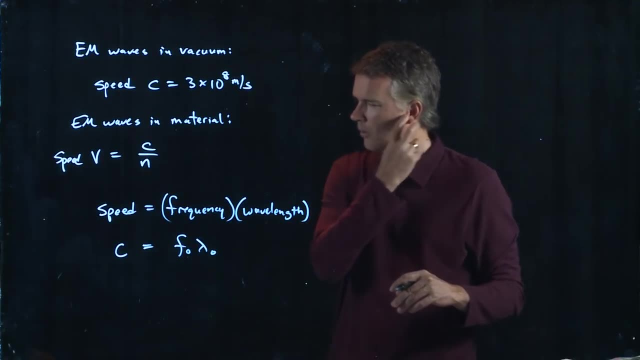 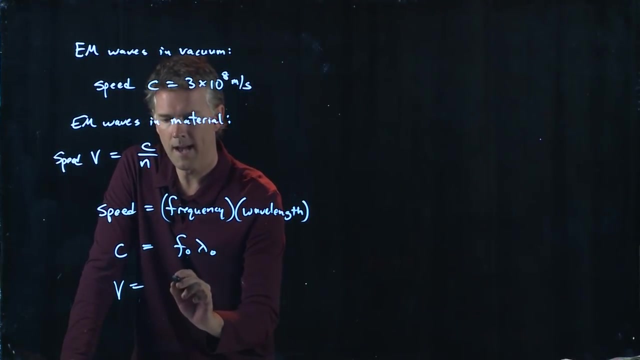 c is equal to f-naught times lambda-naught. What's the frequency of the wave in free space? What's the wavelength of the wave in free space? Multiply those together, you get the speed of light, c. But in vacuum we have c over n and that is lambda-naught, f-naught divided by n. 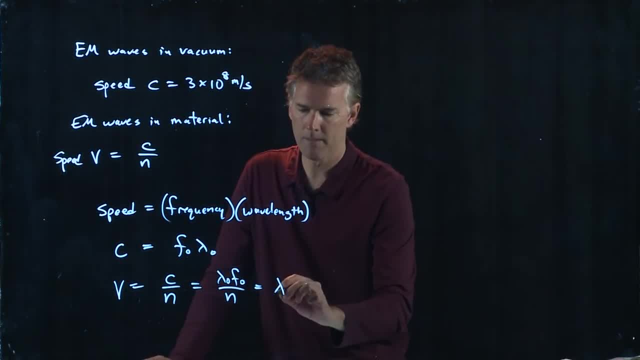 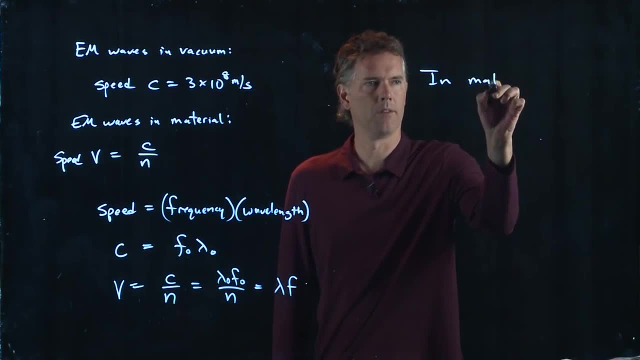 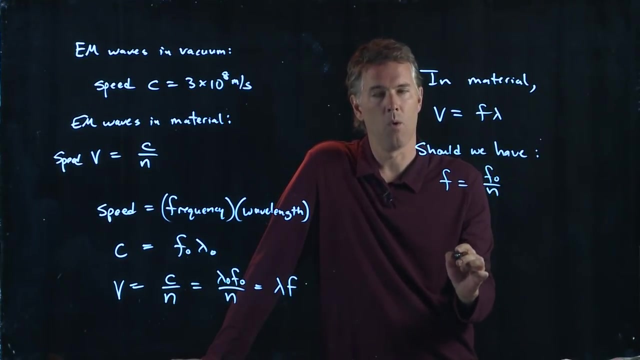 which is lambda times f. In material we get, v is equal to f times lambda, And so now the question is the following: Should we have frequency that changes, Or should we have wavelength that changes? We only have one n in there, so we're going to have to change one of these things. 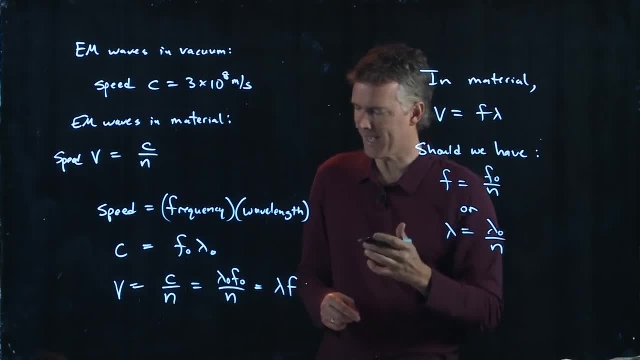 We've got to change the frequency or we have to change the wavelength when we get into material And, believe it or not, this is a debate that is still going on today. I heard a research talk last year by people. There are people that are still trying to sort of decide which is which. 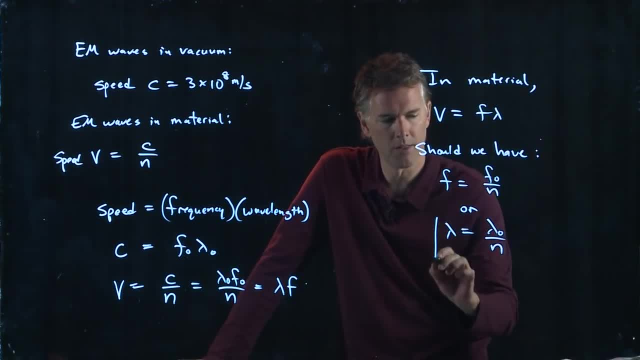 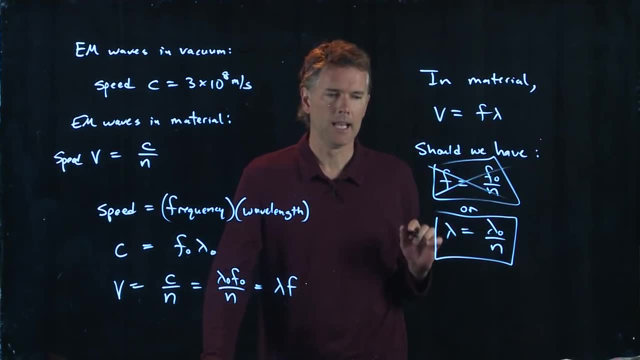 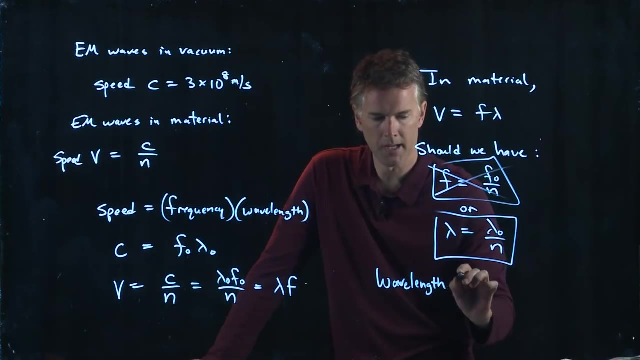 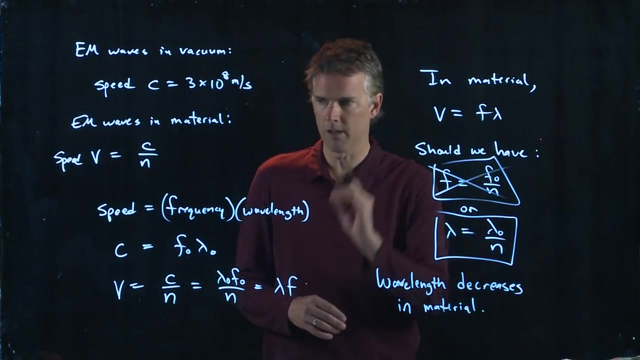 But currently the accepted notion is this: one changes, this, one does not. Lambda means wavelength and the current understanding is that wavelength decreases in material And your wavelength gets shorter. The frequency stays the same, but the wavelength in fact gets shorter. 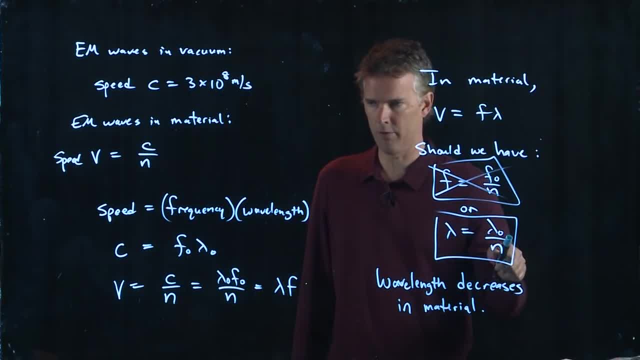 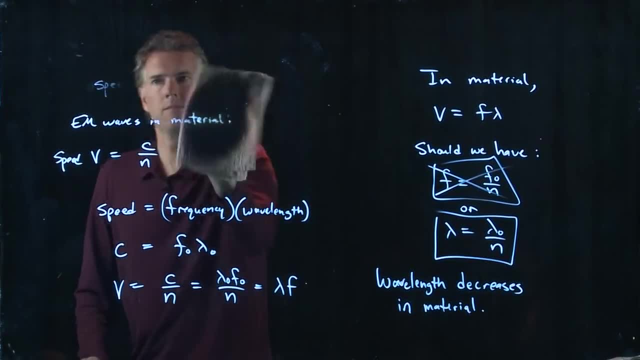 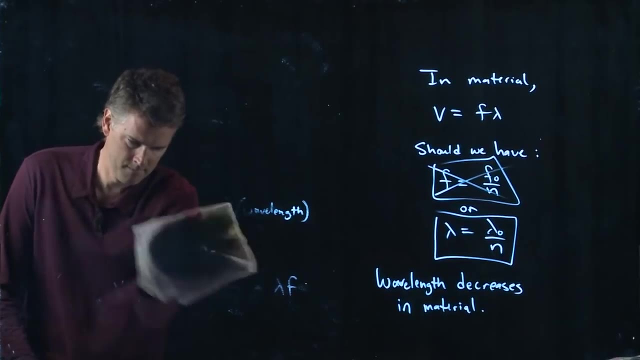 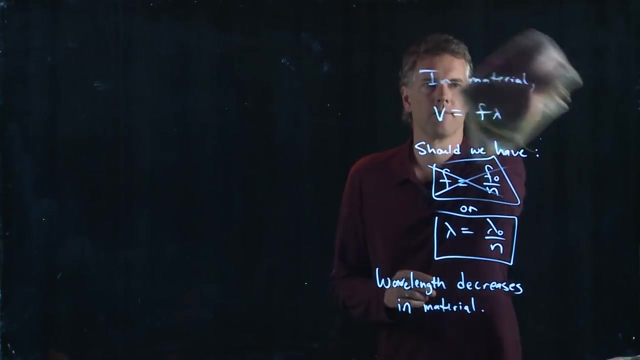 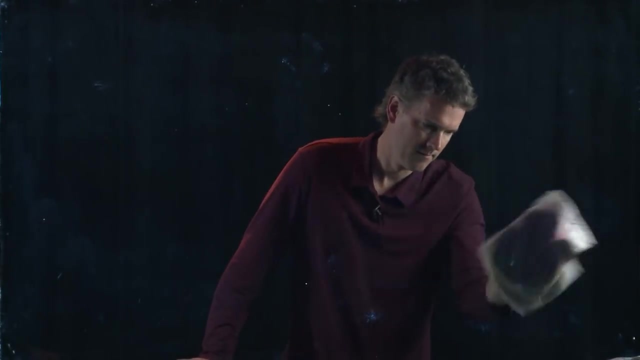 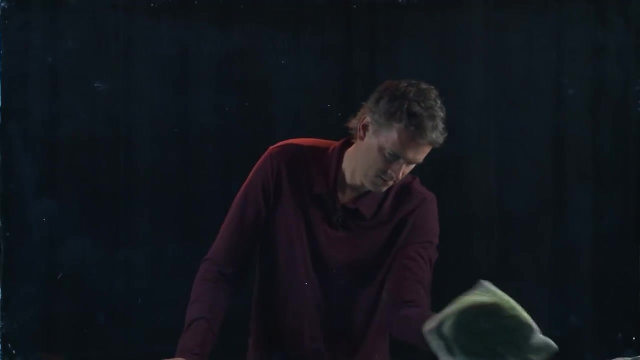 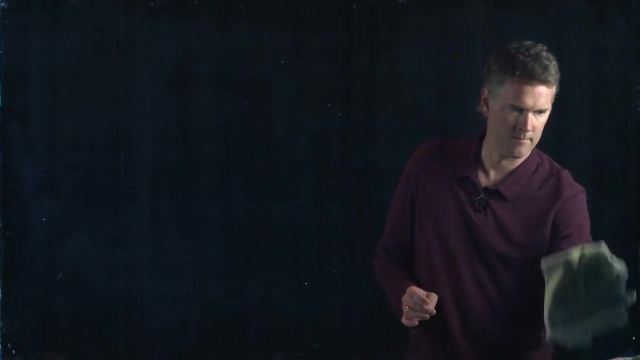 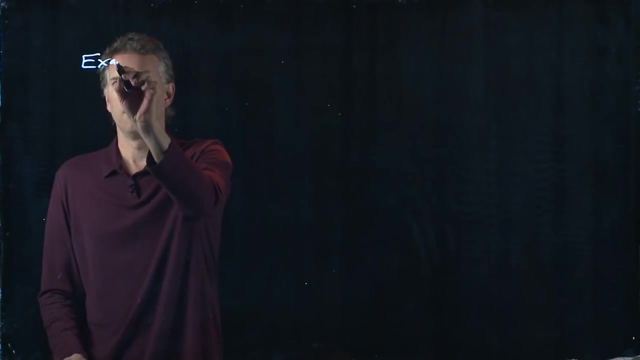 How much shorter It gets- shorter by the index of refraction. Thank you, Okay. so let's try an example of figuring out the wavelength and the frequency of a Heaney laser beam, And let's put that Heaney into water and let's ask the following questions. 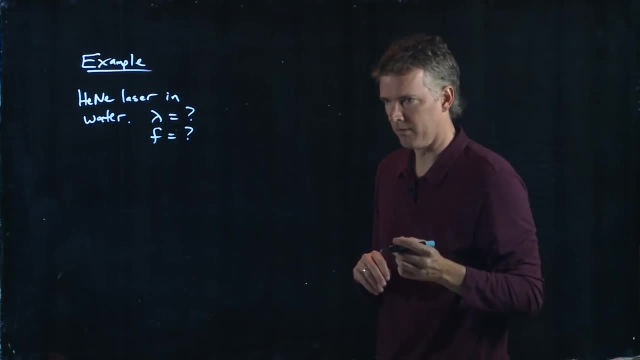 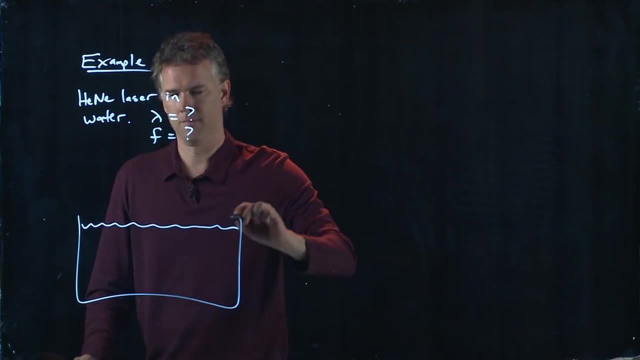 What's the wavelength of the Heaney? What's the frequency of the Heaney? Okay, so here's our tub of water. We're going to take our Heaney laser beam and we will shoot it into the water. You guys have been playing with Heaney laser beams. 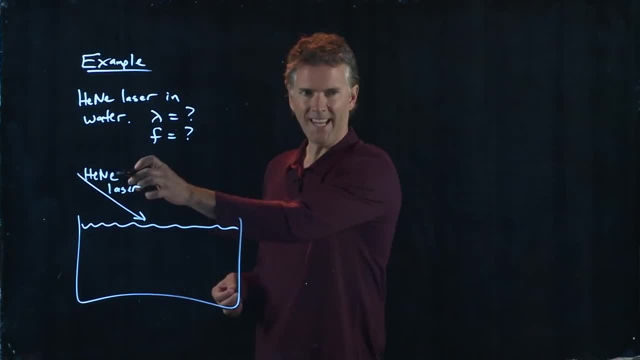 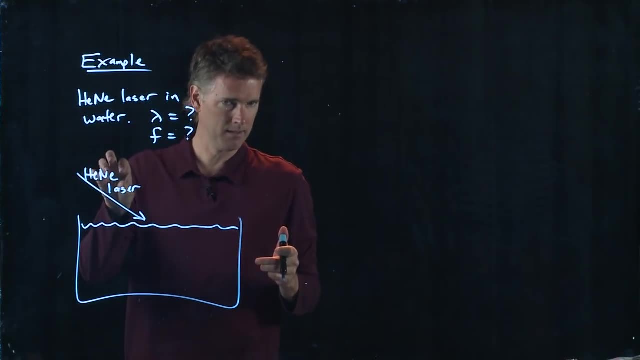 probably in your laboratories. Anybody know what He-nee stands for? He-nee is helium, neon. okay, These are the gases that are in your laser And it turns out the neon is really the important one for lasing. It's the atomic transfer. 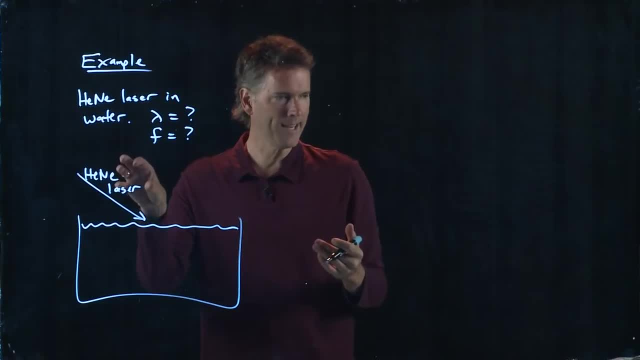 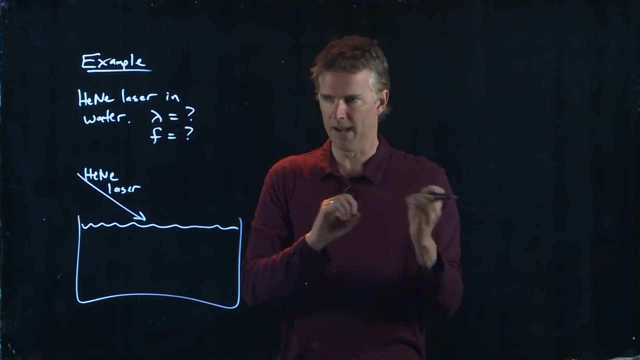 It's the transitions of neon that lead to the particular red color of the Heaney laser. The helium is actually there just to transfer energy. Okay, so the helium bounces around really fast, hits the neon, excites it, and then it can decay and emit light. 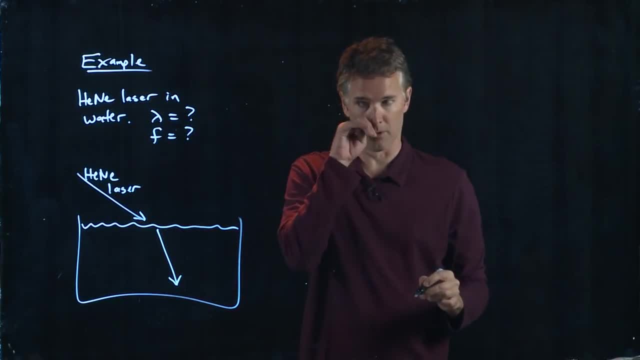 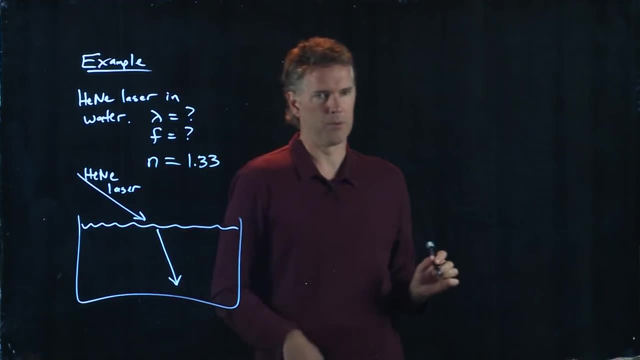 Okay, so we know what's going to happen. right, It goes in. it bends towards the normal a little bit. We know that the index of refraction of water is 1.33, right? And we also know that the Heaney laser has a free space frequency. 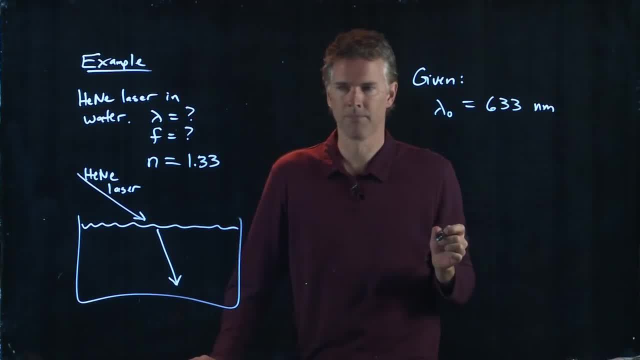 of around 633 nanometers. okay, Specifically it is 632.8.. So how do we calculate this stuff? Well, we know the following: C is lambda naught times F naught. We also know that V equals lambda times F, which is C over N. 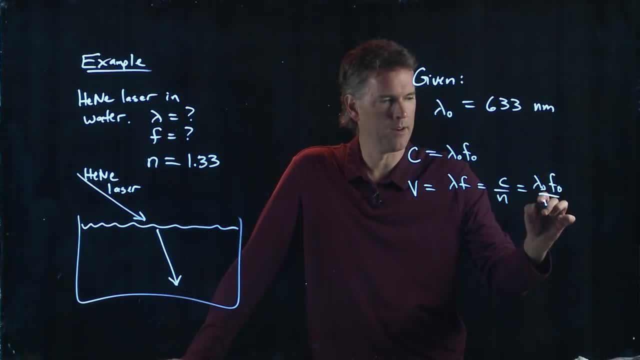 which is lambda naught F, naught over N, And so now we can use this information in this last statement to calculate lambda. like we said, lambda is the one that changes, It's just lambda naught over N, And we get 633,. 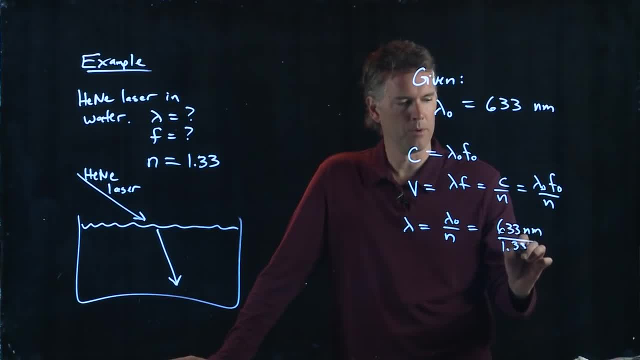 which is 1.33 nanometers divided by 1.33.. And if somebody has a calculator and wants to punch that in, tell me what you get. We can approximate it here. This is 633.. This is a 4, a 3 up in top. 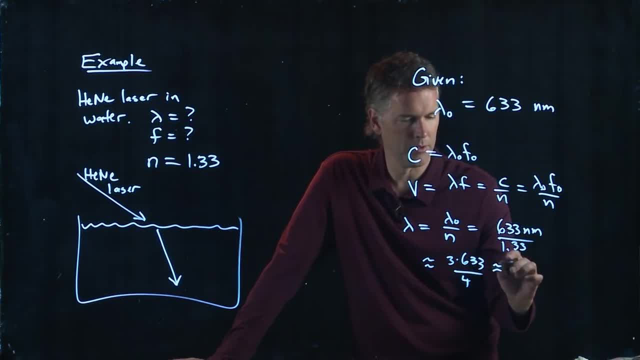 And so we're going to get: 3 times 633 is 1,899.. And we've got to divide that by 3.. So we're going to get: 3 times 633 is 1,899.. Divide that by 4,: 1,899 over 4, that's pretty close to 2,000. 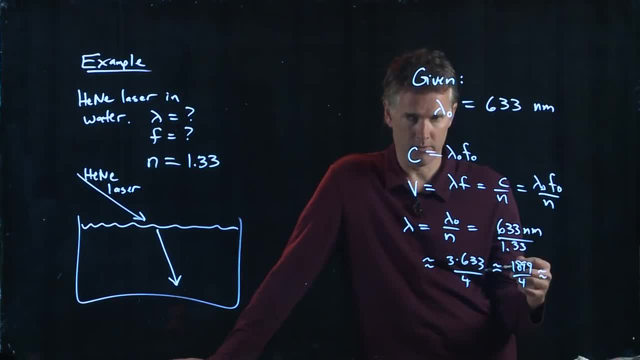 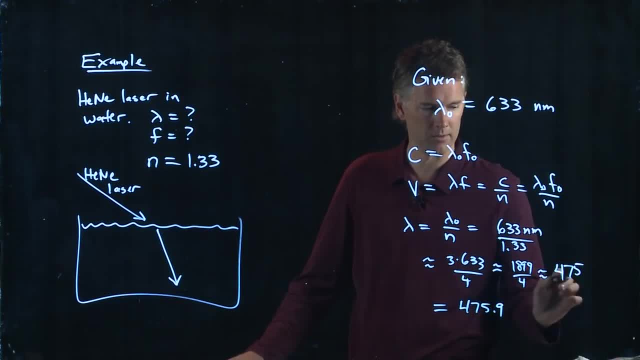 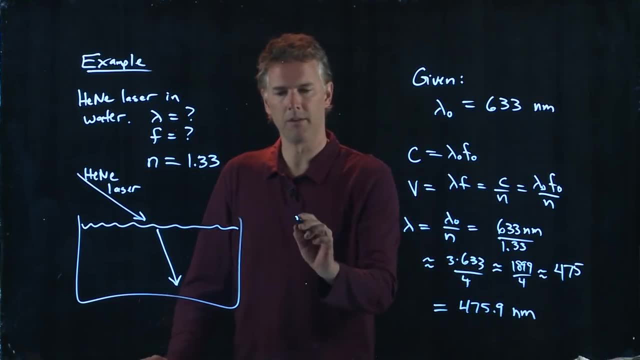 475.. 475.9, okay, so our guess, I'd say, was pretty good, 475.9 for the wavelength. what about the frequency? Well, the frequency doesn't change. The frequency is exactly the same in the material as it is out in free space, and so the frequency is just going. 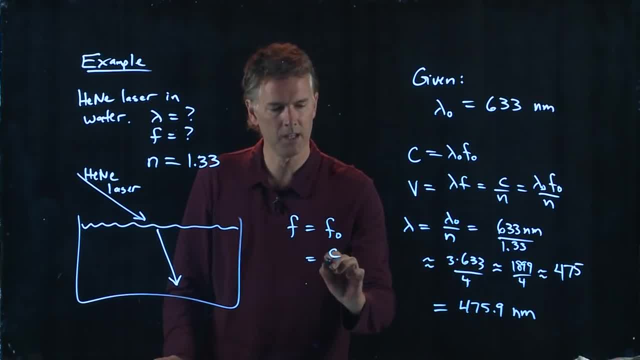 to be given by this equation. right here, It is C over lambda naught, and we know those numbers. C is 3 times 10 to the 8th. It is 638 meters per second. Lambda naught, we gave you 633 nanometers, okay, and now you've got to be a little bit. 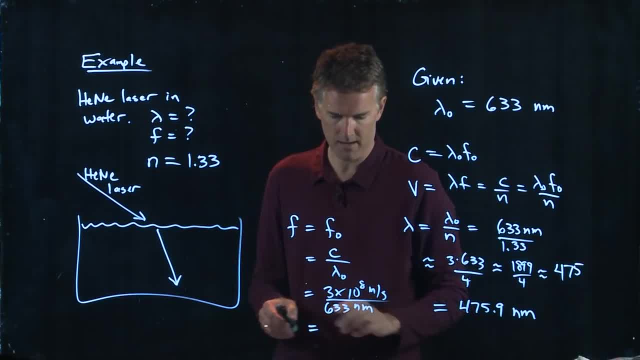 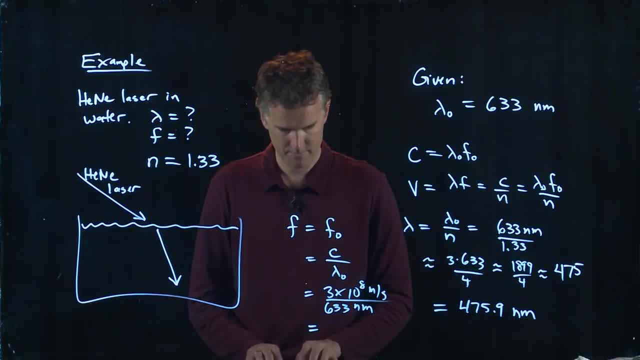 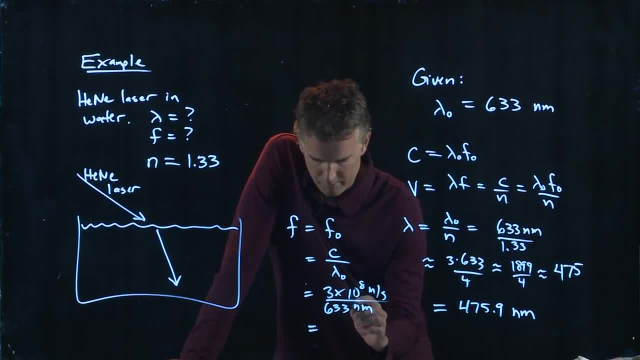 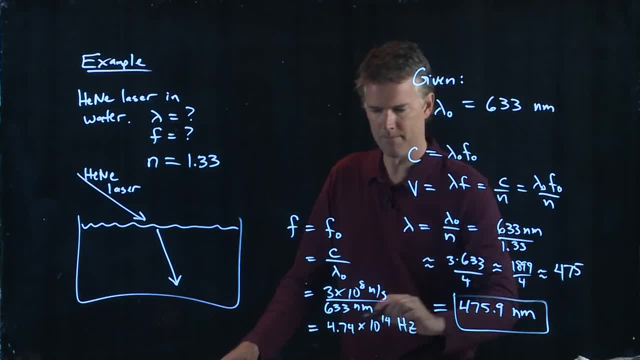 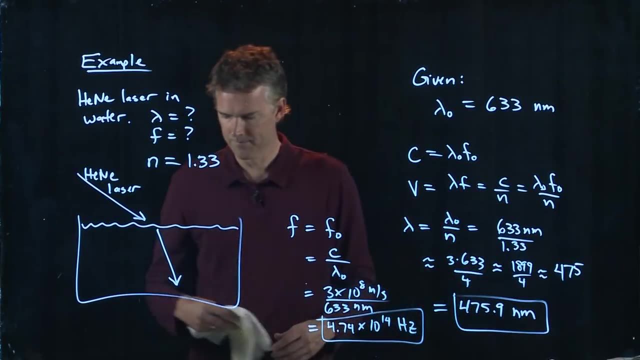 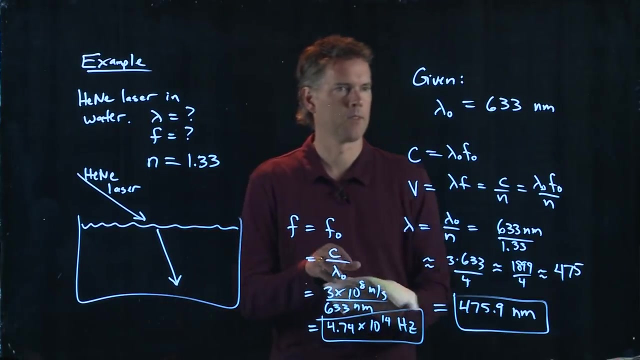 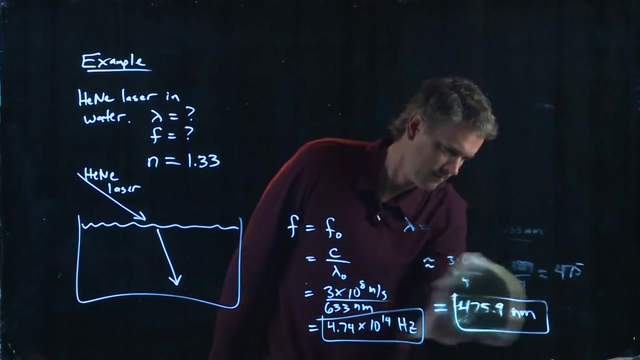 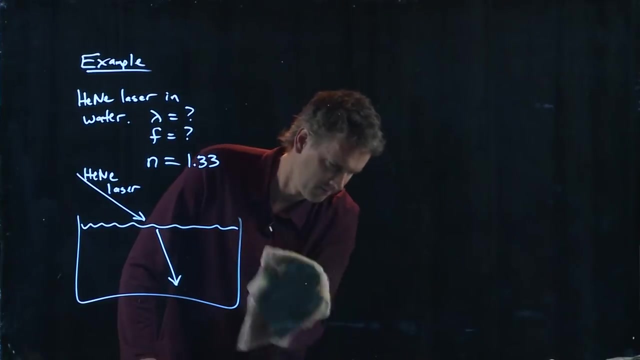 Is that what you guys got? when you punch it into your calculator, Anybody punch it in. Okay, Good, So that's how you calculate the frequency and the wavelength of electromagnetic waves in material. Okay, It's the wavelength that changes. frequency stays the same. 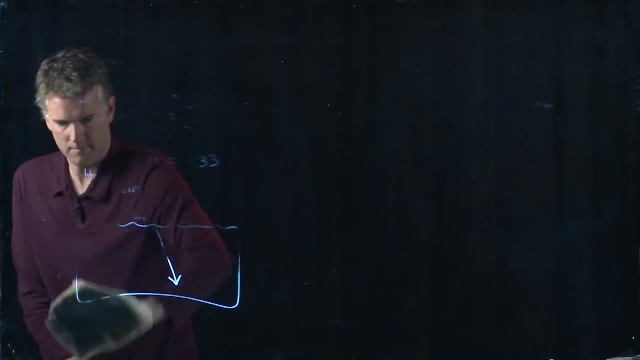 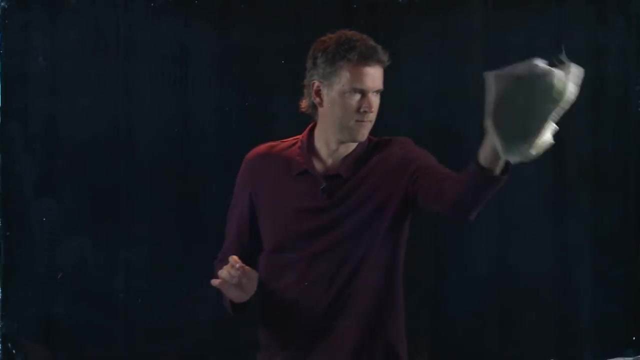 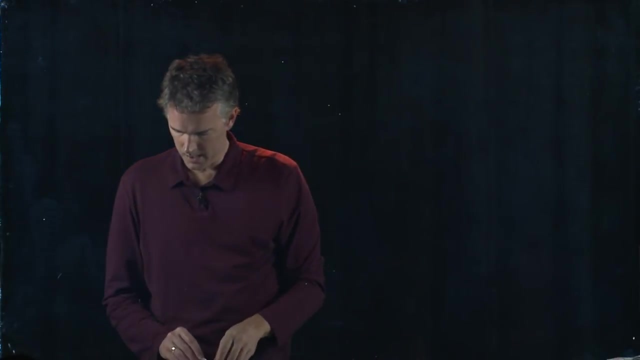 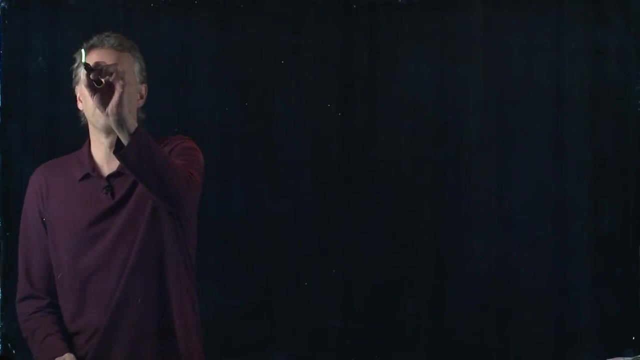 Okay, Okay, Okay, Good, Okay, Okay. why don't we- let's see, why don't we talk about just one more thing and then we're gonna break for today. So let's talk about thin films, and to understand thin films, we need to first understand this idea of 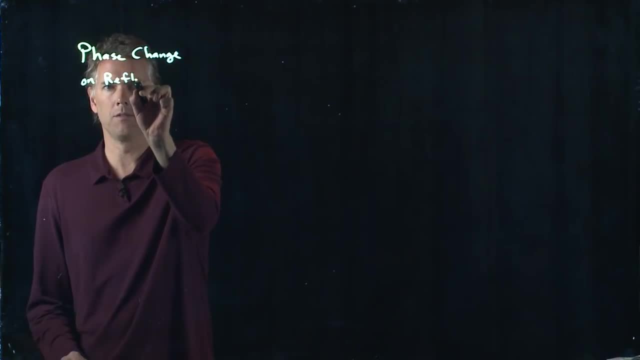 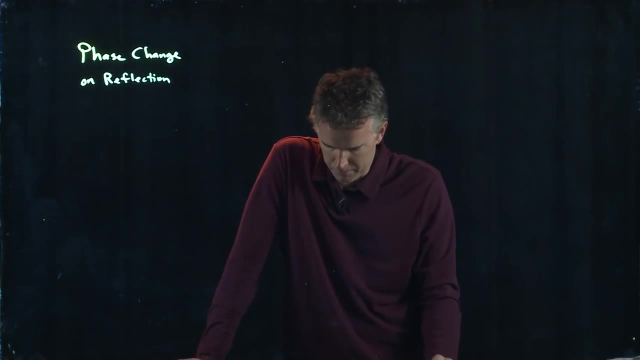 phase changes on reflection. so if we go back to this nice picture that they had on the textbook- Samuel, if you can pull up that screen again, can you guys see that over there? So they have a very nice picture there of a bubble- it's a soap bubble and what you. 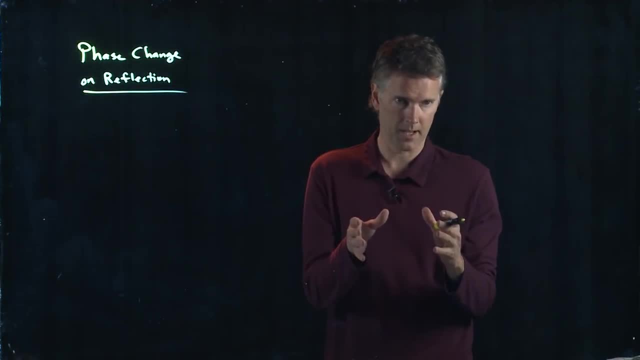 see in that picture is a bubble. So they have a very nice picture there of a bubble. it's a soap bubble, and what you see in that soap bubble is all sorts of different colors, and what we want to understand now is how do these different colors come about? right, 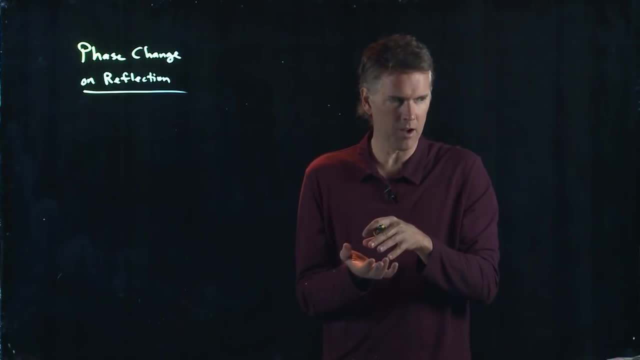 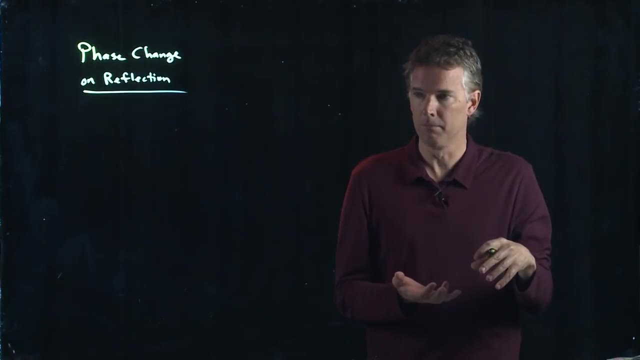 There's no dye or anything like that in the soap bubble itself. it's all the same material, and so you might think that sunlight coming in would bounce off all portions of the bubble exactly the same and it would just look white. to you it would look like sunlight, but there's 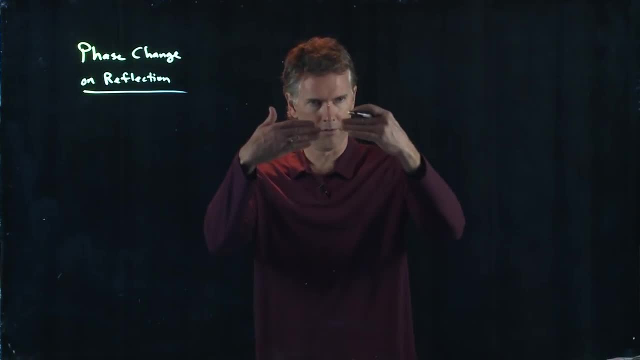 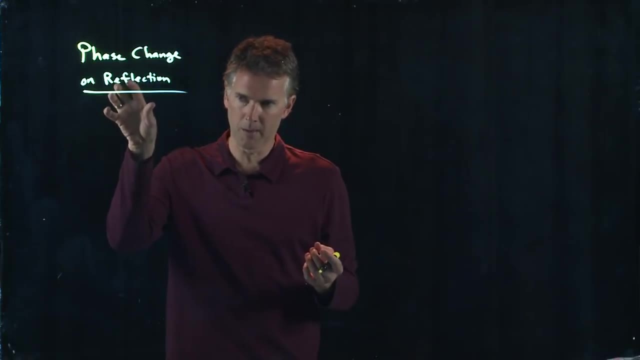 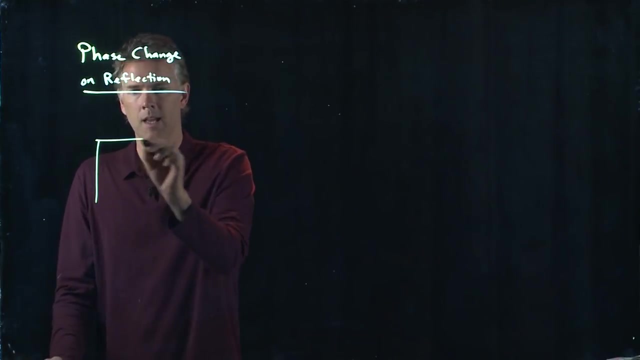 something very different that happens on the top part of the bubble versus the sides, versus the bottom part of the bubble, and to understand that we need to understand thin films and specifically, we have to understand this phase change on reflection. so let's see if we can make some sense of this. 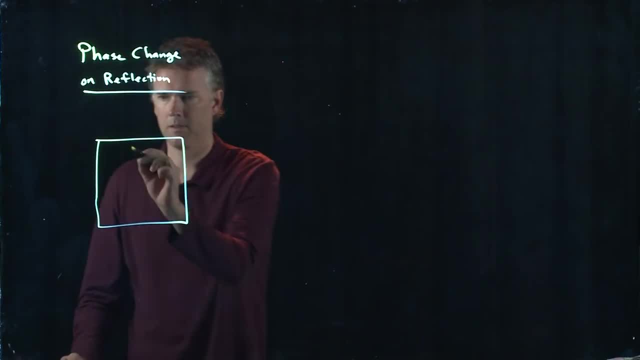 Let's say I take a big piece of glass and I send an incident laser beam towards the edge of the glass. okay, I'm inside the glass already it's going to fire towards this end. okay. Okay, I'm inside the glass already it's going to fire towards this end. okay. 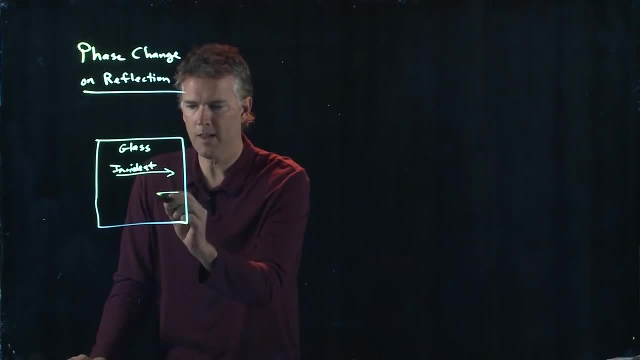 Okay, I'm inside the glass already. it's going to fire towards this end, okay, And this glass is flying down the edge of the glass. There is going to be a reflection here off the glass and this was air, and so we are going. 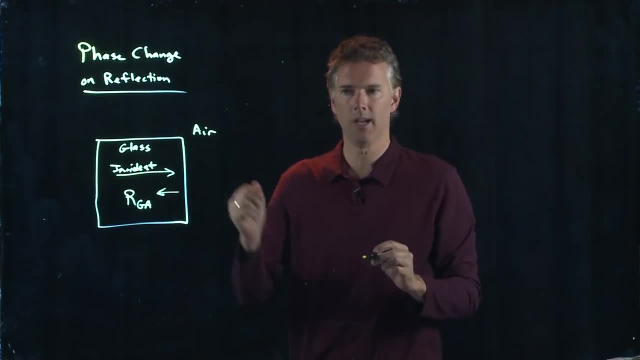 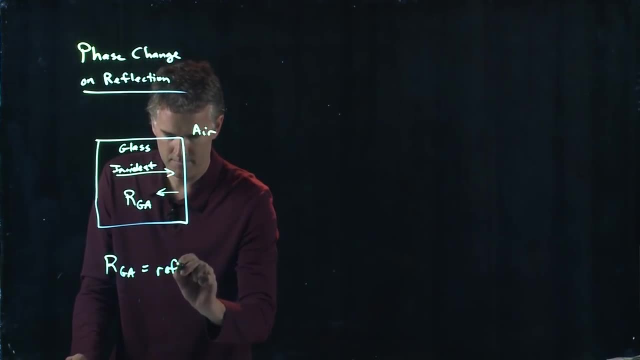 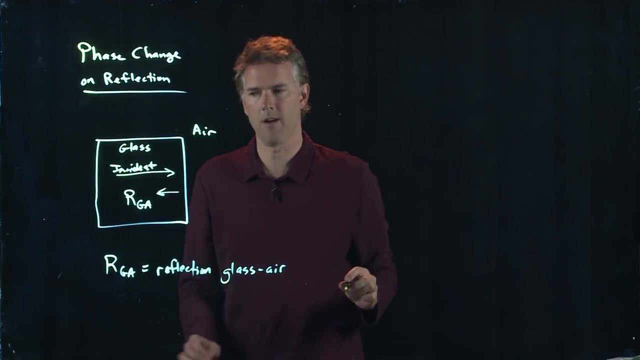 to call this reflection- reflection from glass air interface RGA- The reflection that happens when you are trying to go from glass to air to air. Okay, but we know that some of that light is going to keep propagating right on through, so let's put a second chunk of glass right here and there is some light that keeps. 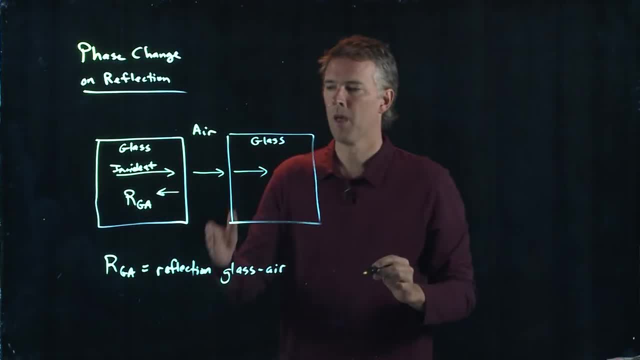 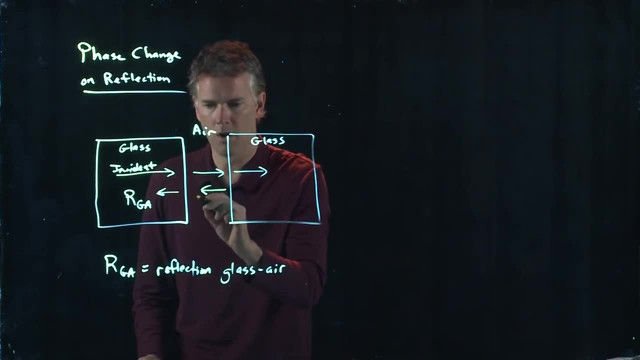 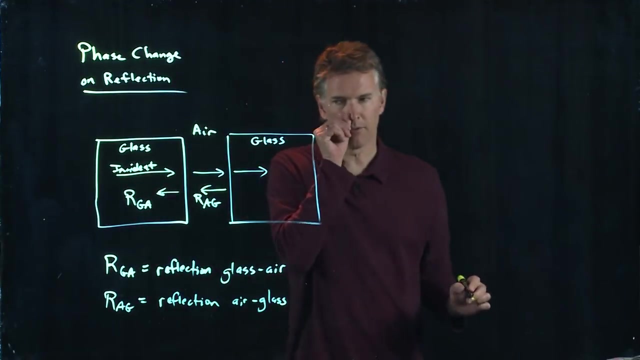 going through and there is some more light that keeps going through, but when this light hits this interface, it reflects again, And so there is r sub a g, which is reflection from air to glass. Okay, so on one of these, you were in glass, you're going to air, You're in a dense medium. 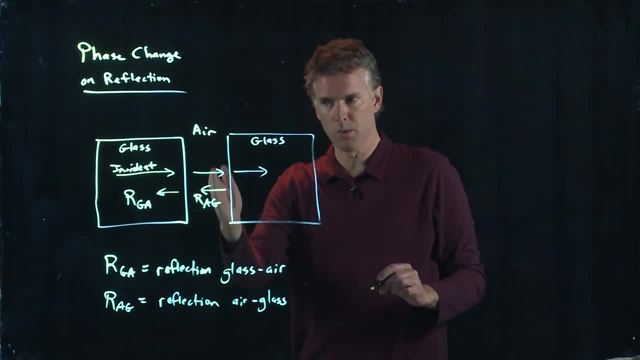 going to a lighter medium, but in the other one you were in air, going to glass, and so that's a reflection from air to glass. So that's a reflection from air to glass. So that's a reflection from air to glass. 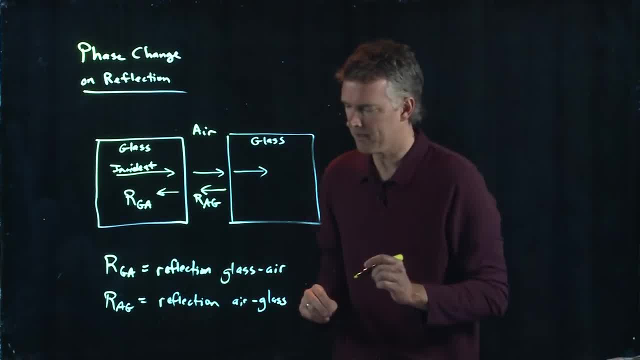 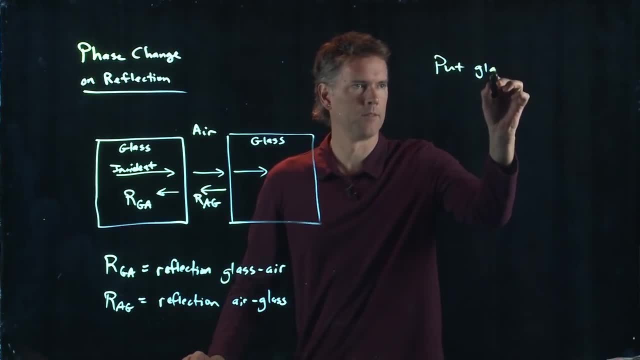 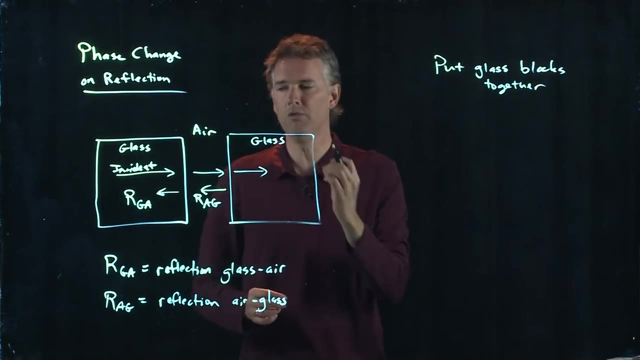 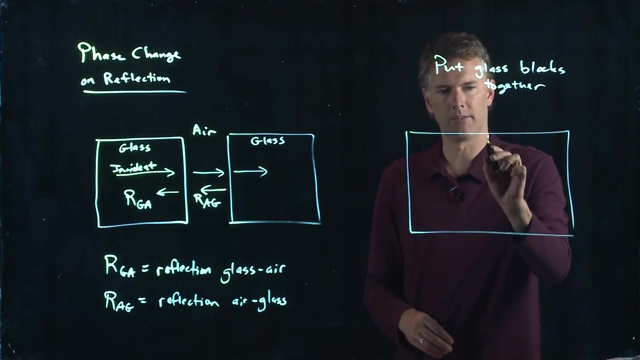 reflection from a light medium going to a dense medium. But let's put these glass blocks together. Okay, if we fuse them together, then it should just be one big block of glass and that interface should go away. Okay, we're going to push them together. 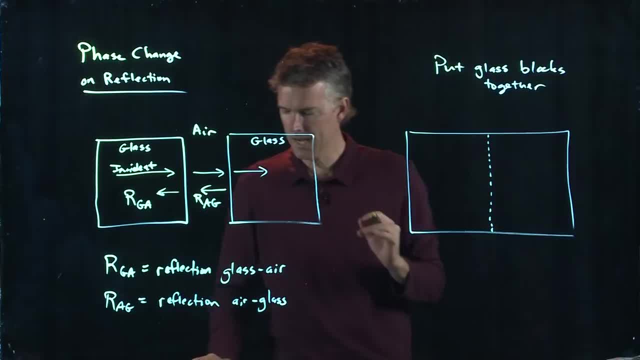 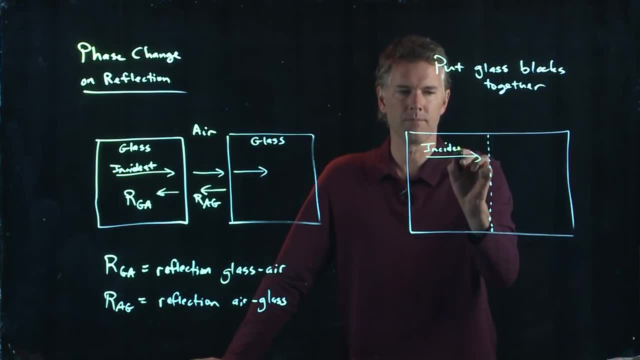 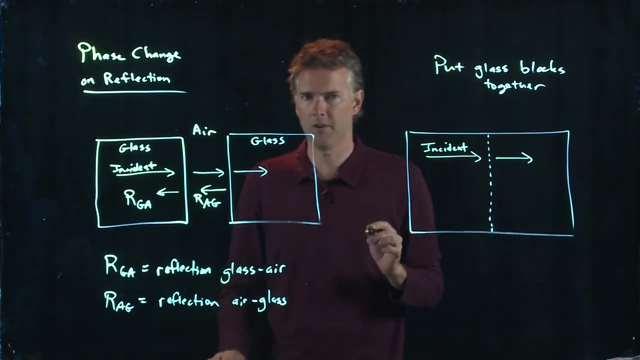 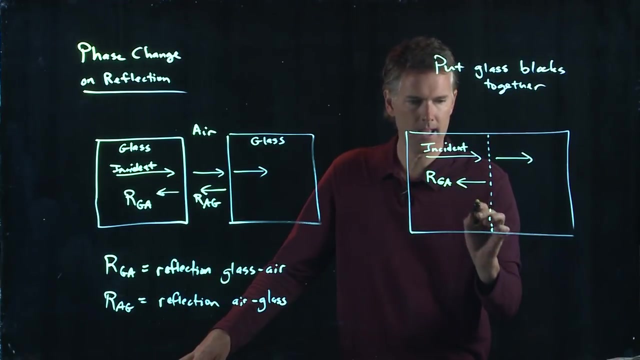 melt them a little bit, really have them stick together, and now there's essentially no interface. So any light that's coming in towards that hypothetical interface is going to keep going without being disturbed And in fact, any reflection here. RGA and RAG are going to be right on. 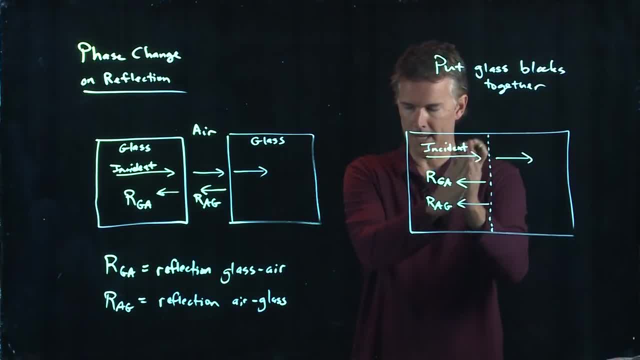 top of each other- Okay, because the interfaces are right on top of each other now, But there is no reflection. When you send light through a piece of glass, it just keeps going through the glass. It doesn't suddenly bounce back halfway through the glass. 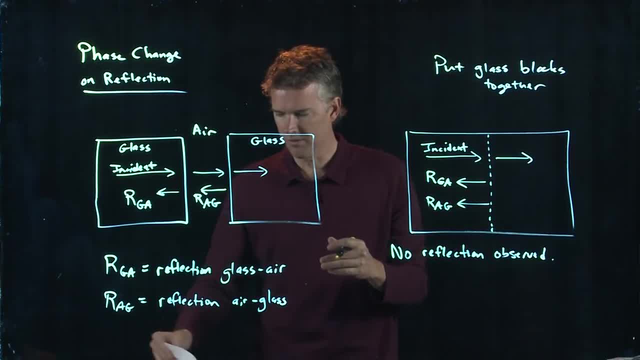 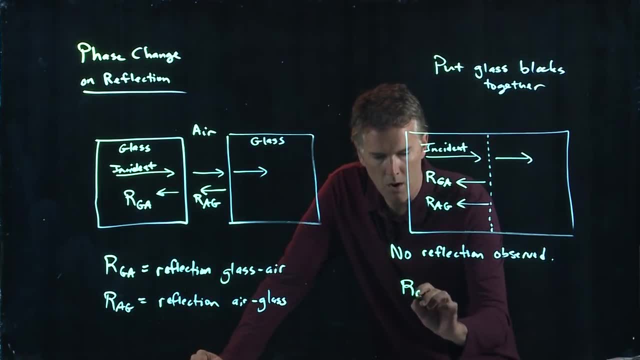 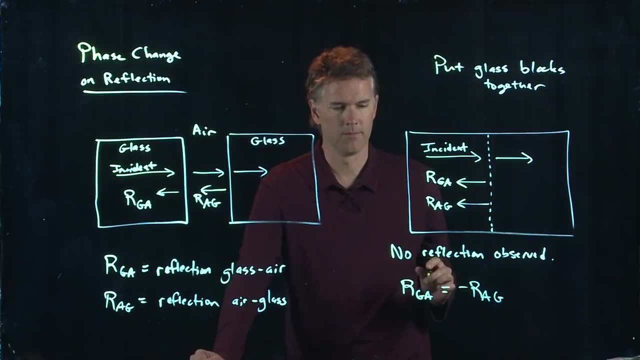 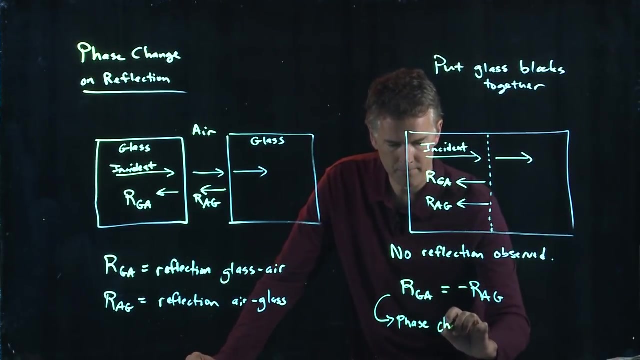 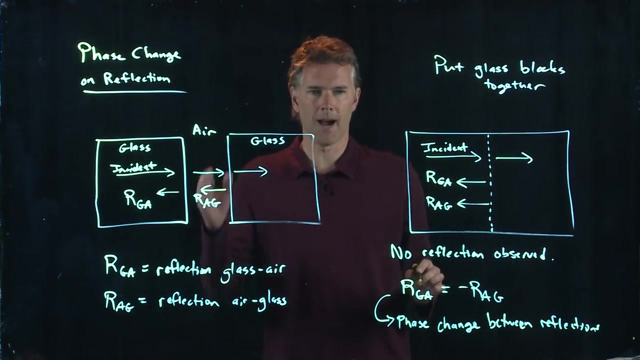 Okay, it just continues onward. So there's something very critical: that what we can say about the reflection RGA is in fact equal to negative RAG and this means that there is a phase change between those two reflected beams. Okay, when you go from high density to low density material versus low density to high density, there is a phase change. 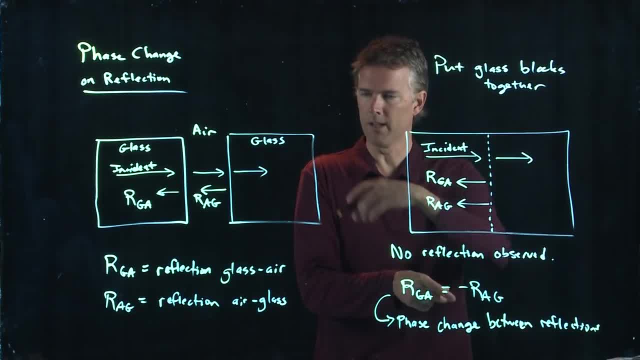 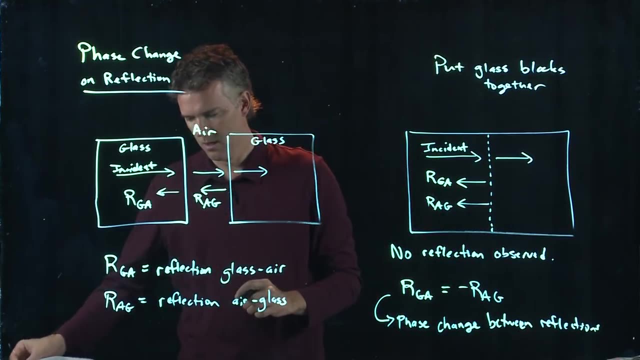 There is a 180 degree flip of your field. Any field that was a cosine becomes a negative cosine, And that way, when you add these up, you're going to get zero. You will, in fact, get zero reflection. All right, Let's see if we can spell that out with regards to these thin films and these soap bubbles. 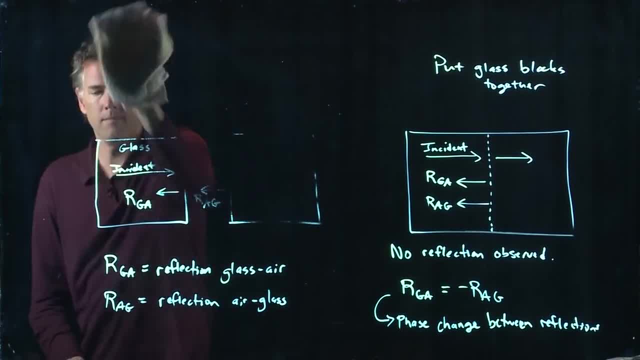 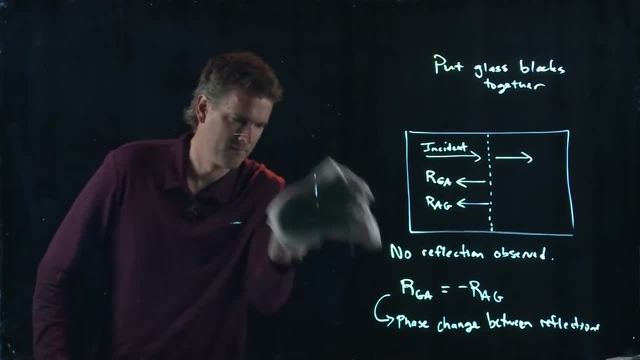 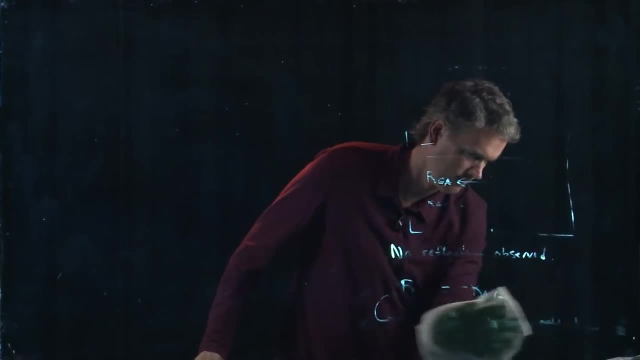 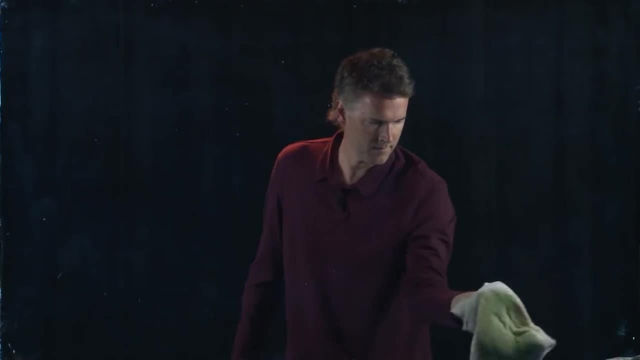 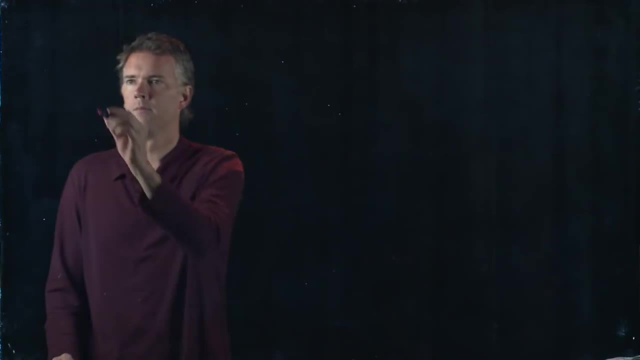 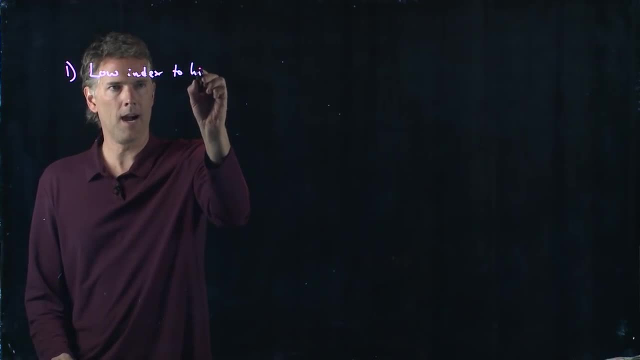 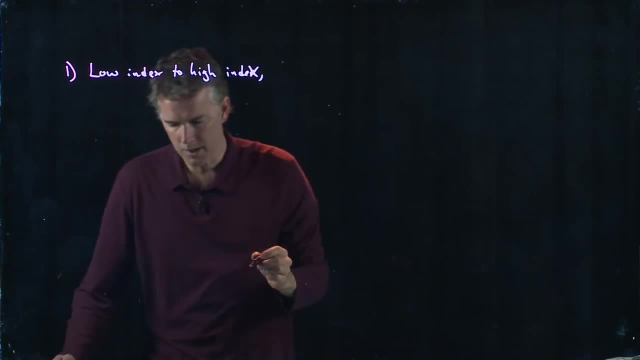 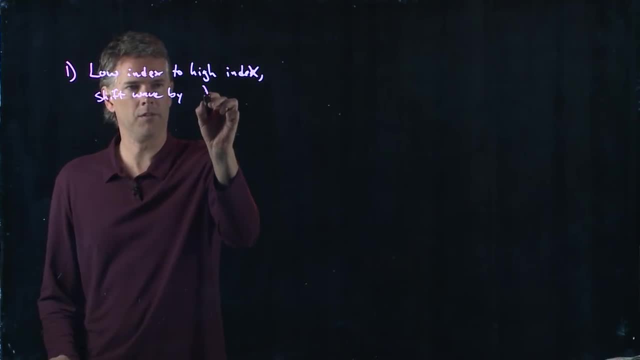 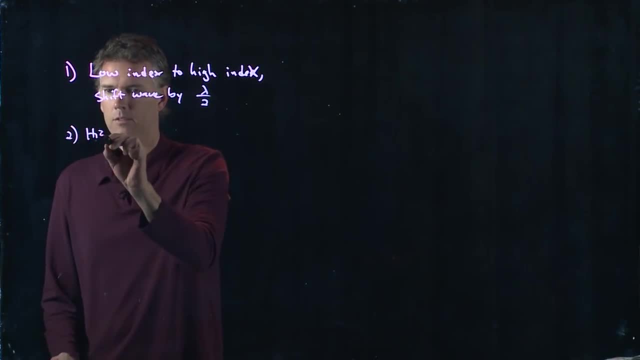 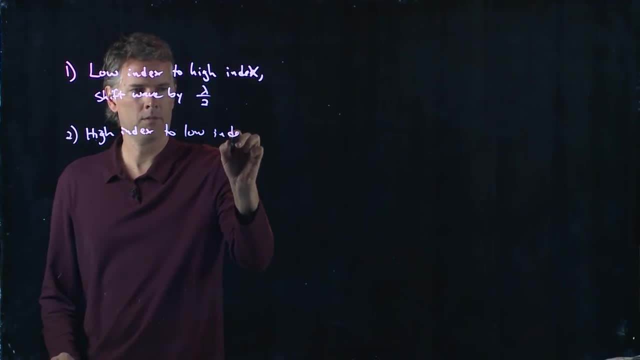 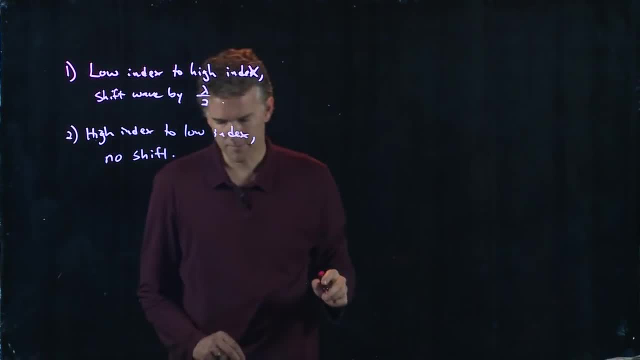 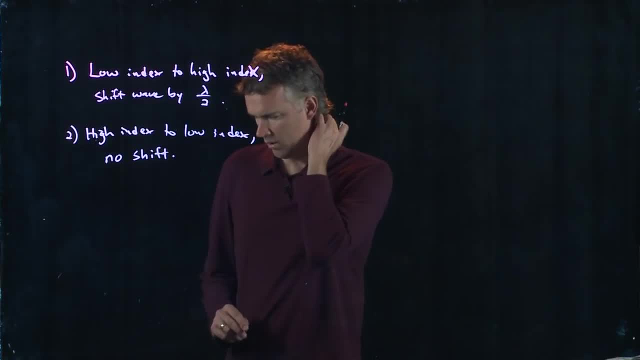 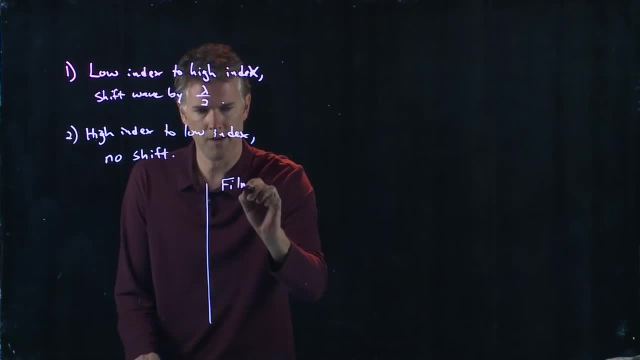 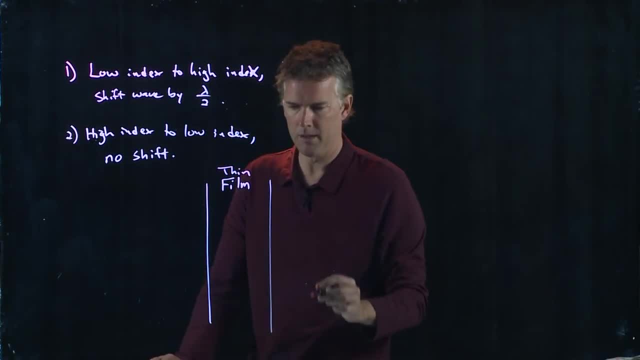 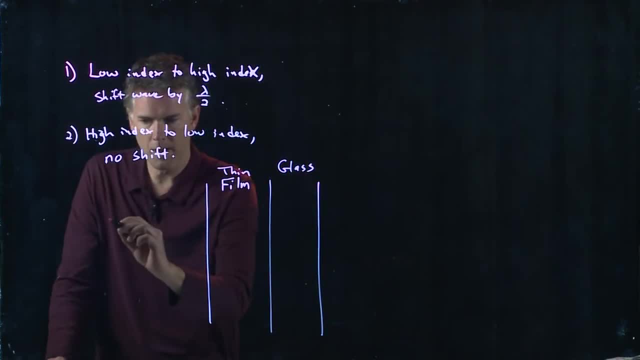 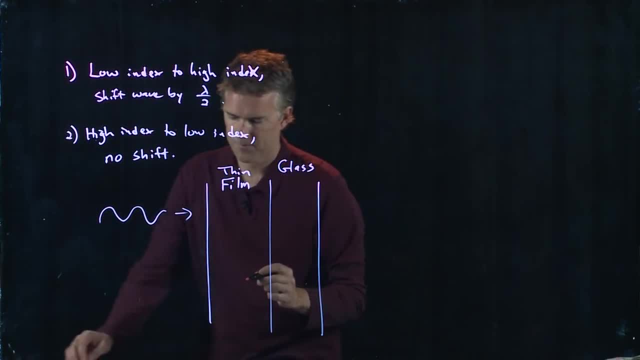 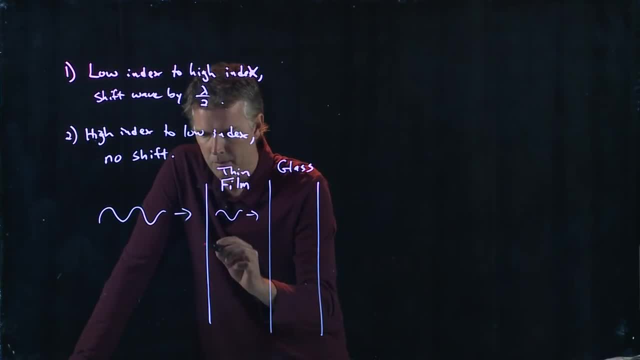 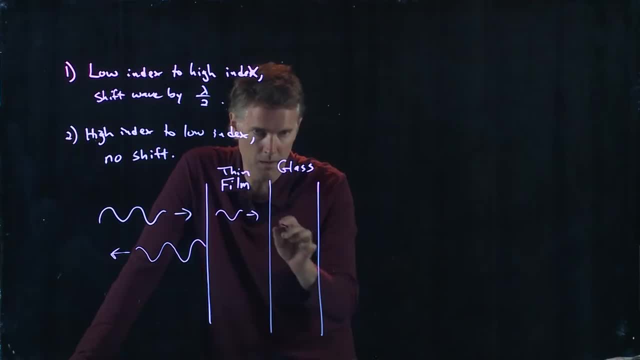 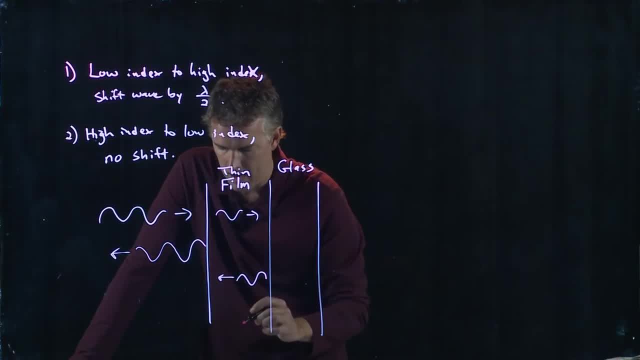 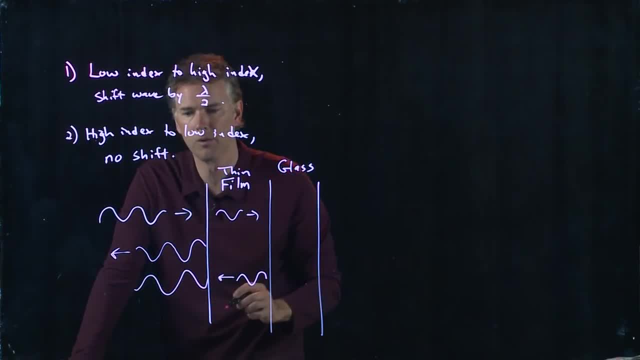 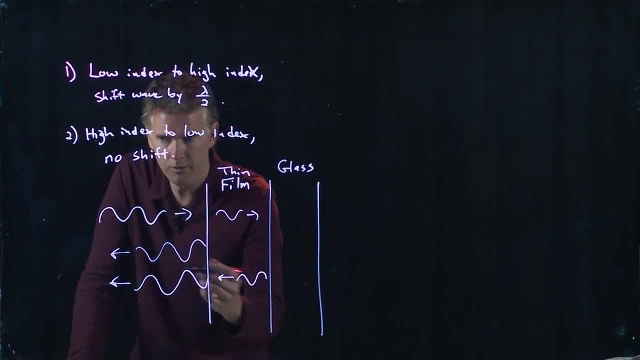 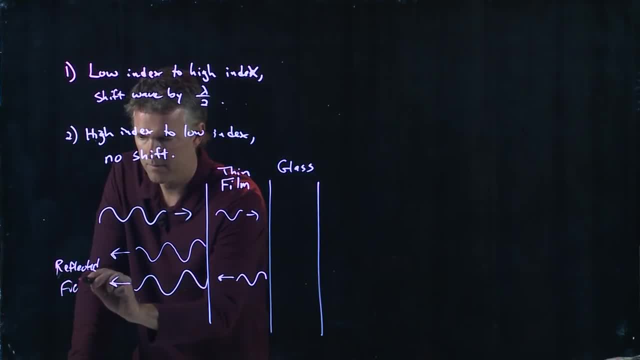 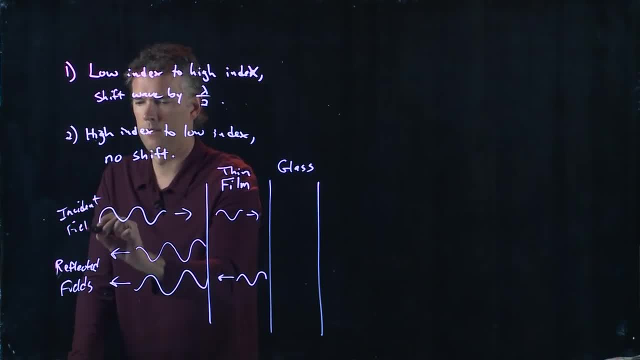 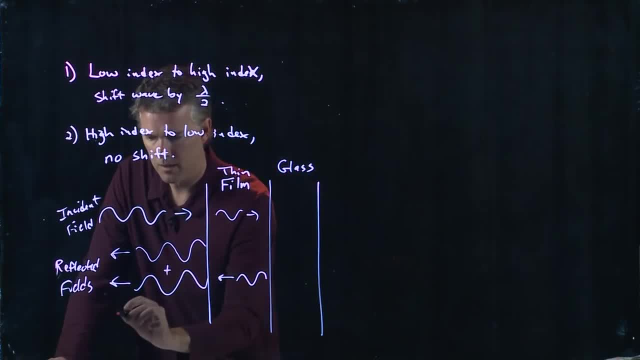 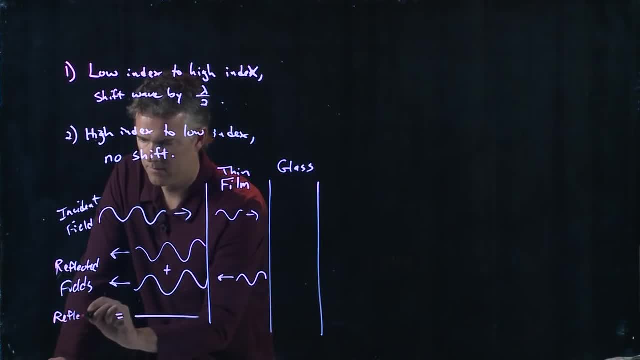 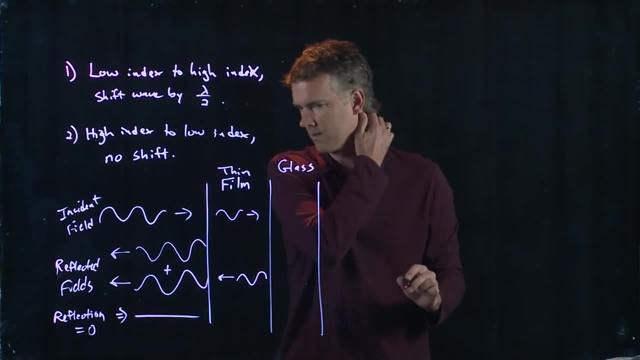 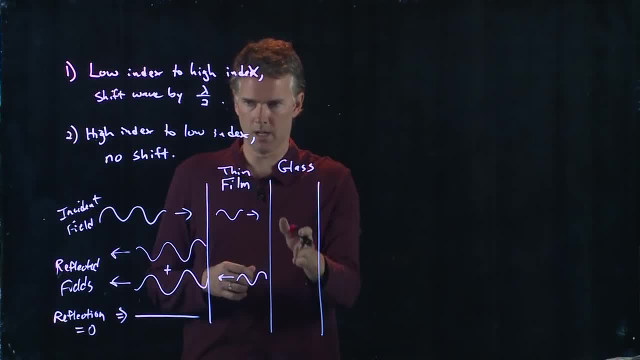 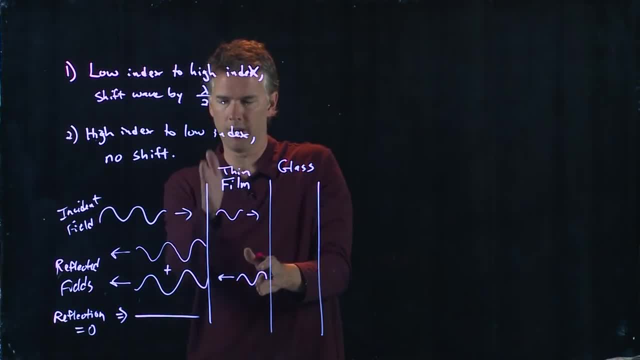 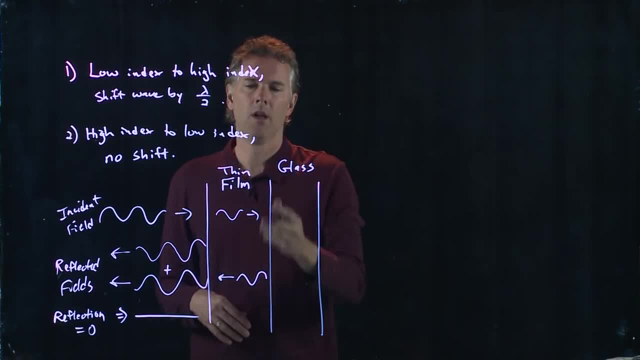 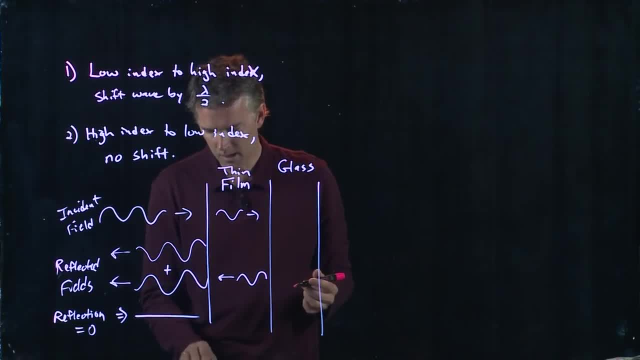 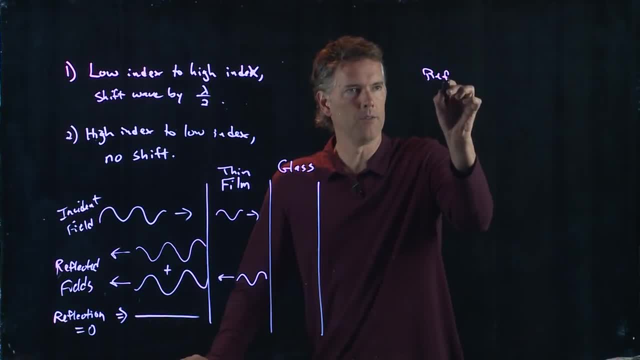 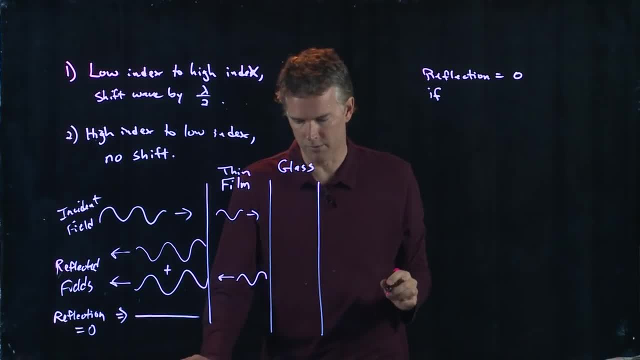 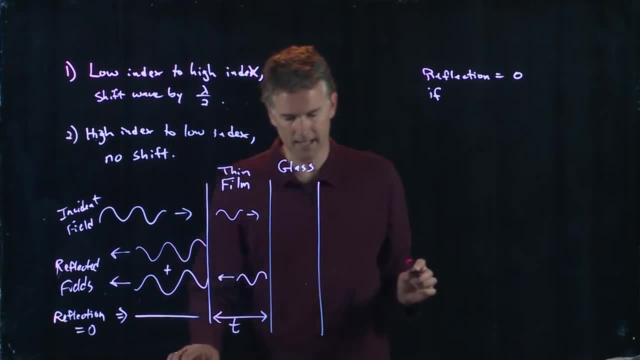 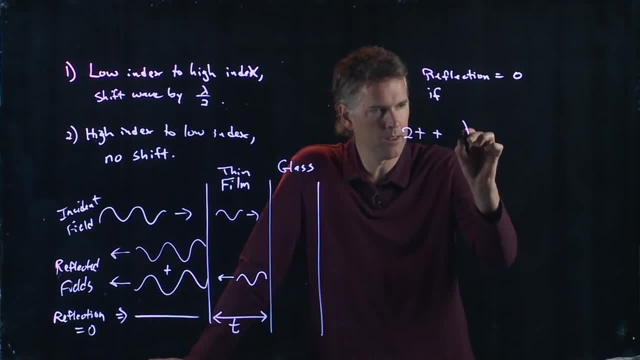 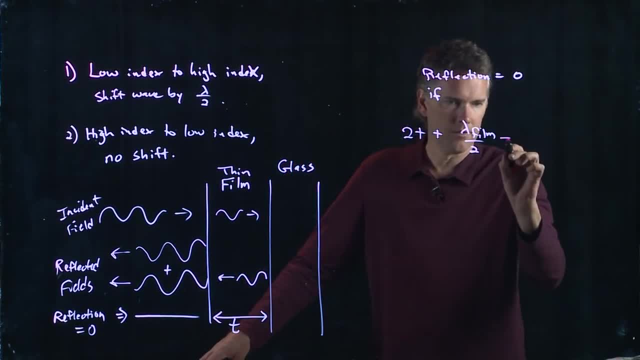 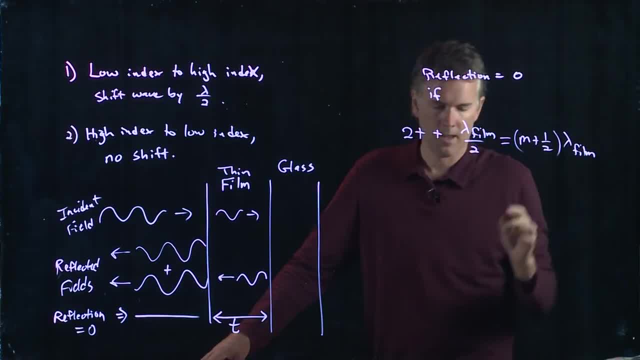 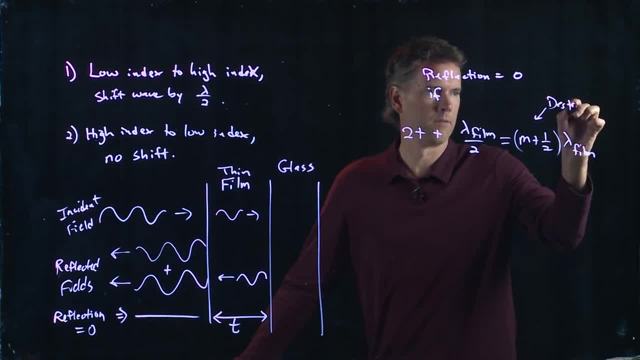 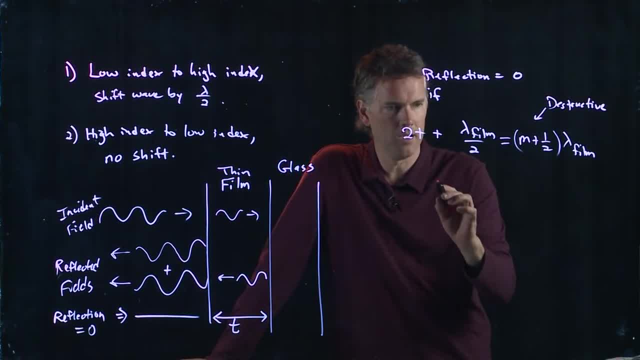 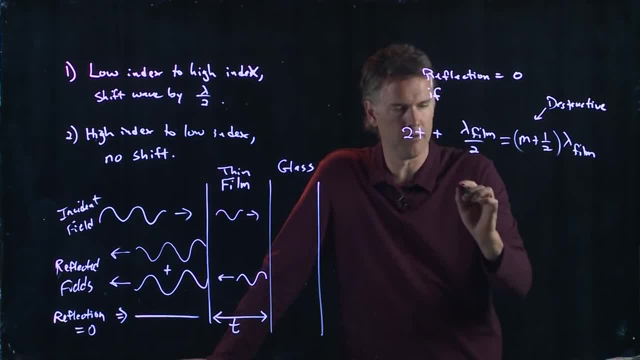 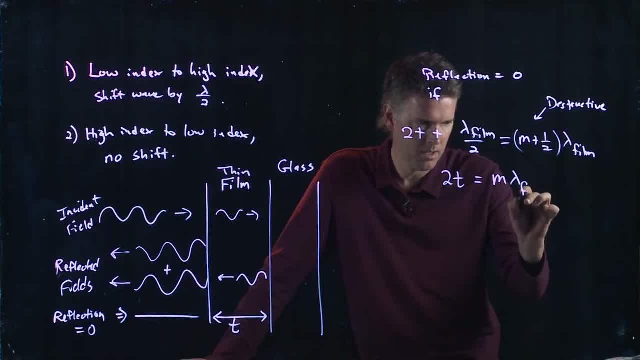 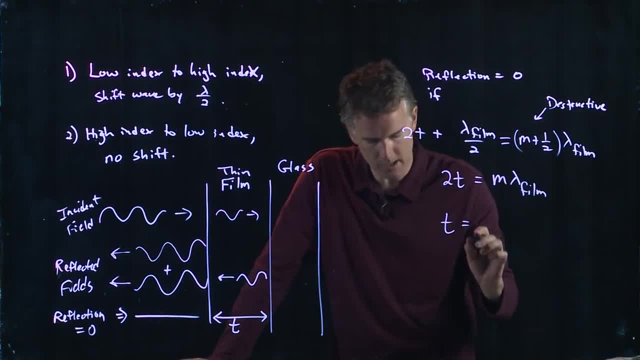 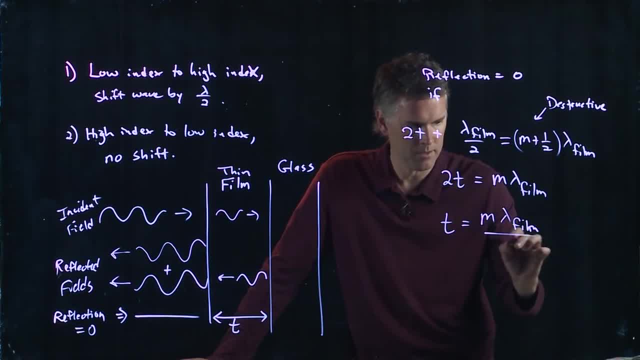 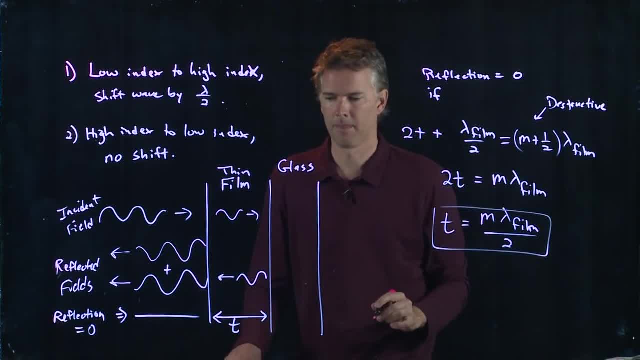 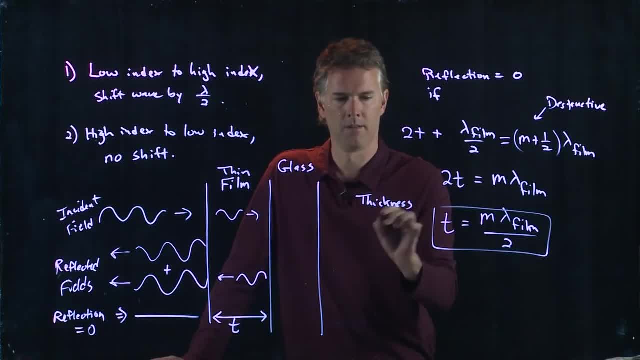 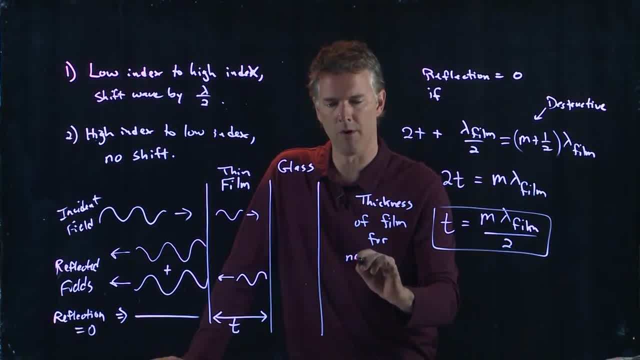 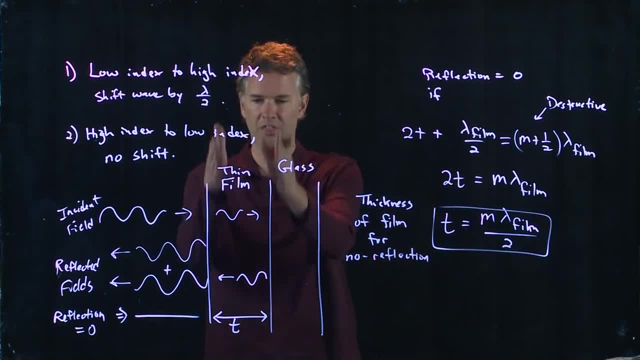 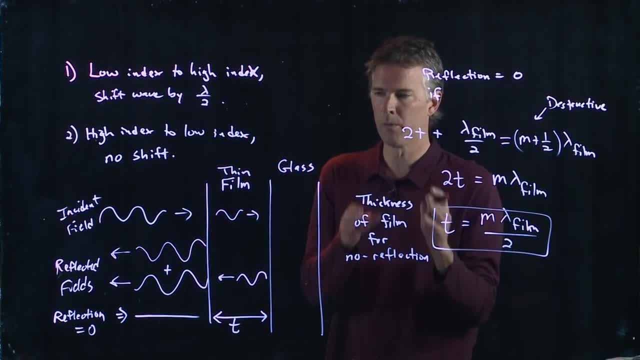 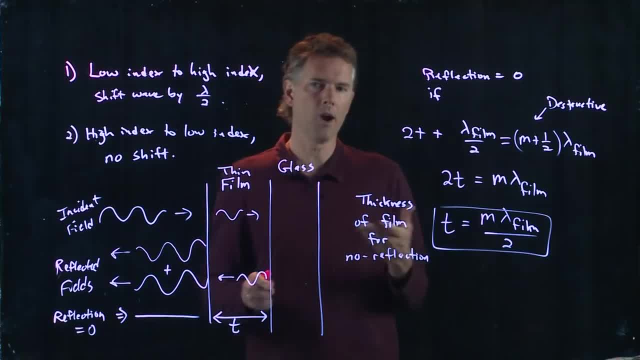 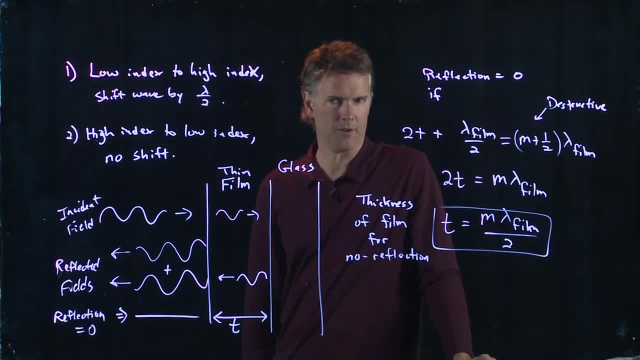 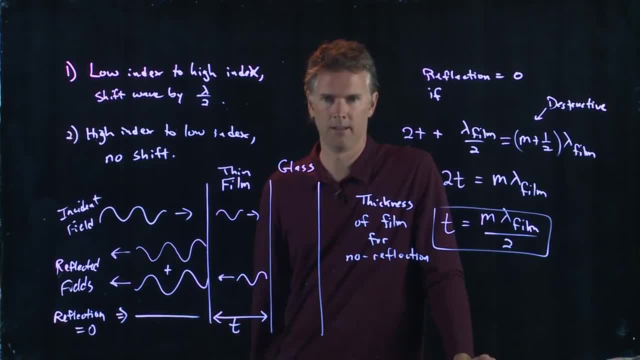 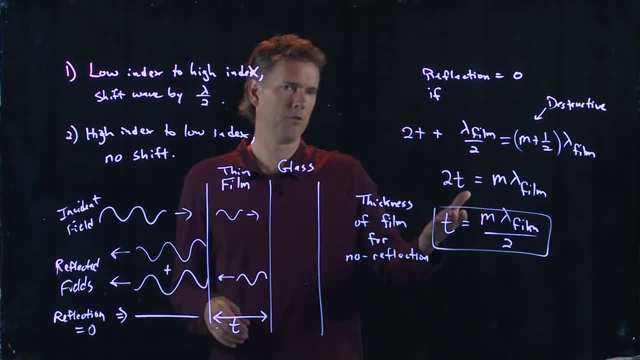 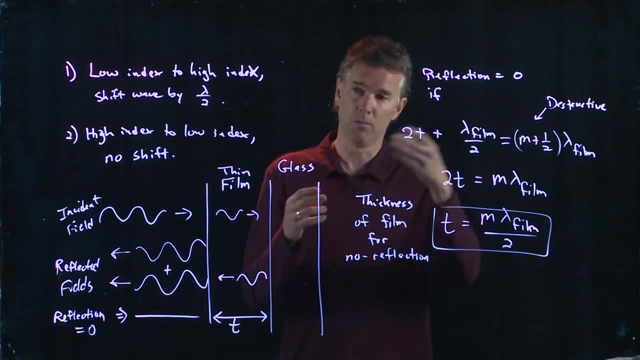 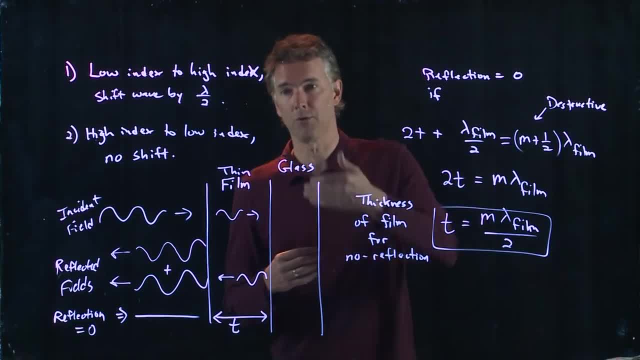 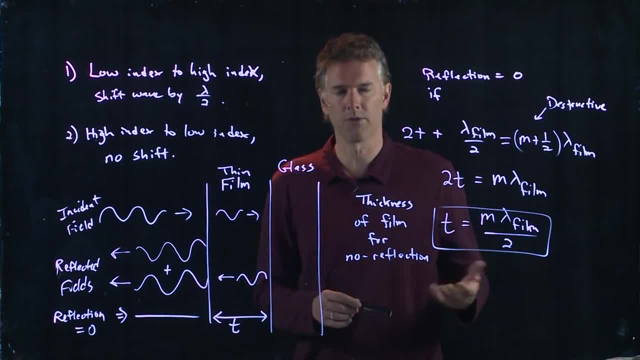 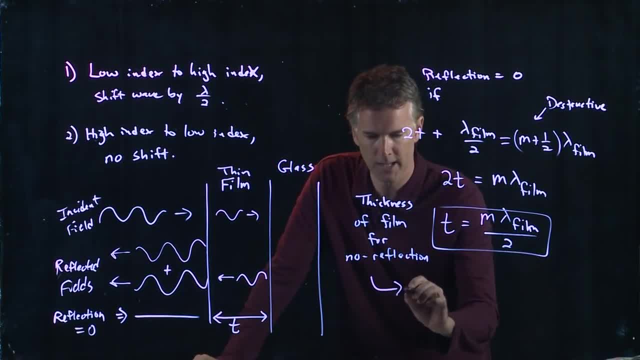 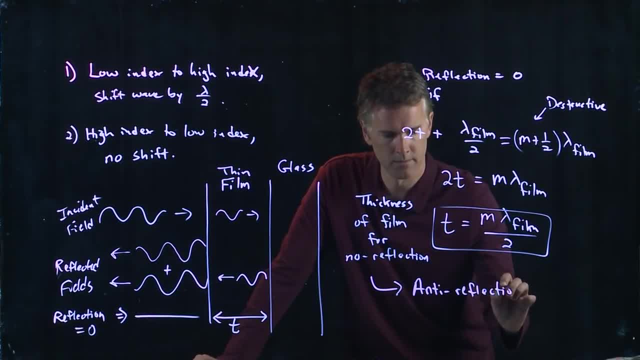 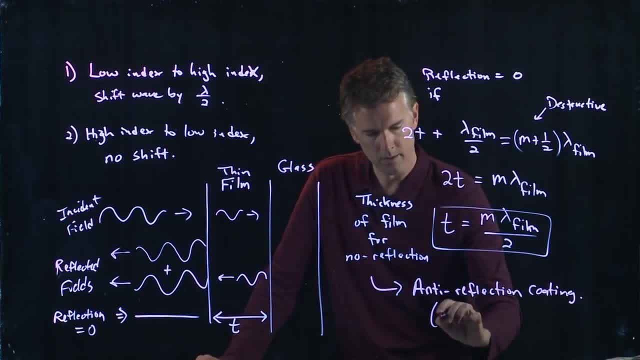 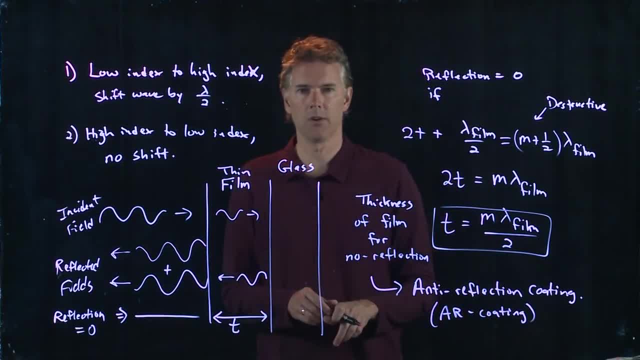 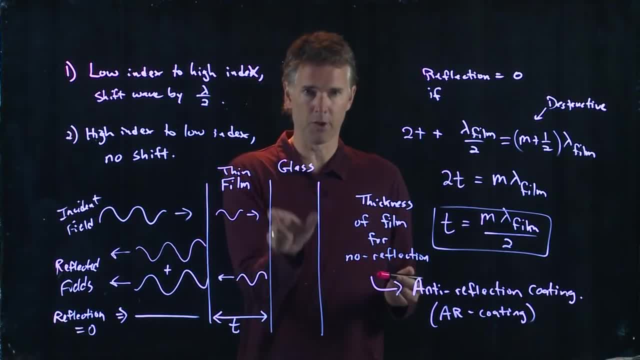 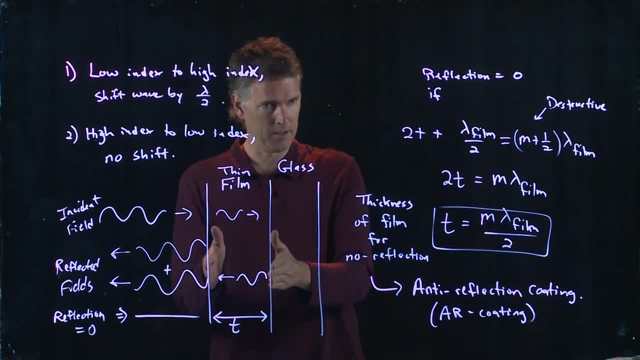 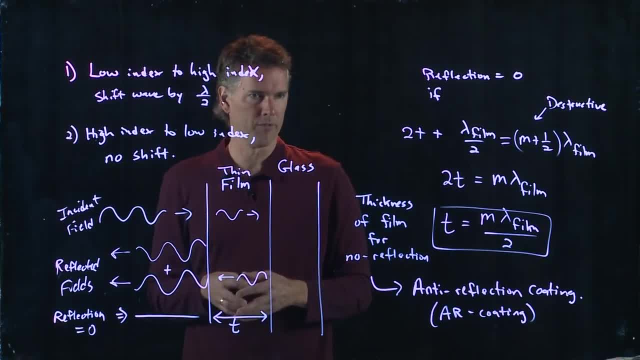 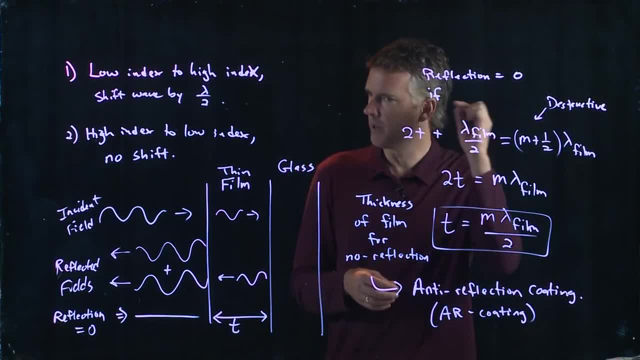 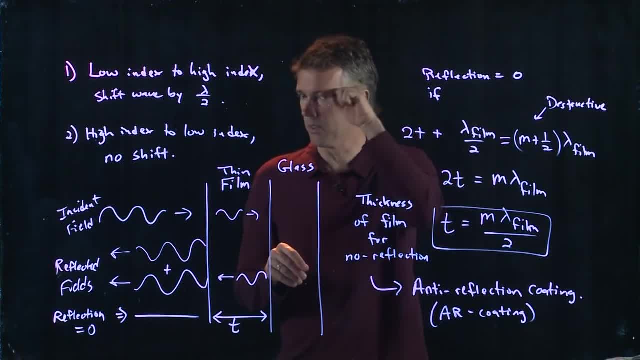 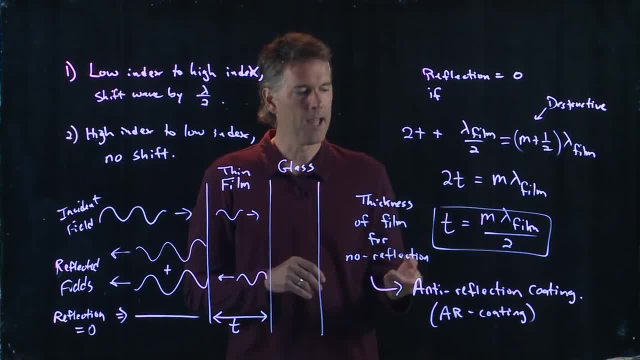 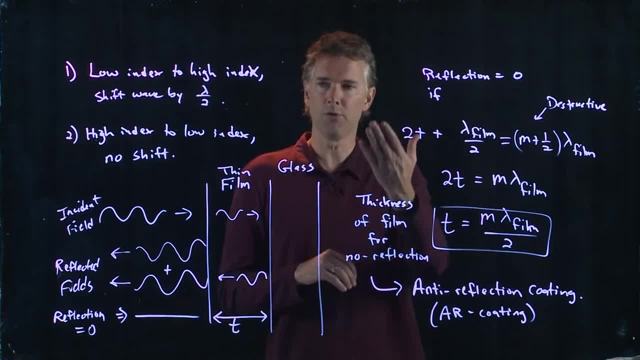 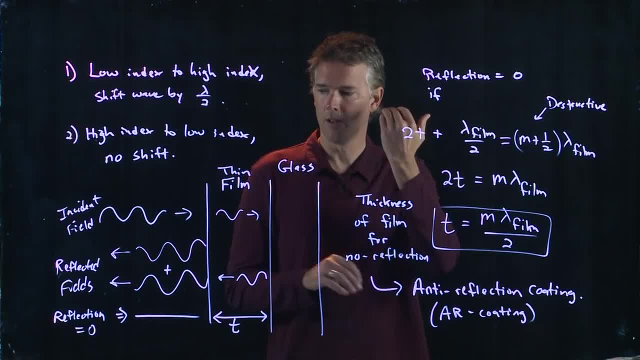 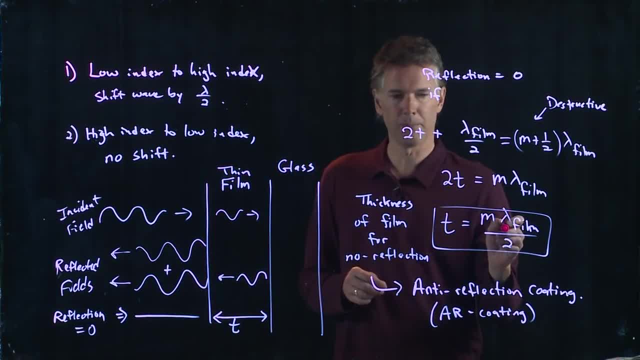 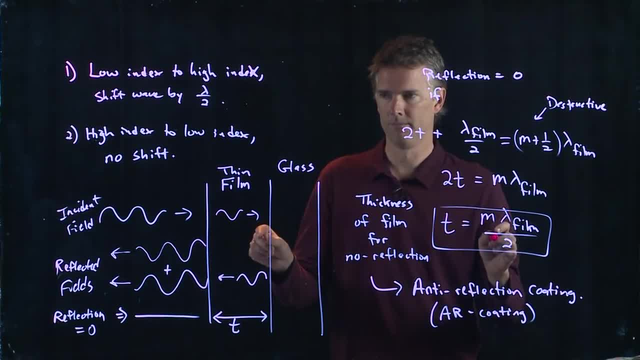 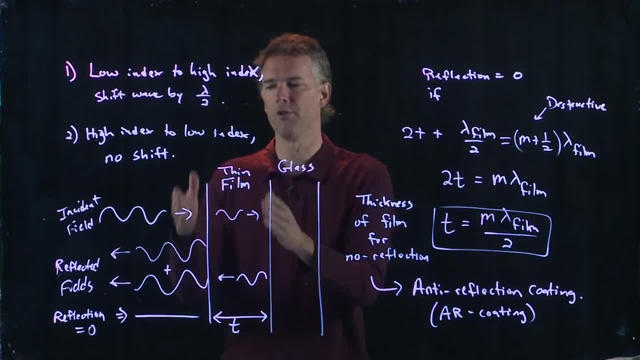 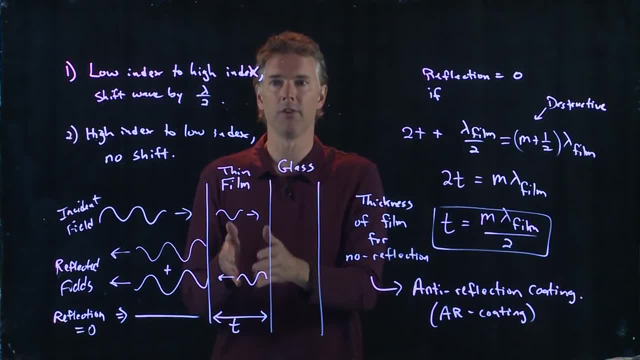 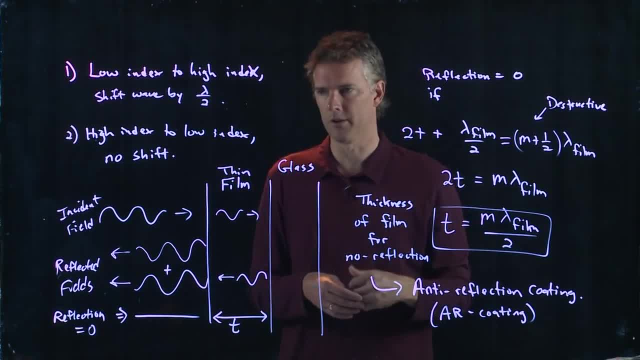 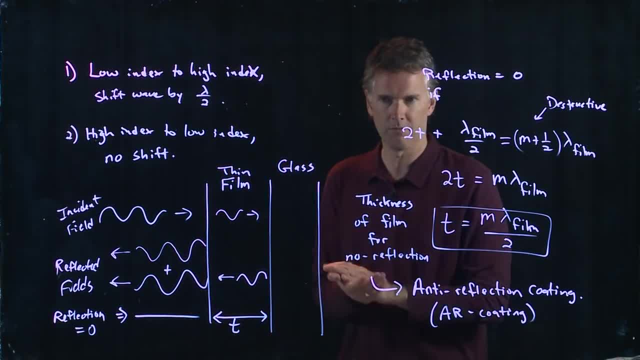 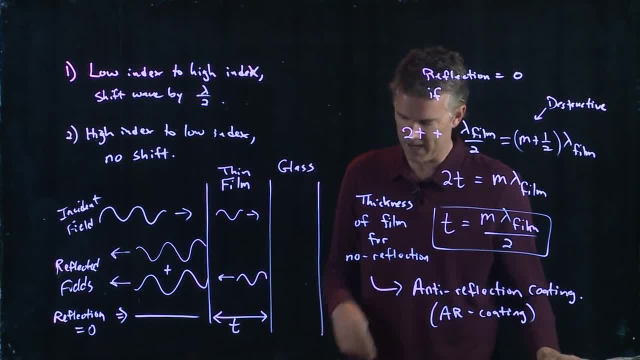